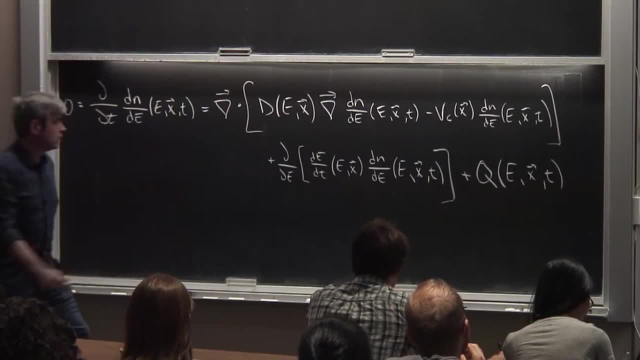 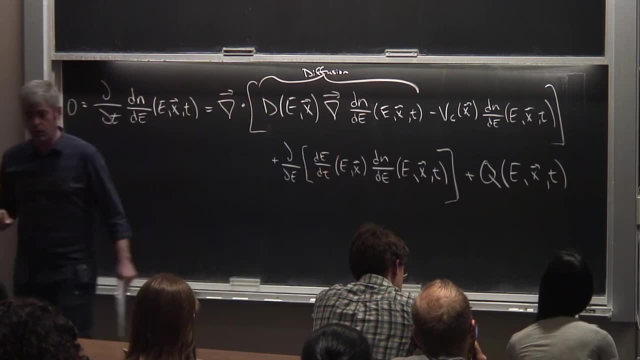 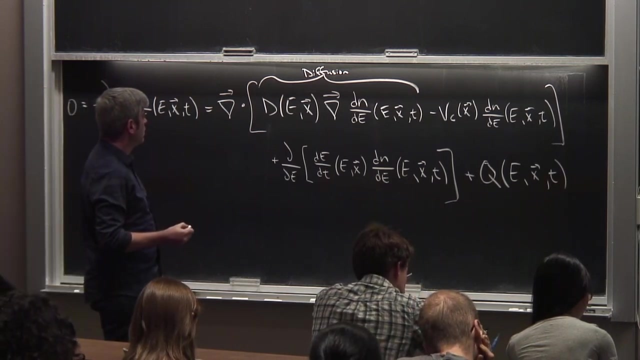 have this term here. What does this term describe? Diffusion In words? what are we talking about when we say diffusion, Diffusion, Okay, So are we taking the gradient of the diffusion term, or does the diffusion term include the gradient operator? 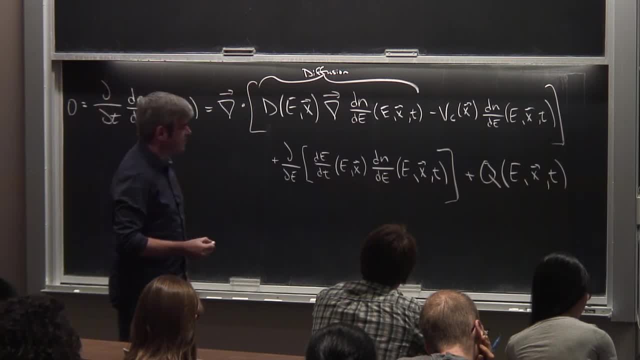 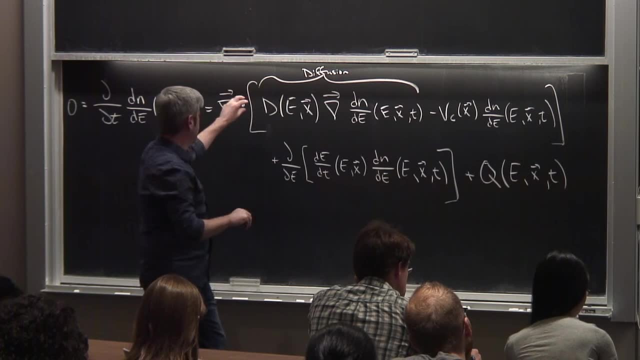 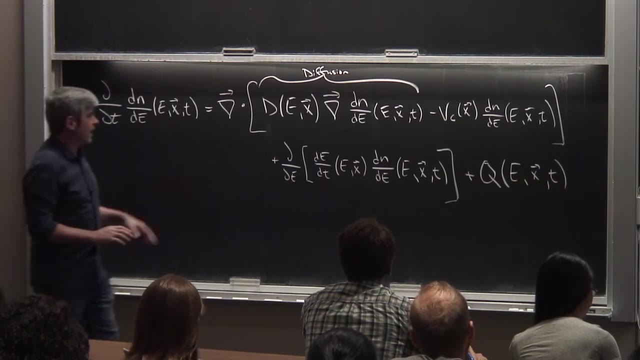 I mean that's a semantic difference. I mean, like, honestly, what I would have done to make this a little bit more clear is write this dot this minus that dot that, And then you could more cleanly separate them. I didn't want to extend this here because of the brackets. 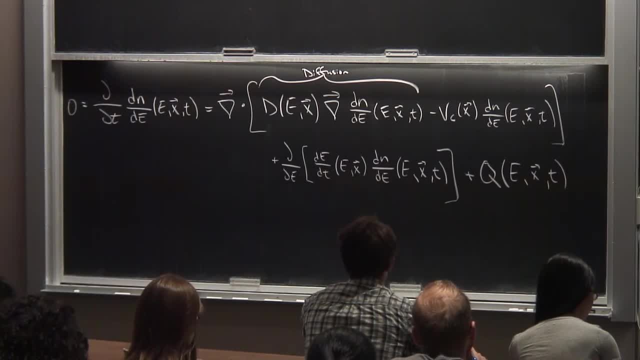 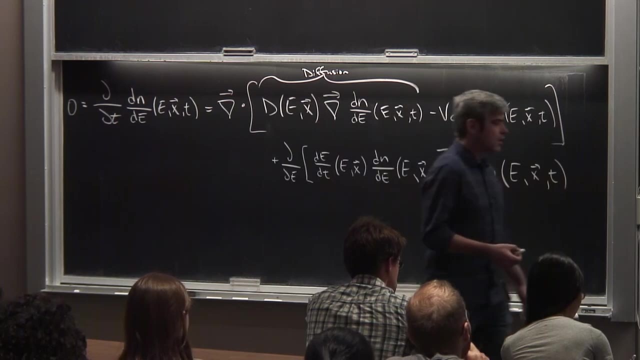 but I think that's all I mean by it. Good, So if you look at the magnetic field in the Milky Way, we have good reasons to think that it's, you know, a few microgauss on average And it has an ordered component. 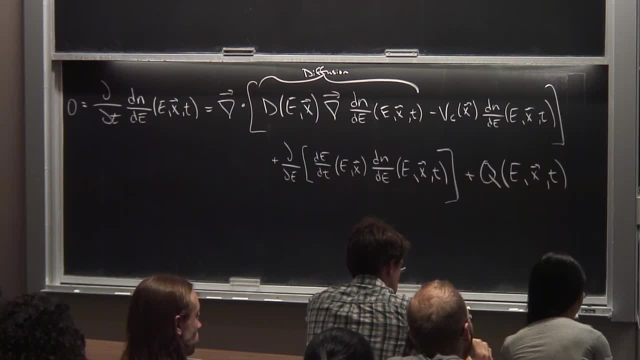 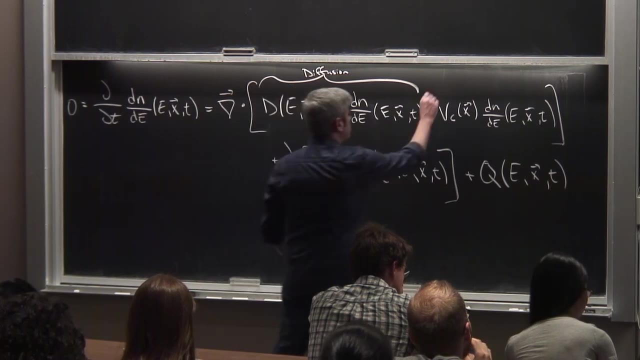 on top of a tangled component, And it's a tangled component that drives diffusion. So you jump from field line to field line, moving in what is effectively a random walk, And you know you can see the. So I'll start with the. 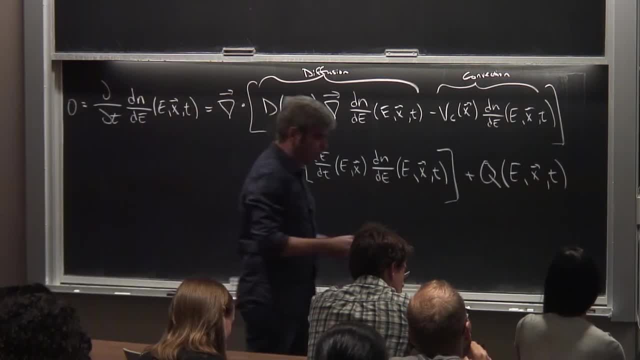 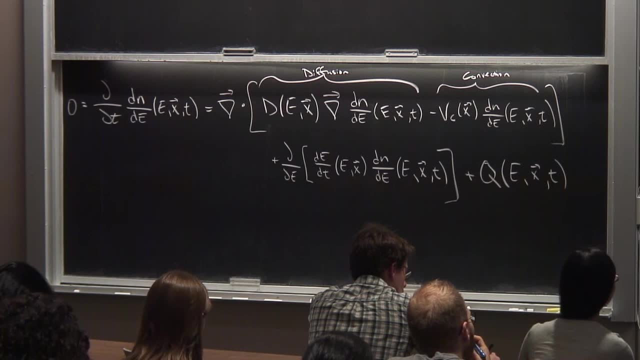 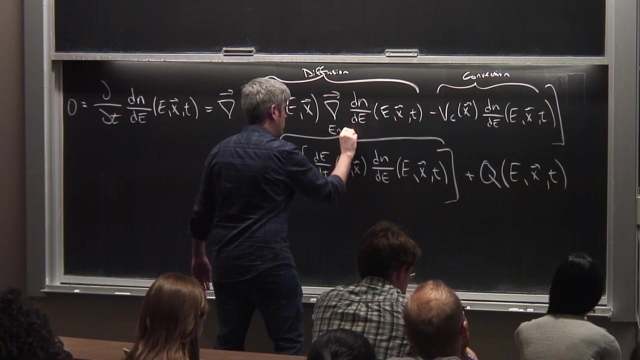 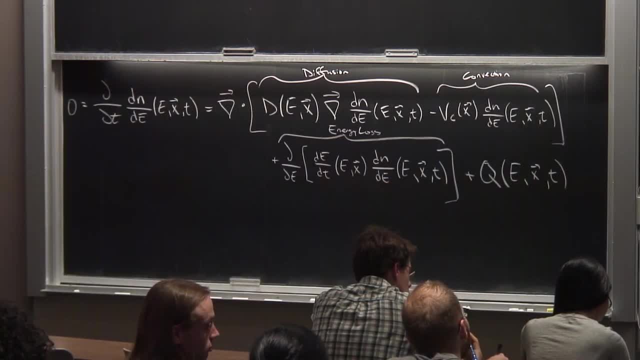 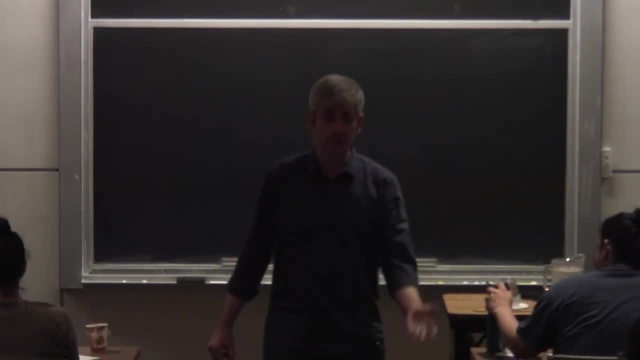 large fractions of the speed of light. The 10 to the minus 3 of the speed of light that the galaxy is rotating at just doesn't matter in that picture. for that reason, If we are rotating at a tenth of the speed of light or something, you would worry about terms like that. 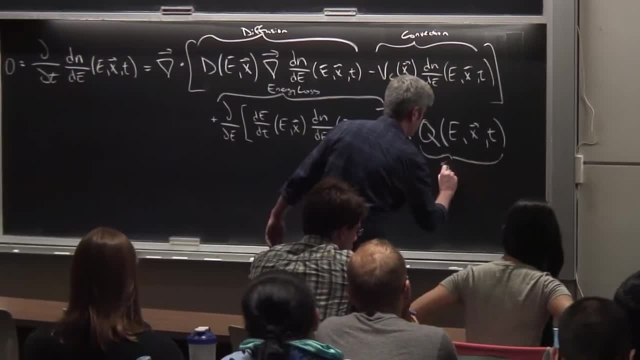 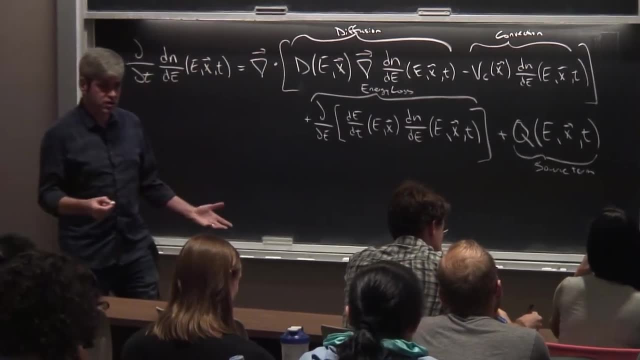 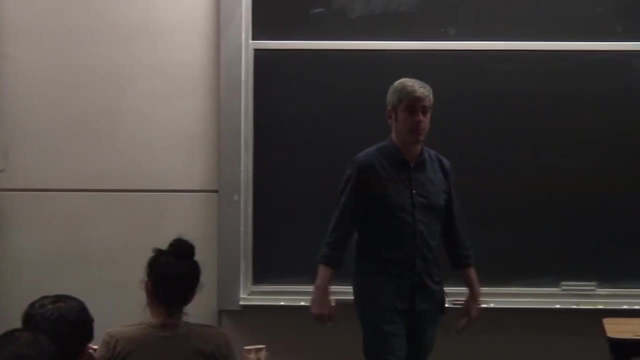 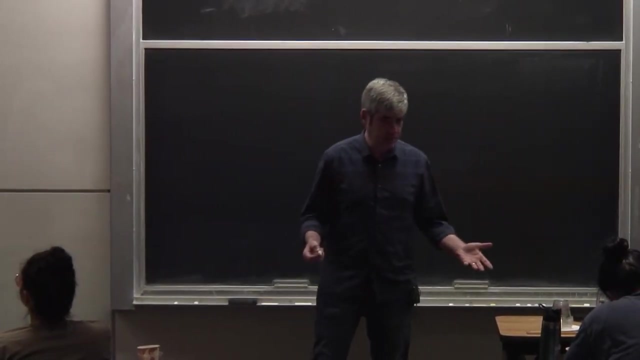 And then this last thing is just what we call the source term, And that encapsulates where all the sources of cosmic rays are and what the spectrum and other temporal properties of that injection rate is. So this source term can include both primary and secondary terms. 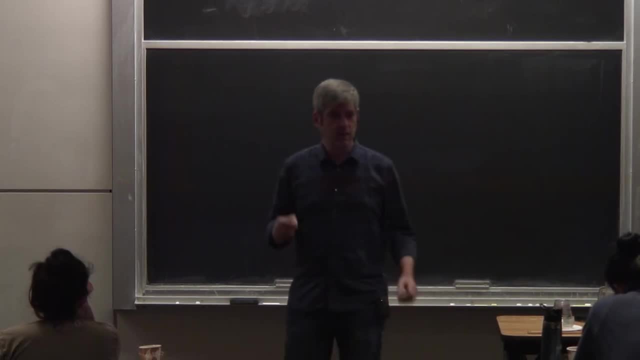 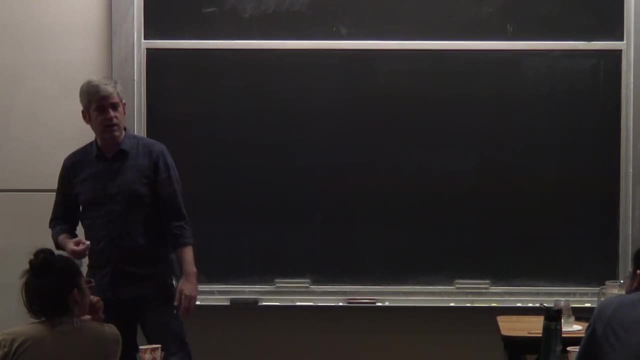 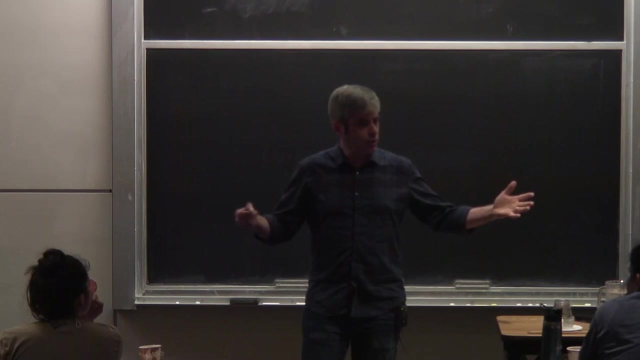 By primary I mean, like a supernova remnant is accelerating cosmic rays, dumping them into the environment, Or dark matter is annihilating, dumping cosmic rays into the environment. I also include secondary terms, where I have in mind the cosmic rays are traveling throughout the Milky Way. 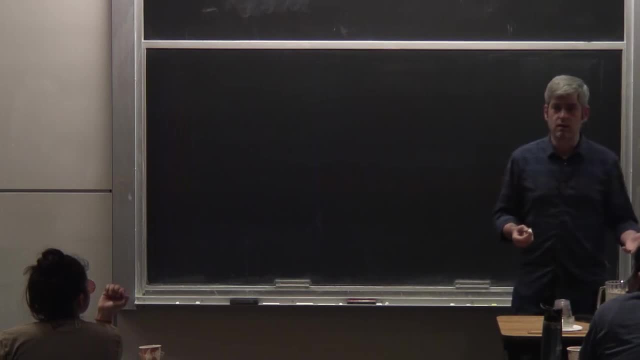 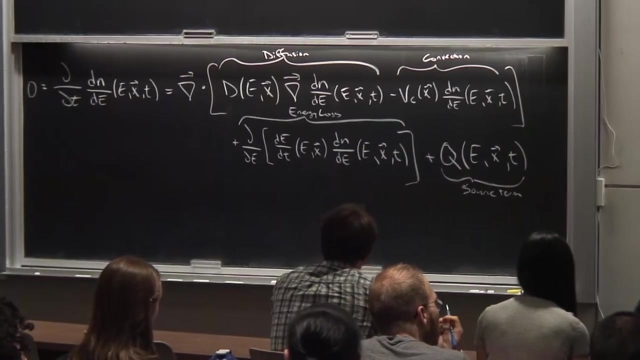 They interact with something, causing new particles to be created in a diffuse sort of way, And that's what I mean by secondary cosmic rays. I'll talk about primary and secondary a lot in the lecture ahead. Sure, I have a general question. Sure, 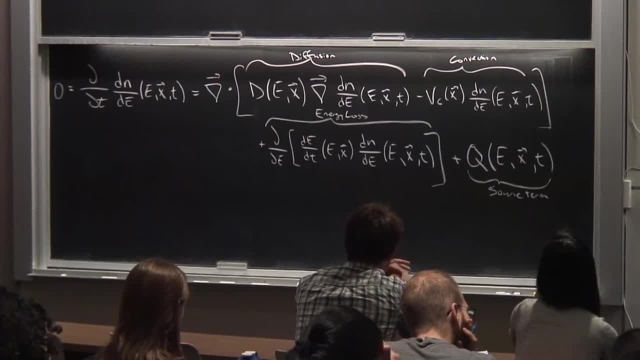 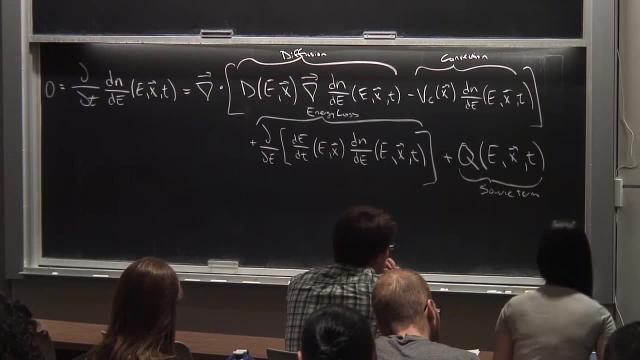 How approachable can dark matter annihilation be in cosmic rays? It seems to me we've predicated on the assumption that we understand where all of the other cosmic rays are coming from, so we can limit them because we know where they come from, by the idea of sources. 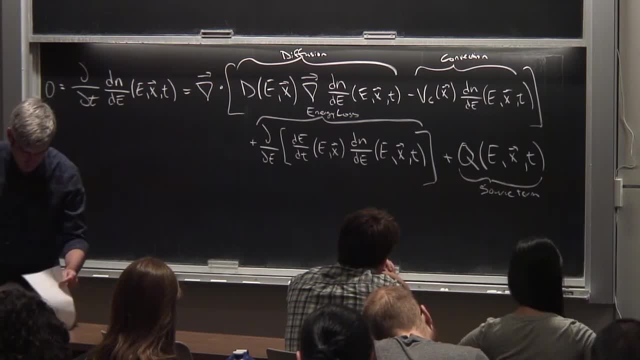 Wasn't there really a question that we knew understood all of the various sources of cosmic rays that well Well so. So instead of answering that question now, I'm going to show you how we constrain some of these parameters, including the source term. 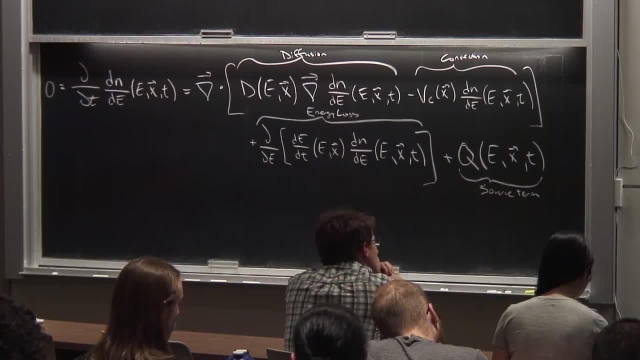 I'm not going to disagree with the sentiment that there are things we don't know about the origin of cosmic rays. We know enough about them. however, through a series of observations to, I would say, make this problem tractable, even if there are going to be some underlying uncertainties in the problem, even when we're done. 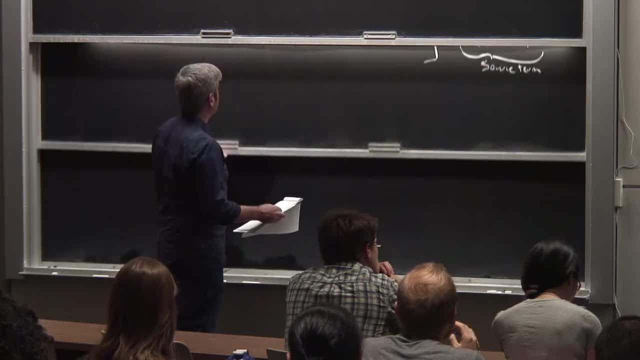 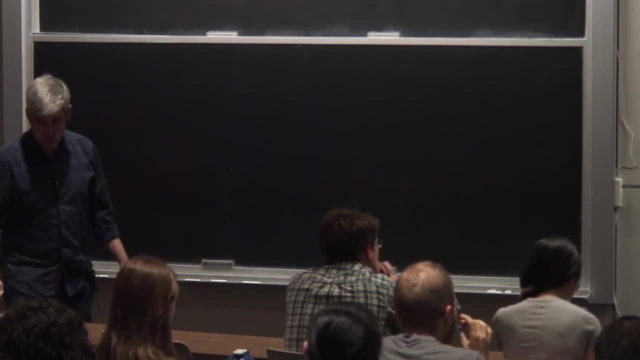 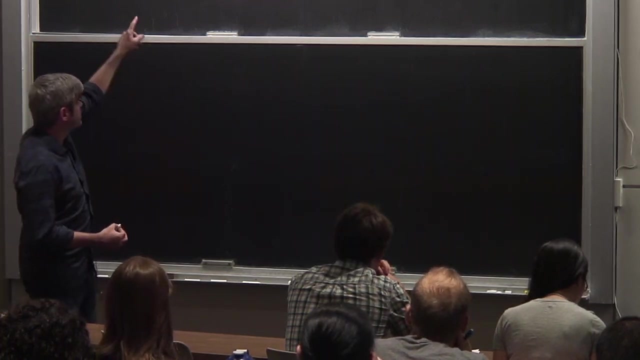 All right. so We have a lot of freedom in this equation that we're going to have to try to constrain. if we're going to make progress, We need to figure out what the size of that diffusion coefficient is, the d of ex and maybe its energy dependence. 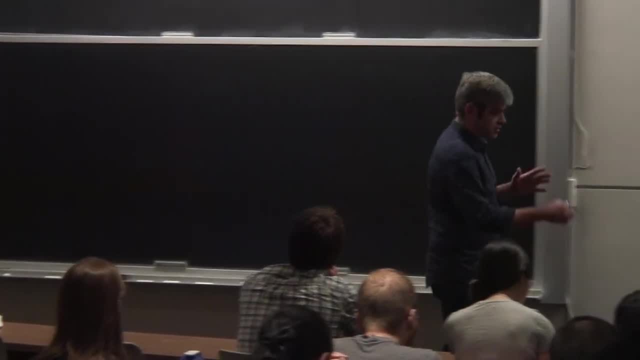 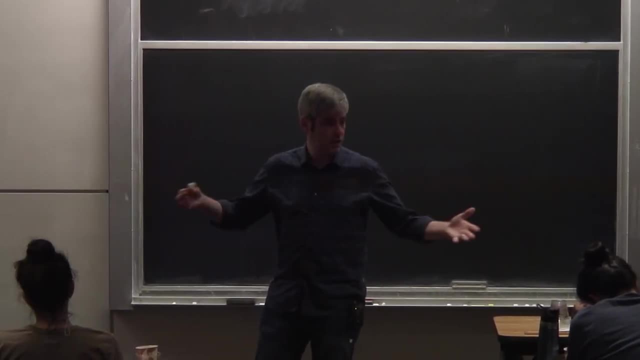 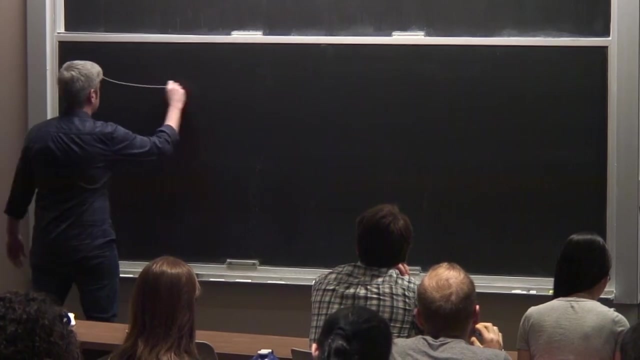 You notice, it's a function of location That effectively gets modeled in modern cosmic ray codes as boundary conditions to the diffusion zone. So we talked about the cylinder that we pretend the Milky Way is described by. I'll just sketch that again. The idea is: 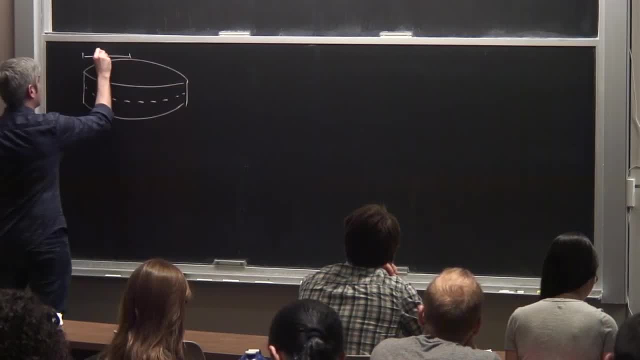 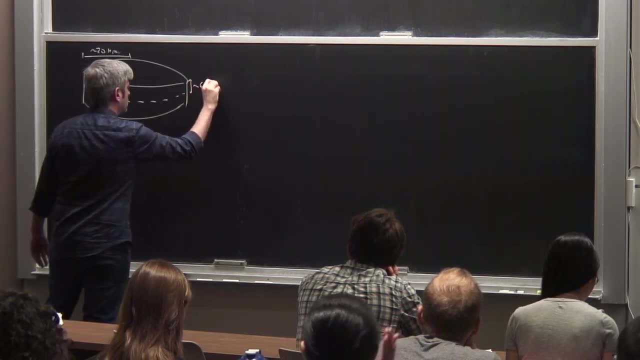 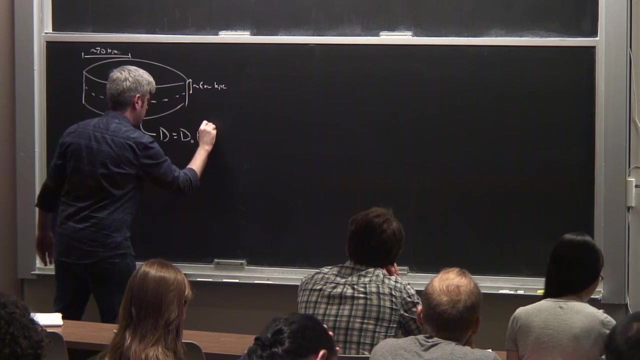 the Milky Way is some sort of cylinder with a radius of like 20 kiloparsecs or so and a half width of a few kiloparsecs, And the idea is that anywhere, anywhere inside that cylinder, the diffusion constant is independent of location. 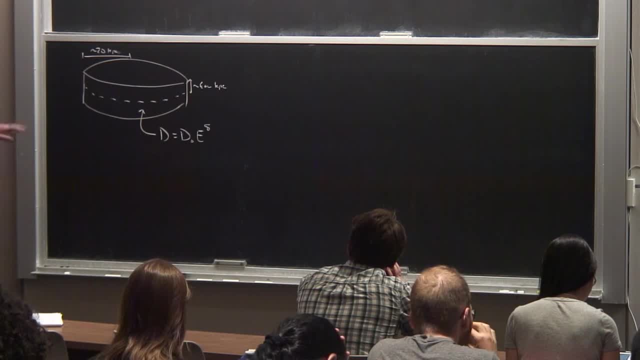 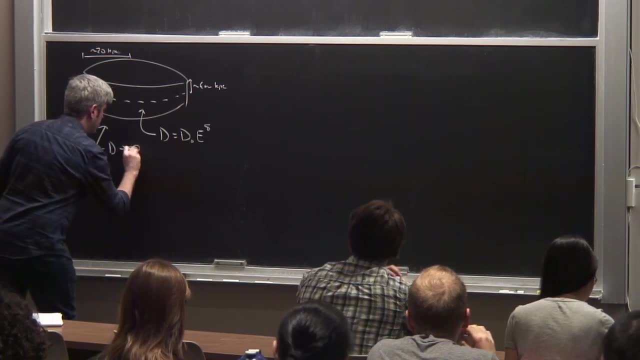 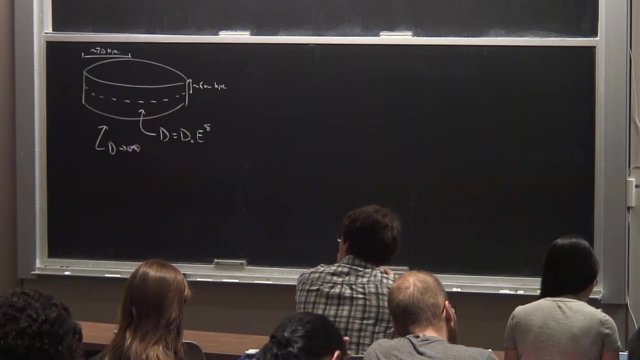 It's just some constant times, some power of energy. That power of energy is usually measured to be about a third, And then, outside of the zone, everywhere the diffusion constant is taken to be infinity. This is another way of calling it: free escape, boundary conditions. 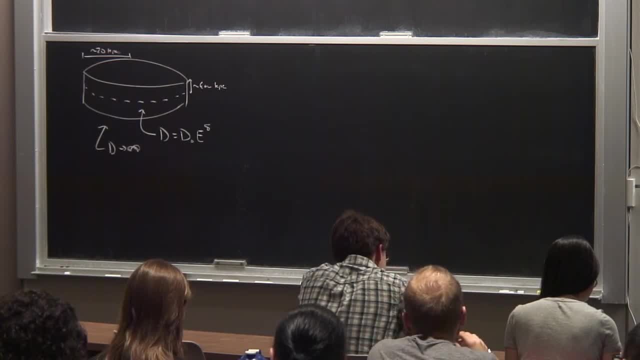 Every time a cosmic ray hits the boundary, it leaves your problem. This is obviously not physically what's going on. What's really going on is the diffusion constant gets steadily larger, perhaps as you move away from the plane. But this is a way to encapsulate that physics in a more tractable parameterization. 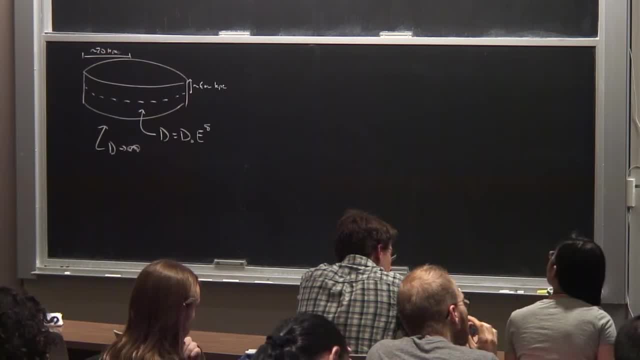 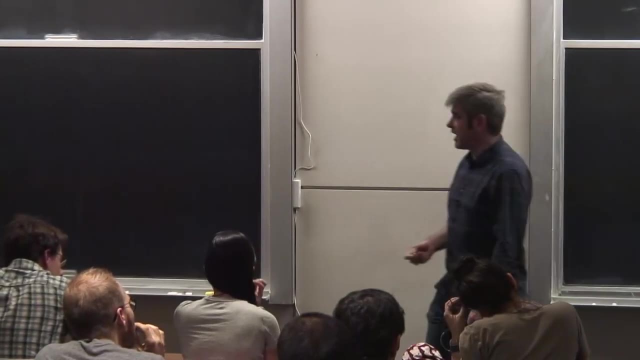 Sorry what The cylinder describes the diffusion coefficient, which has to do with the magnetic fields which, of course, are correlated in some complicated way with baryonic activity. Clearly, the dark matter- halo- is much bigger than this, But the baryonic matter, for example, is not a few kiloparsecs thick. 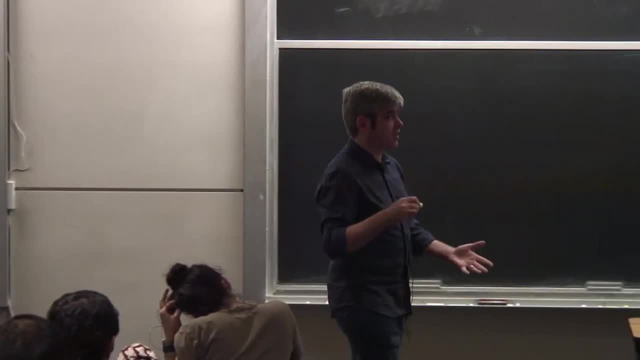 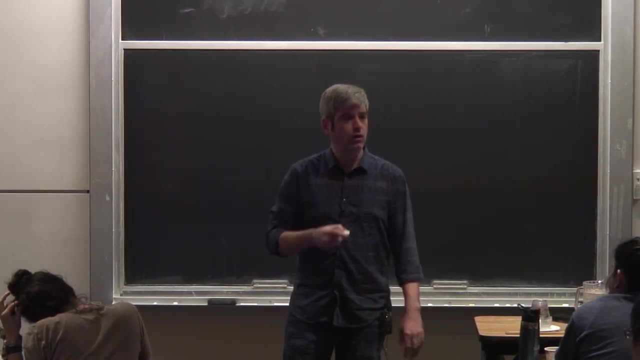 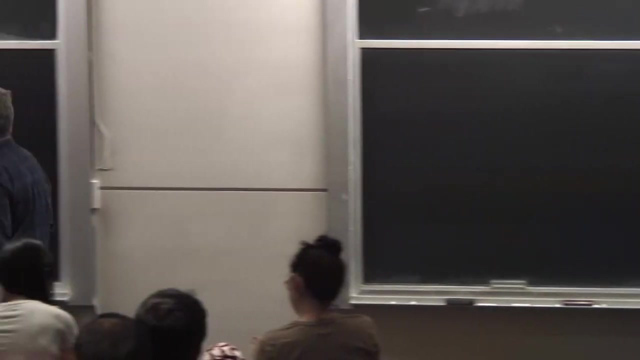 It's a few hundred parsecs thick, So this is much thicker than that. So it seems that the diffusion is confined to a much larger vertical size scale than the distribution of, say, stars or gas or something. Okay, so we've got the diffusion coefficient. 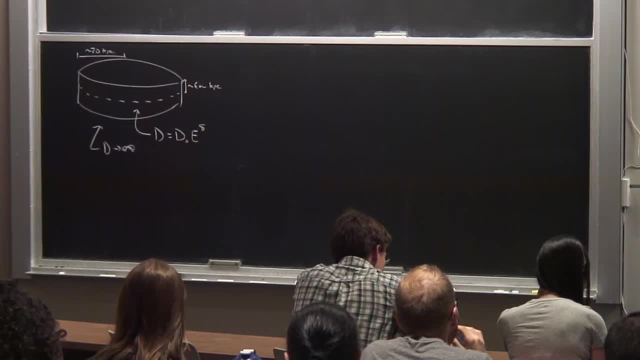 We have the boundary conditions, And then of secondary but still some importance, are things like the convection velocity. I've written down a re-acceleration term, but there are parameters having to do with that, And then you also probably want to put things into your energy loss term. 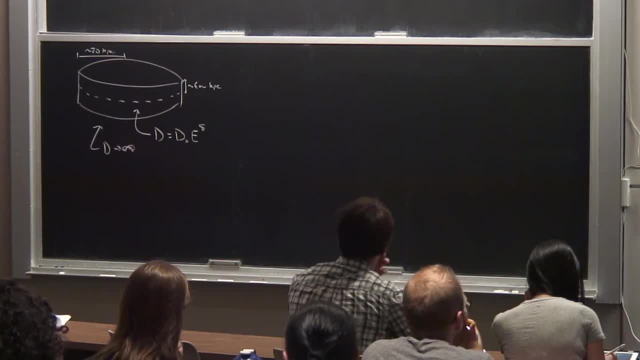 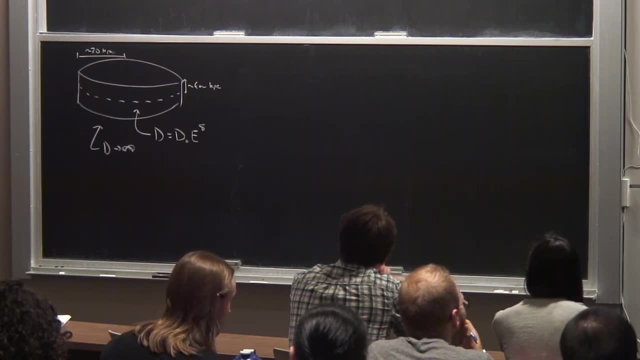 that describe where the gas and radiation and stuff your particles are scattering off of are. And then, finally, you need to define the source term. Maybe you assume that supernovae are receiving energy and are responsible, in which case you would put some sort of source term. 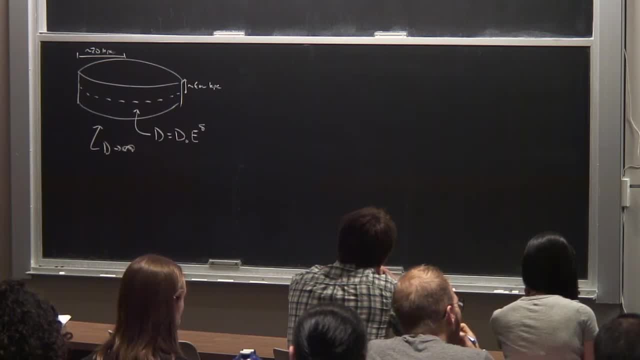 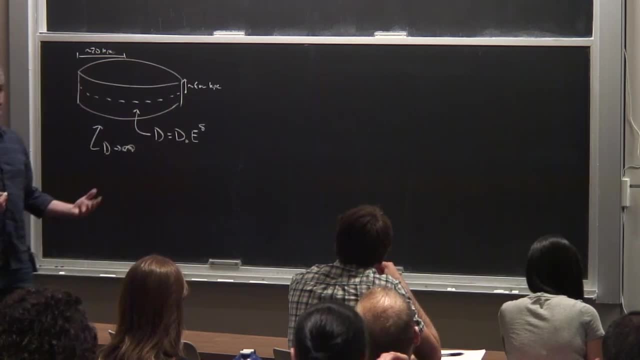 that scales with the stellar distribution or the distribution of massive stars. Maybe you're going to assume that's in steady state or so something like that, Things like this. You have to assume also things about the injected spectrum of those particles, And that's a lot of free parameters. 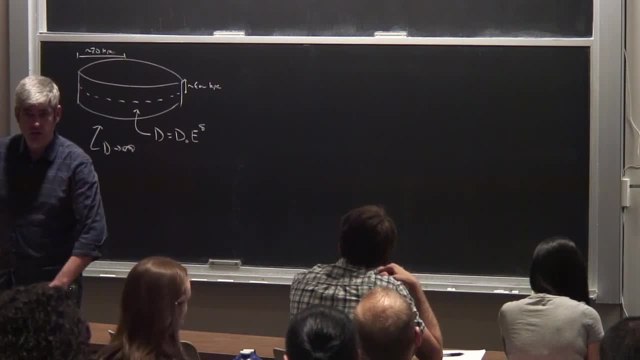 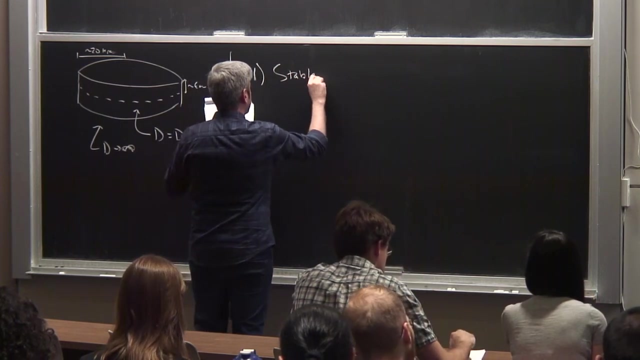 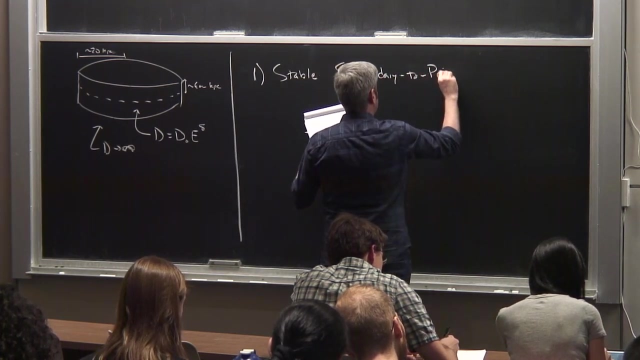 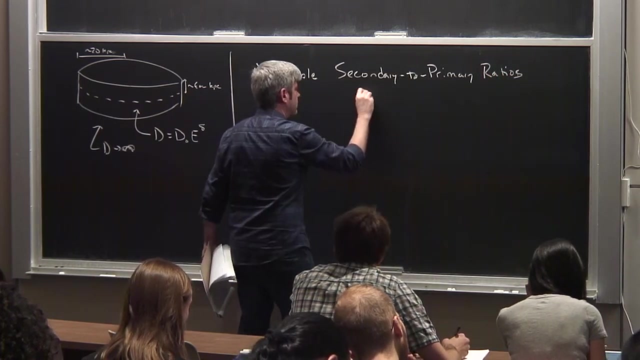 But fortunately we have a lot of data to constrain those various parameters with. All right. so first we're going to start with considering what we call stable secondary to primary ratios. So here I have in mind, for example, boron to carbon. 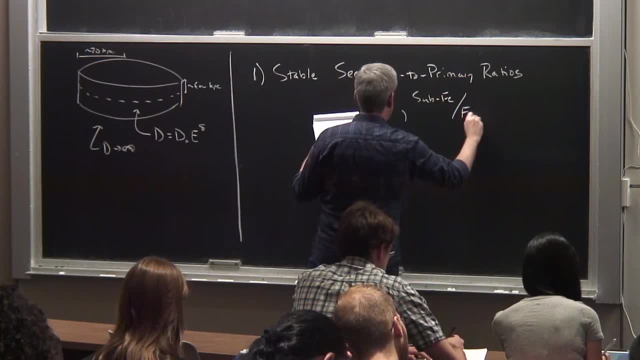 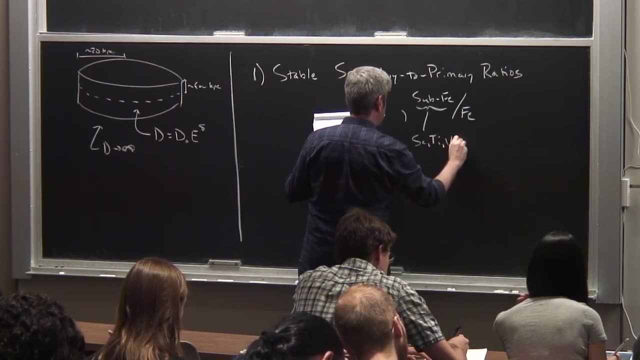 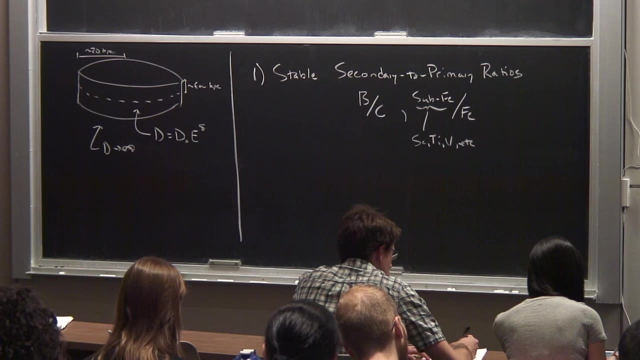 What's commonly called sub-iron to iron, And by sub-iron I have things in mind like titanium and stuff like this. So let's say, I put an experiment up in space or on a balloon or something And I measure the spectrum of boron. 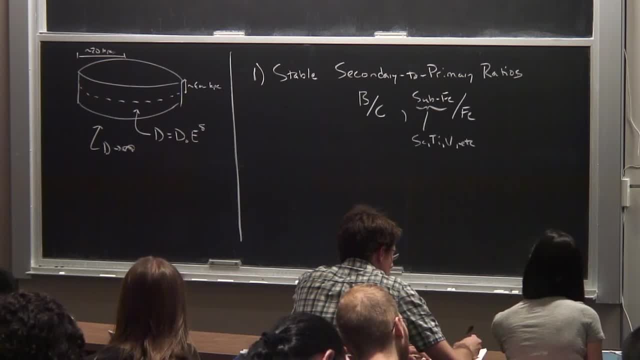 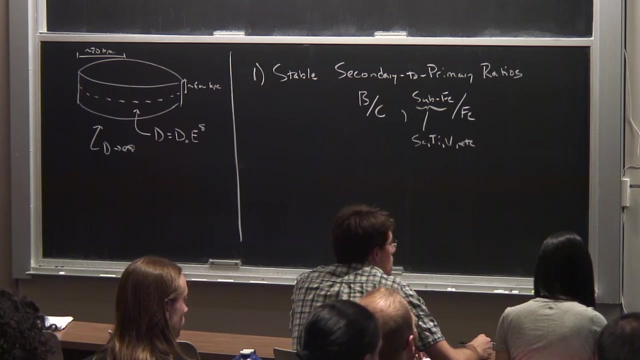 and I measure the spectrum of carbon. What does that combination of information allow us to say about carbon? Let's talk about how cosmic rays are produced and transported through the Milky Way. Where do we think the boron and carbon come from? Supernovae is stars. Which of those do you expect they would make more of In a typical star? What's a typical star? made of Hydrogen and helium, But that stuff doesn't make for very interesting cosmic rays. So, for the purposes of this, what are the other big quantities of stuff out there in stars? C and O, basically Carbon, nitrogen, oxygen and then iron in the really massive stars. That's the stuff you get lots of. You don't find any substantial amounts of boron, So supernova remnants make you a lot of carbon. 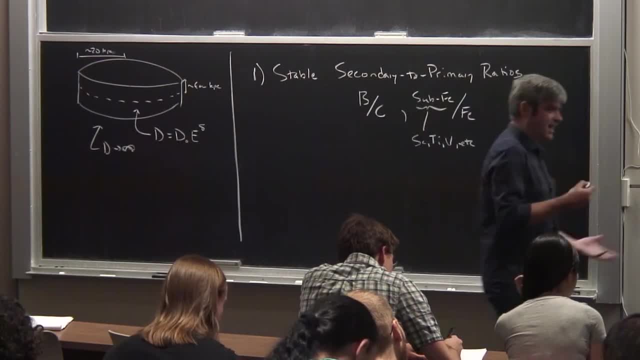 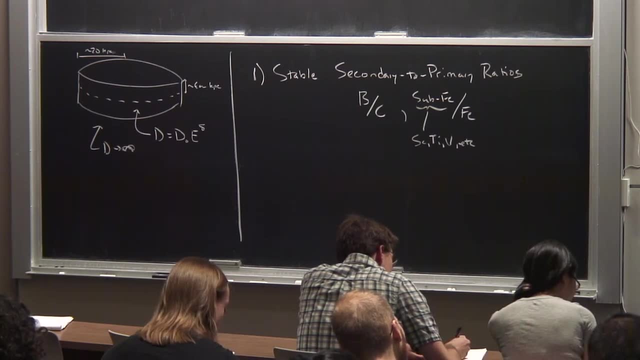 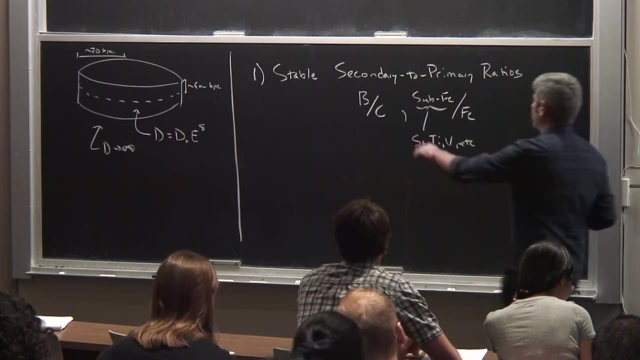 and almost no boron. But the boron to carbon ratio is not that small. So where's the boron we observe in the cosmic ray spectrum actually coming from? It's not so to distinguish. there's a hint here. I've called this the secondary to primary ratios. 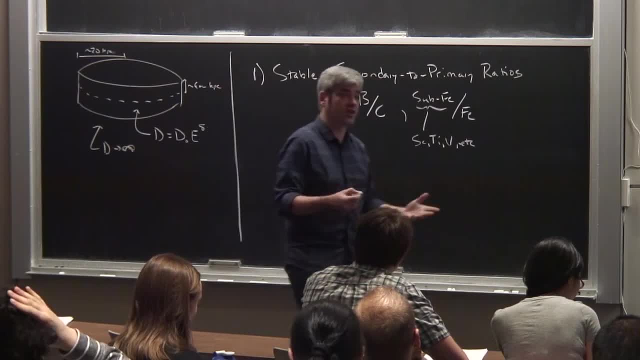 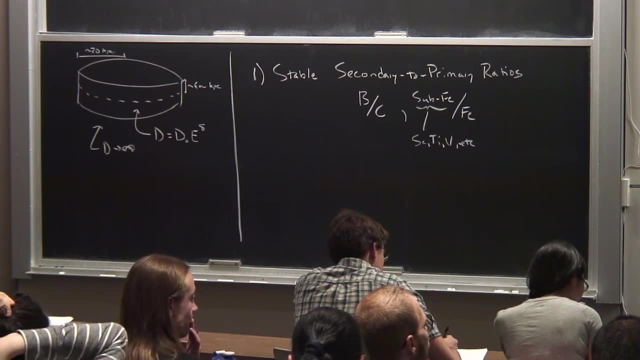 Obviously the carbon is my primary And I said before, secondary is something that's produced in cosmic ray propagation. So you're a carbon nucleus flying around near the speed of light through the Milky Way. You hit some gas and you break apart, creating some boron. 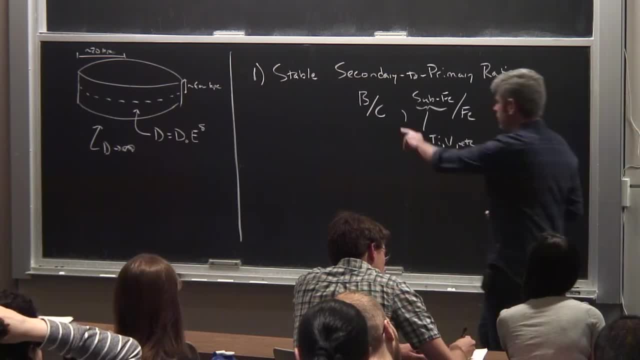 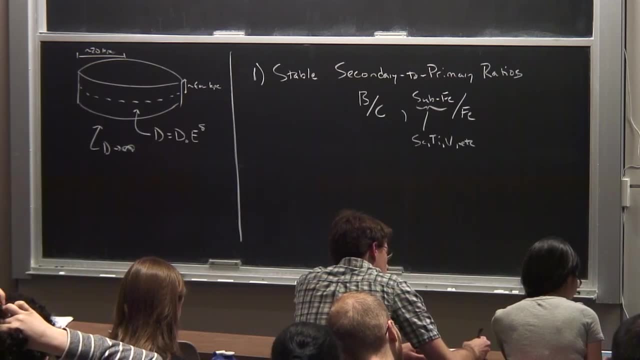 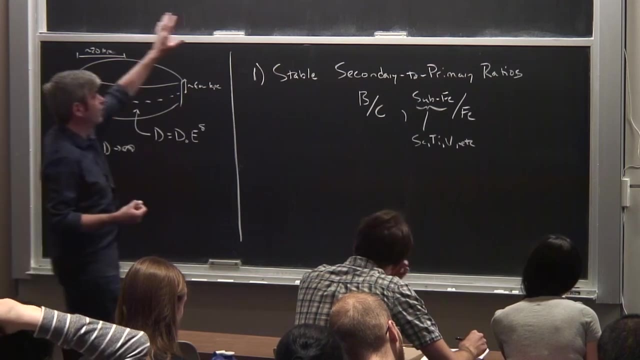 So by measuring this ratio as a function of energy, you're learning things about how much material a typical cosmic ray passes through in the course of its life. Of course it's a statistical thing, But you can take a given set of cosmic ray parameters. 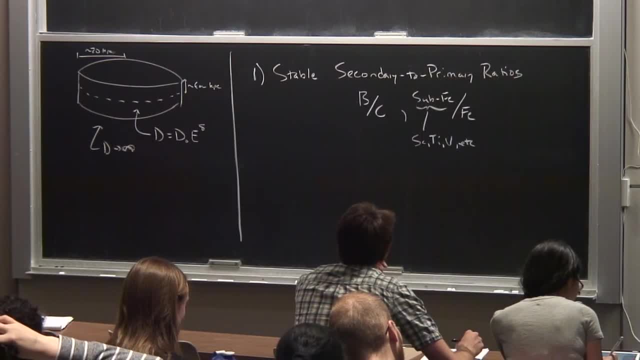 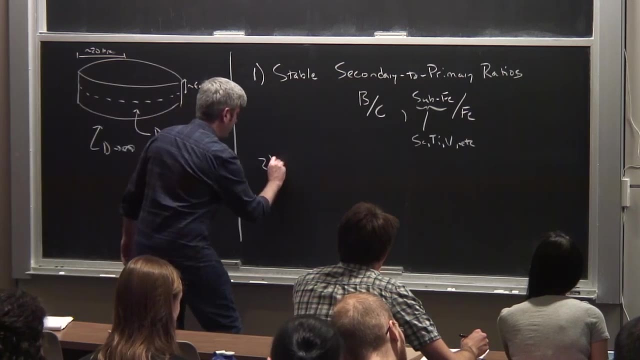 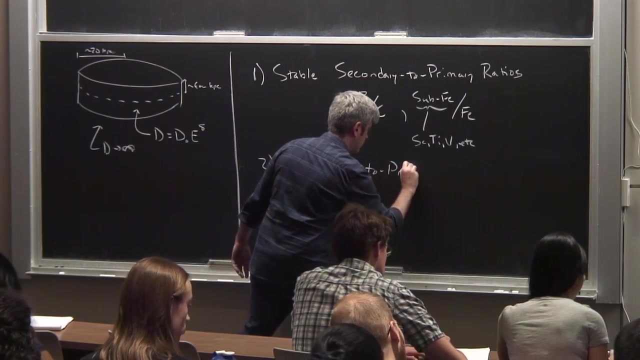 try different combinations and see which agree with the boron to carbon ratio as a function of energy, And you can do it independently for sub-iron to iron and other secondary to primary ratios. So you can probably guess what the next thing I'm going to write is. 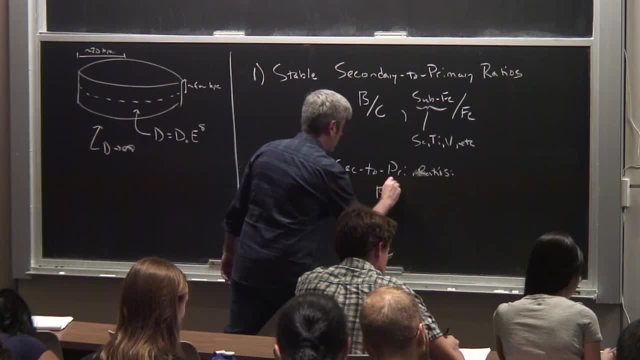 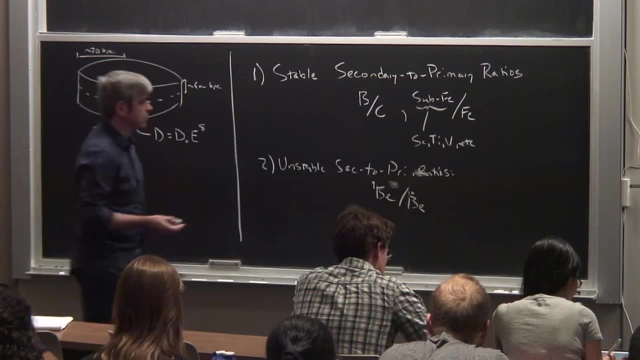 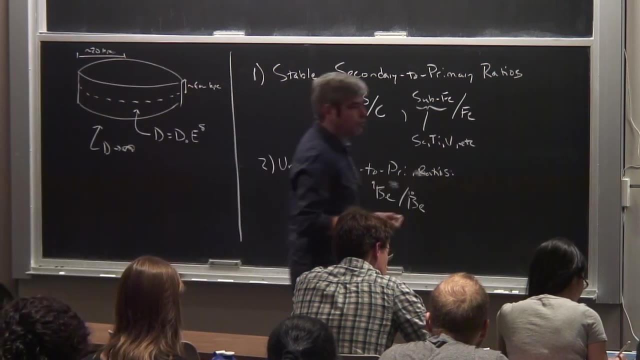 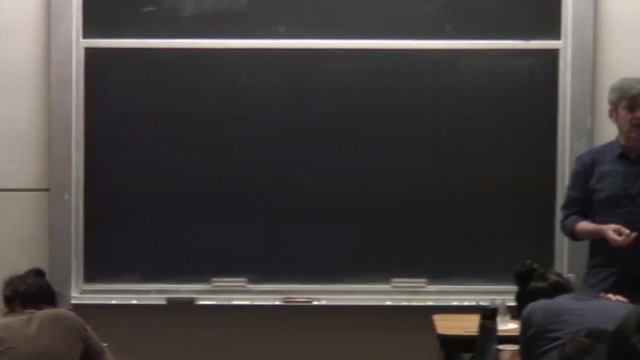 And here I have the bryllium-9 to bryllium-10 ratio as maybe the single most useful example. So why would looking at an unstable primary to secondary ratio provide different information, or what information would it provide in contrast to the stable example? Okay, good, It depends a little bit on the time scale we're talking about, right? So in this particular case, bryllium-10 has a lifetime of about 1.3 mega-year, So that's not all that local. 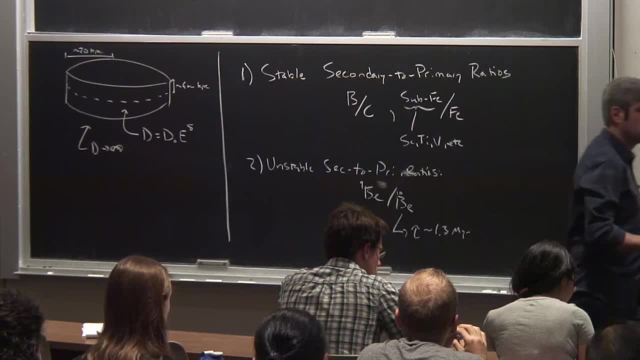 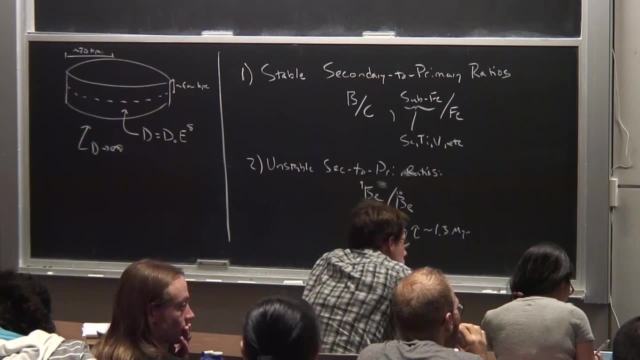 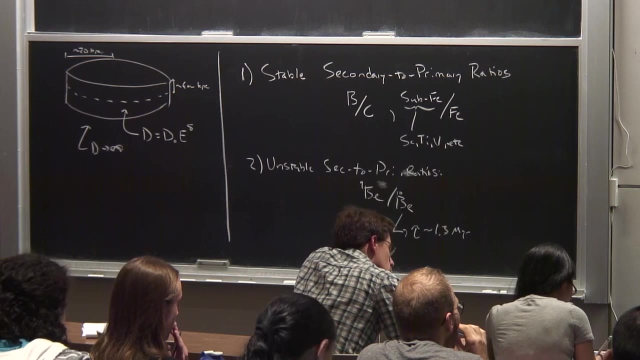 We'll do a back-of-the-envelope estimate of that in a second. So by measuring boron to carbon, a stable secondary to primary, you're inferring how much material cosmic rays propagate through. What are you measuring here, with an unstable secondary to primary ratio? 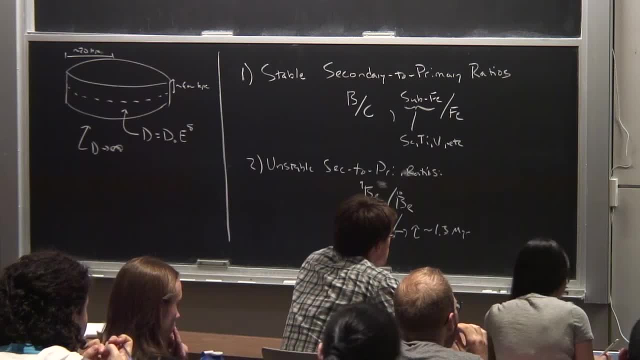 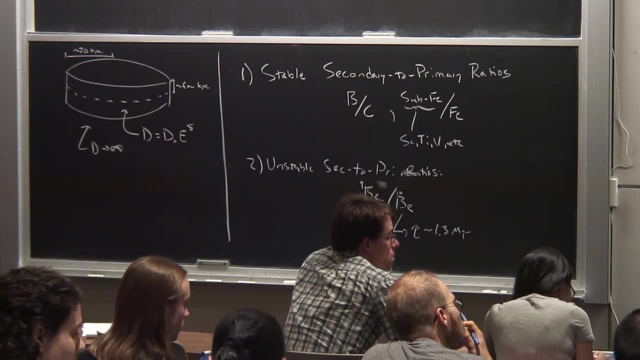 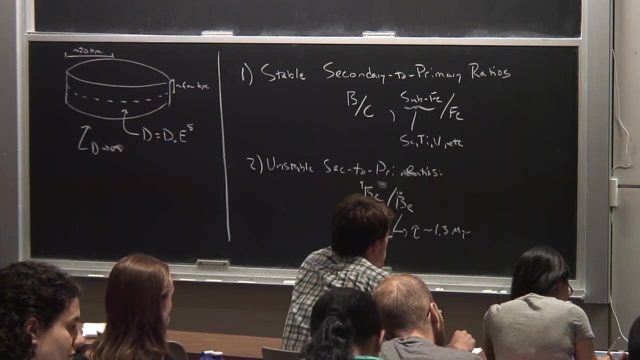 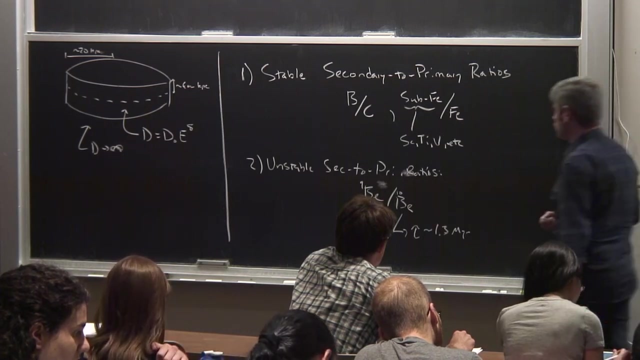 Yeah, good, It's approximately right. I'm going to translate it to a slightly different notion, but it basically tells you how long particles have been traveling through the halo before they escape, before they reach us. So let's just draw a cartoon. 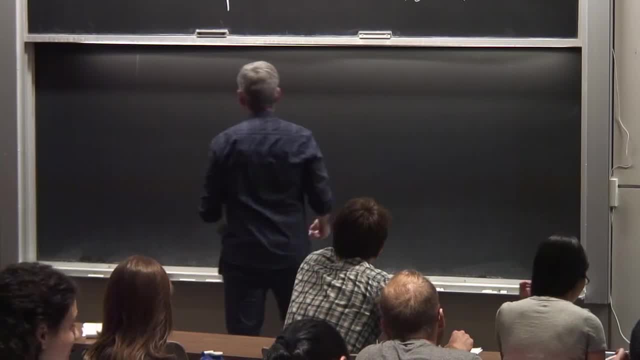 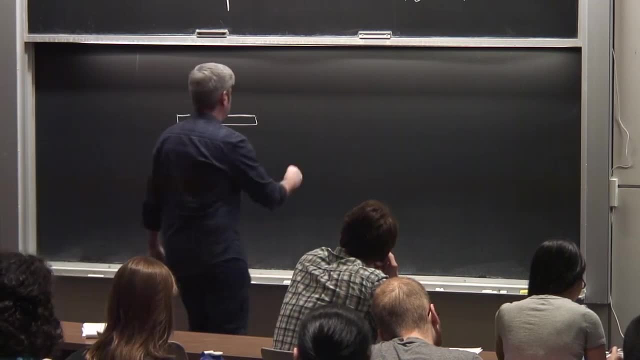 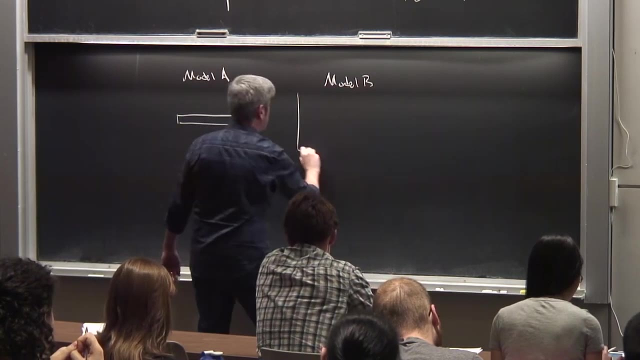 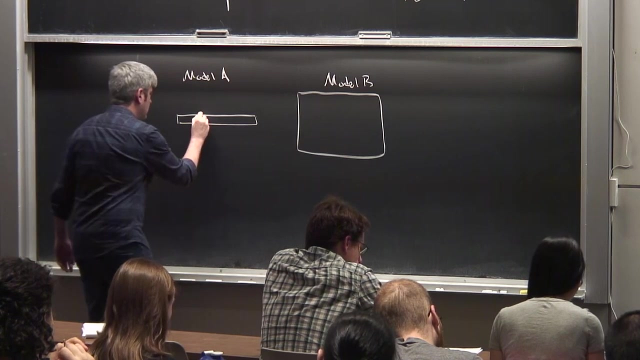 to kind of understand what that might look like. So let's say I have two models. One is this: I'm looking edge-on and the galaxy is really thin. Model A: Model B: the diffusion zone is really big and fat. Okay. 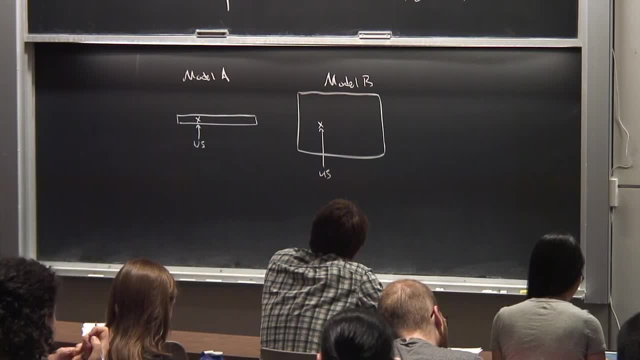 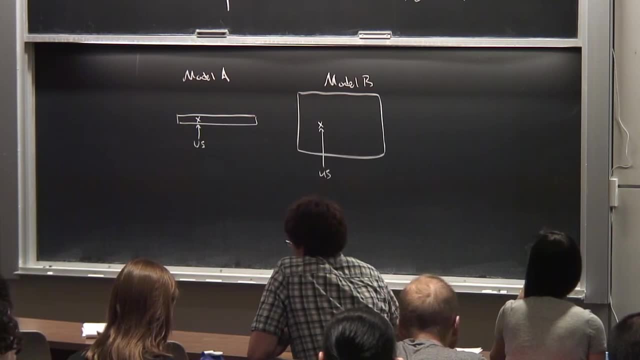 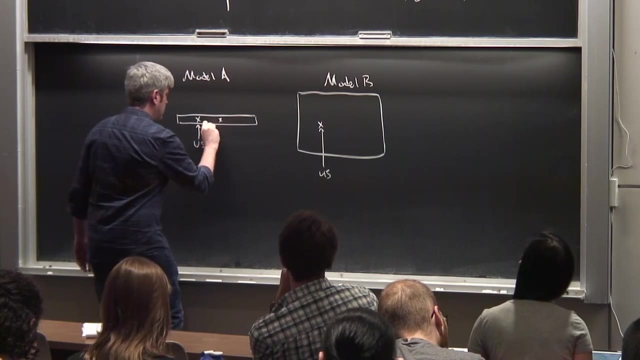 I'm putting us here And now. I have a primary to secondary ratio that's stable, like boron to carbon, and that gives me an idea of how much stuff you pass through. okay, So maybe I put a source here, an average source, okay. 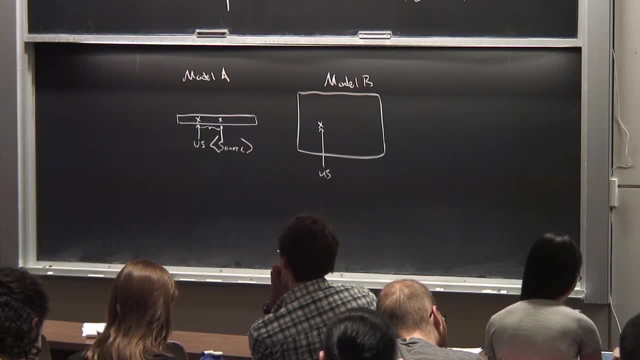 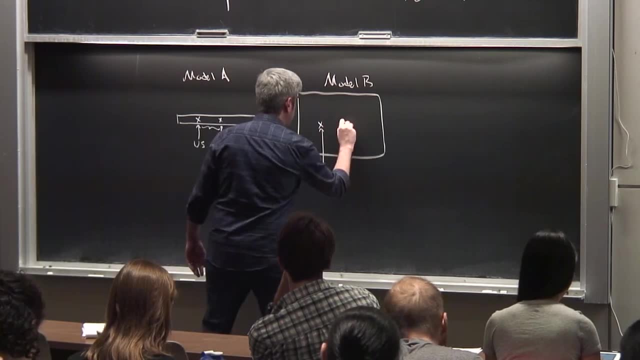 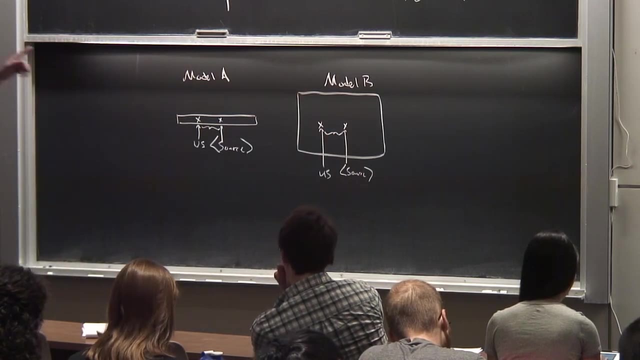 there, because I have some idea of how much stuff was propagated through in route, And that would be true in this case. You'd have the same sort of distance here. This is the average source or something kind of analogous to that. But now I measure the beryllium ratio. 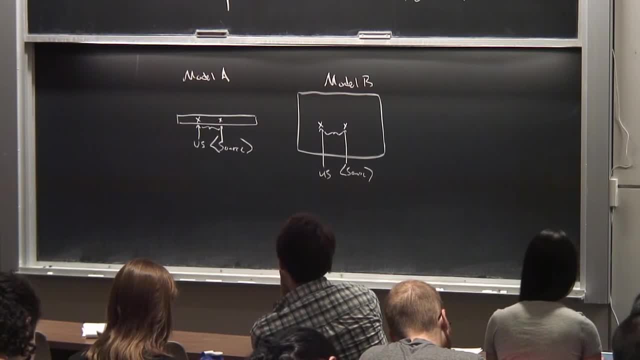 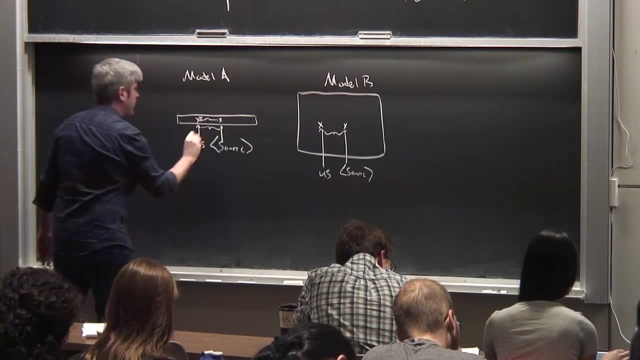 Okay, And this tells me how long these particles have traveled. If we're in the thin model, this thing basically has to random walk straight to me. There's no other way for it to get from me, from it to me, Because if you hit this boundary, 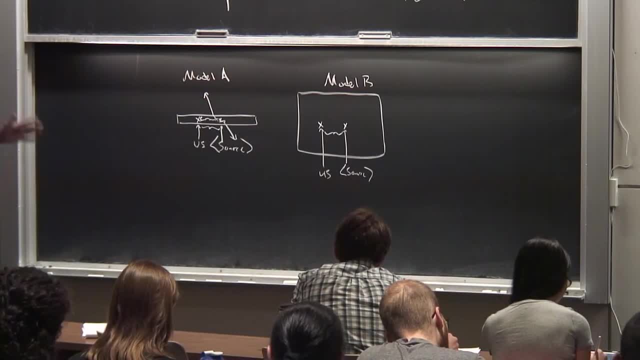 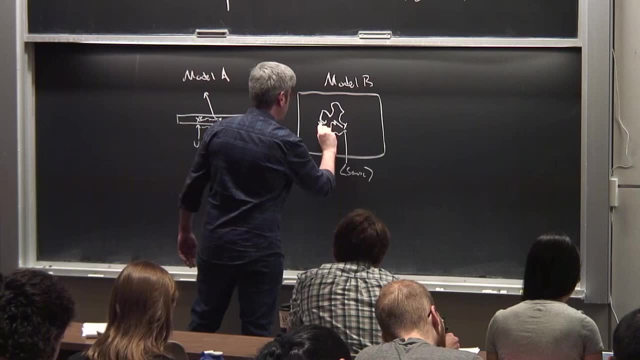 you free escape, So it more or less had to travel in a straight line. In this case, there are a lot of routes available. Random walks will tend to give you complicated trajectories, right. So in this case, even though the diffusion coefficient 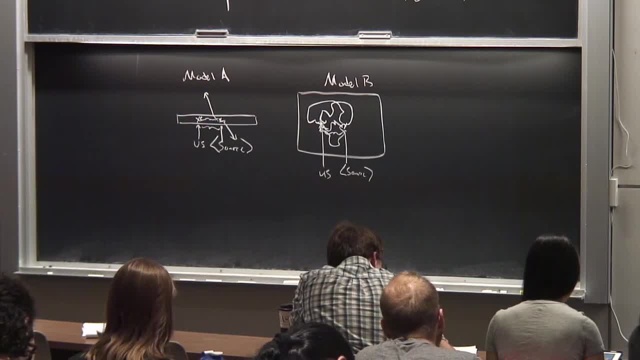 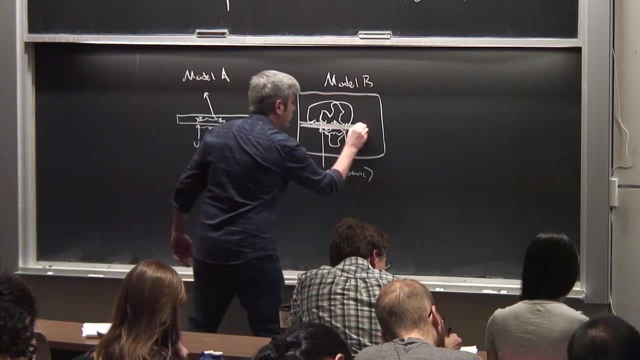 is set to the same value, you wind up with very different lengths of time and very different amounts of material you propagate through. But most of the material we know is distributed in a thin strip that we call the galactic disk. So by measuring this time, 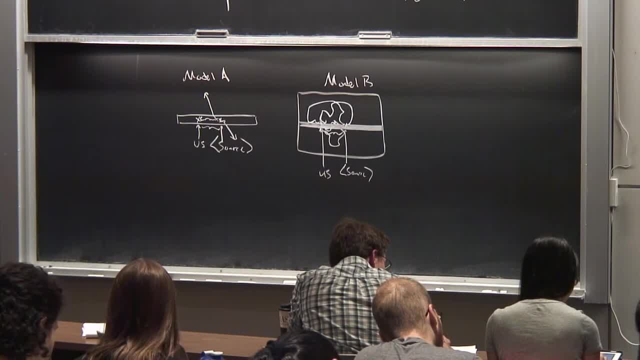 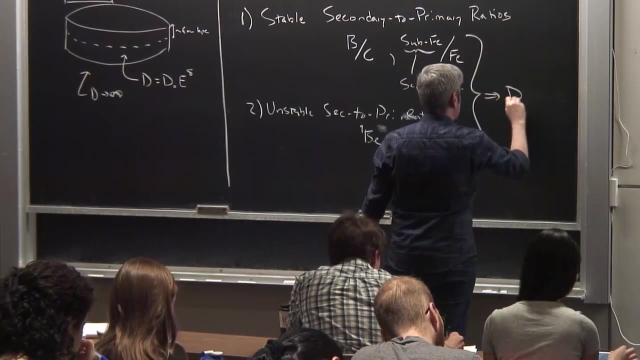 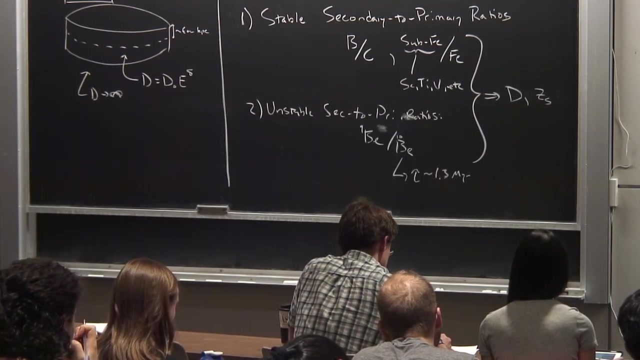 through the unstable ratios and simultaneously measuring the material traverse through with the stable ratios. you can separate these two things and approximately use this information to get information about both d and the scale height of the disk of the diffusion zone. These are approximately the two things. 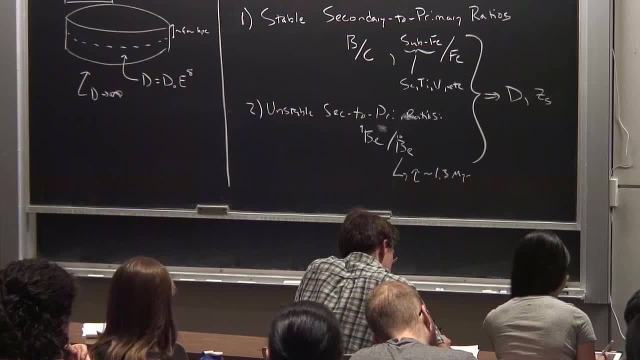 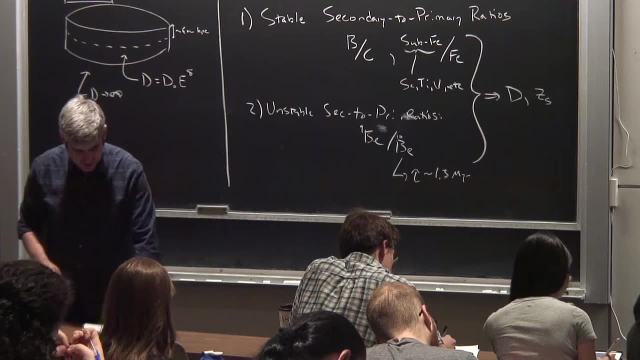 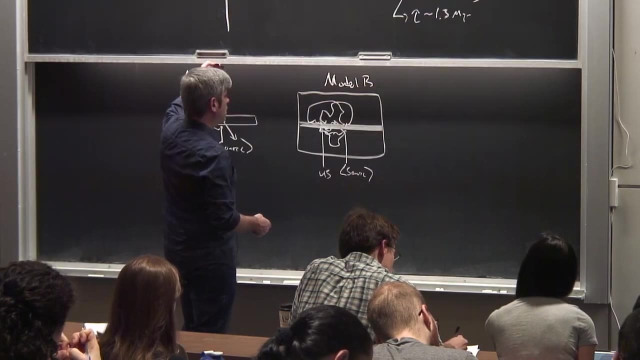 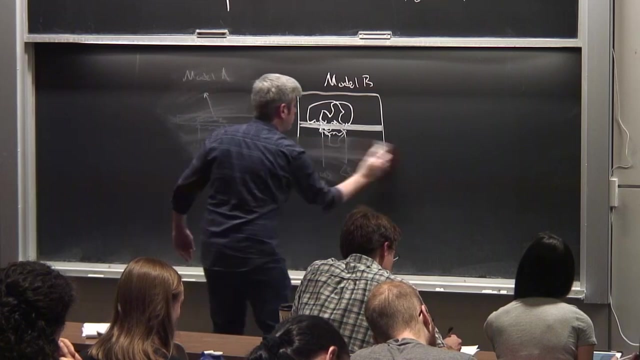 you extract from this information. There are a lot of details I'm sweeping under the rug, but this is a reasonable cartoon of how this works. Yeah, a few kiloparsecs, That's right. So if you do a big global fit, you will find with modern AMS and other data. you will find roughly the following answer, And this is for energies above a few GeV, And the best fit scale heights are right around 4 kiloparsecs And that's a convection velocity. and it's generally in the ballpark of a few tens of kilometers per second, which only matters at very low energy. So we can for the most part treat that as a pretty unimportant factor. That's the picture that's emerged from modern cosmic ray observations. I will mention just in passing that none of the models of the type I'm describing really provide a statistically good fit to all the data anymore. This is a new fact in the AMS age, Back before AMS, when we were relying on other experiments. 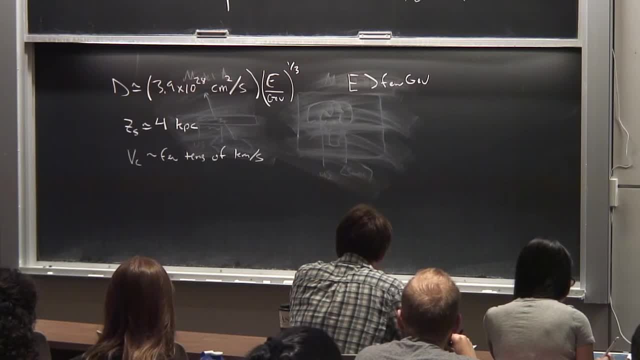 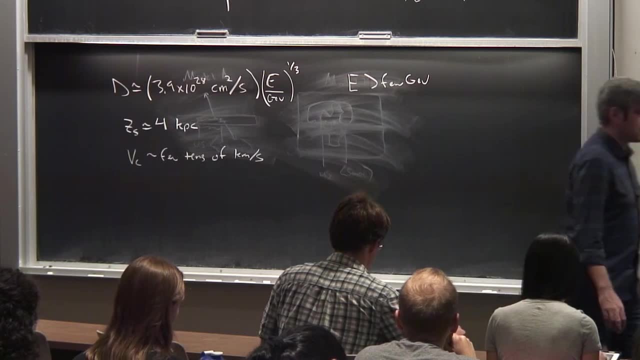 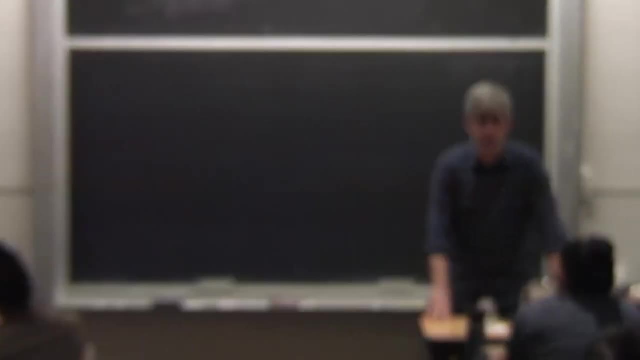 with much larger error bars, you could get perfectly reasonable fits. The error bars provided by AMS are incredibly small and, as a result, there are no particularly good fits anymore. What should I think of this? What is this telling me about the galaxy or the problem at hand? Something we don't understand, or maybe something that's not encapsulated in the model. I described this model yesterday as being a spherical cow, and that's really all it is. There's no reason to think the galaxy's diffusion zone looks anything like that. 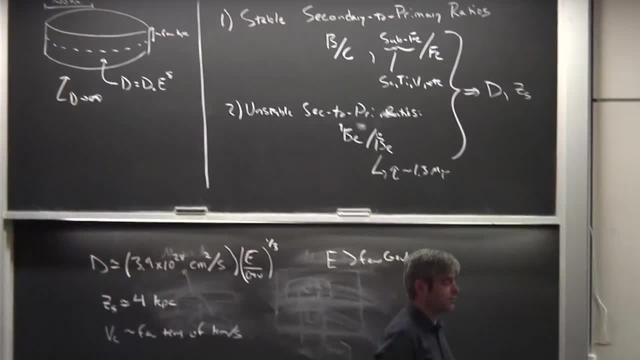 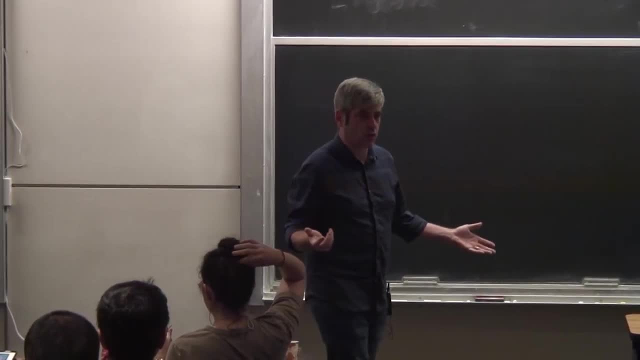 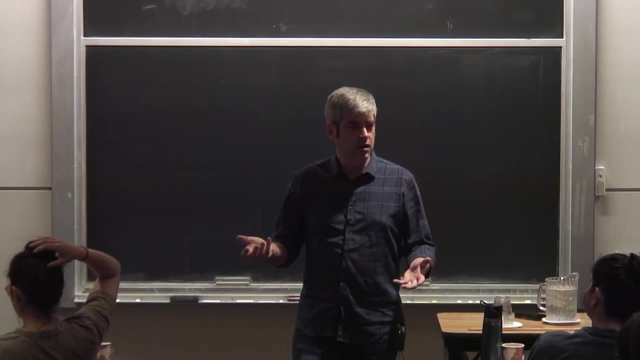 I'm quite confident that if you measured the diffusion constant in, say, a spiral arm and out of a spiral arm, you'd get different numbers. We pretend that's not true. So there's a bunch of averaging going on here that is necessary because of our ignorance. 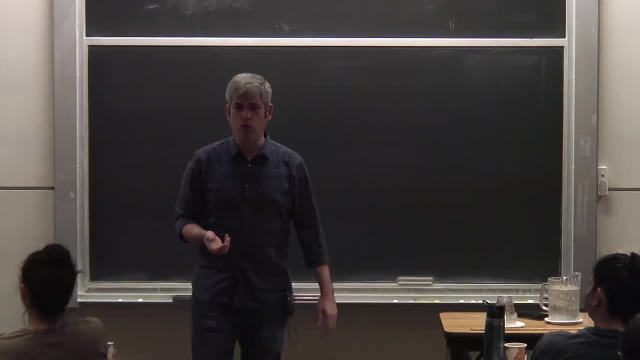 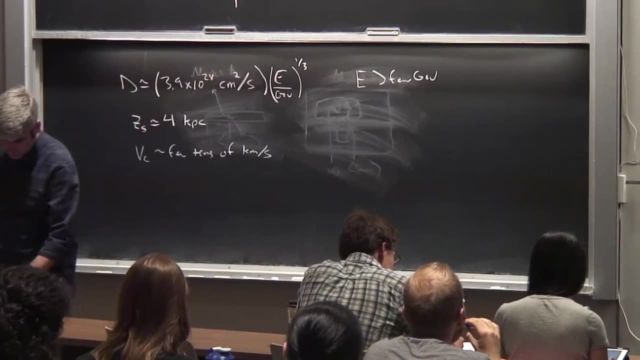 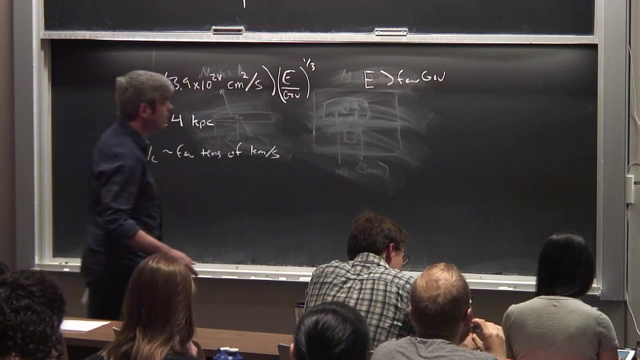 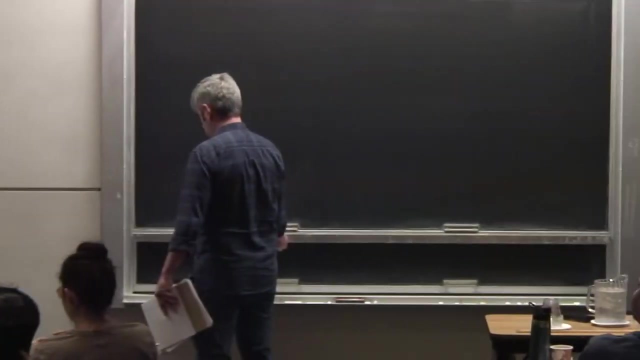 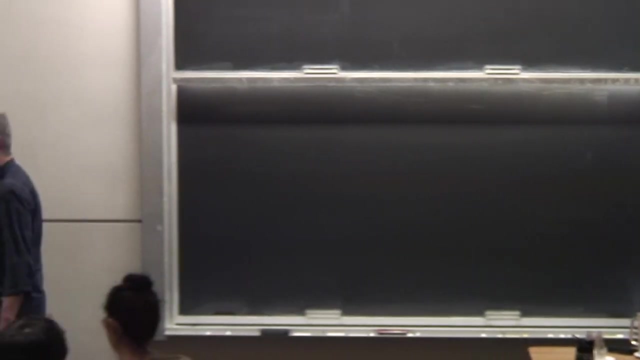 but we shouldn't be that surprised when you measure something at three or four sig figs and it doesn't line up perfectly. We're trying to do weather here, you know. Okay, Yeah, Sure, Well, so I understand where you're going with this. 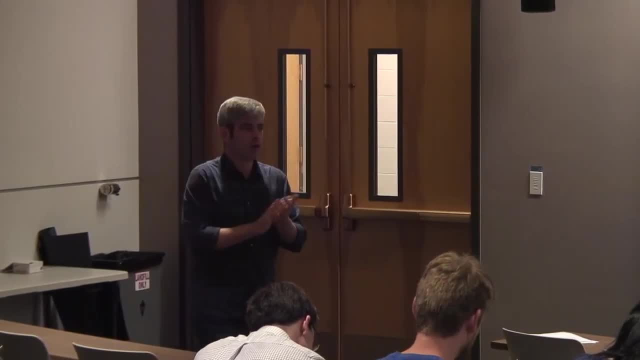 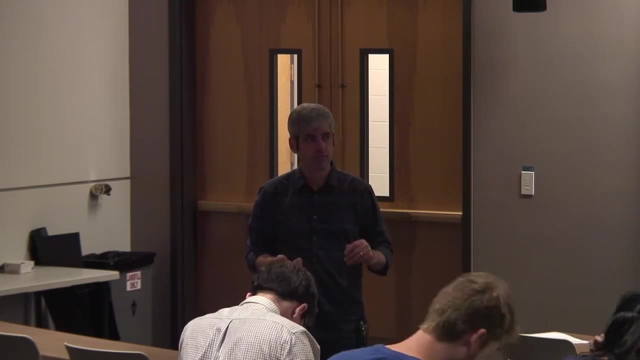 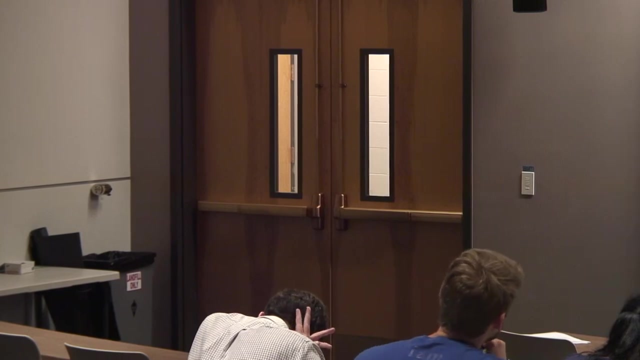 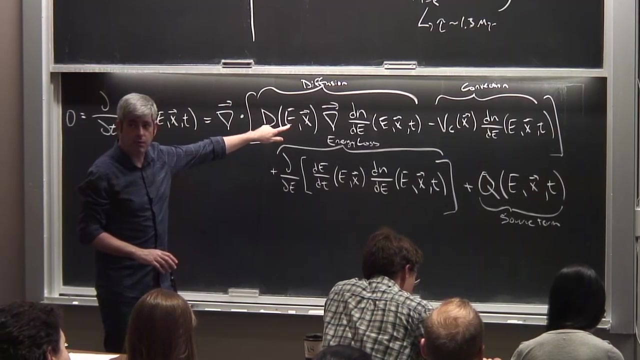 but here's the fundamental problem with trying to do it. Any kind of description you would write down in terms of the So. So what we typically Here are the free parameters that are already in the model, At least two numbers associated with this. 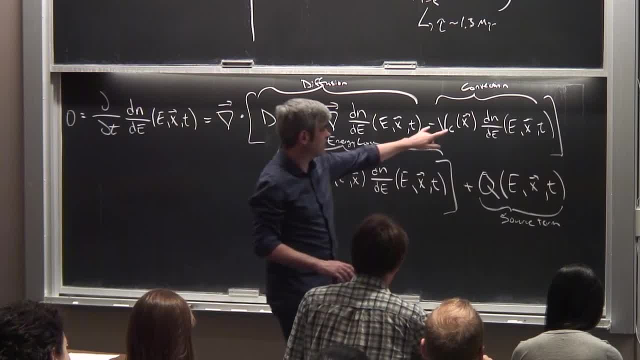 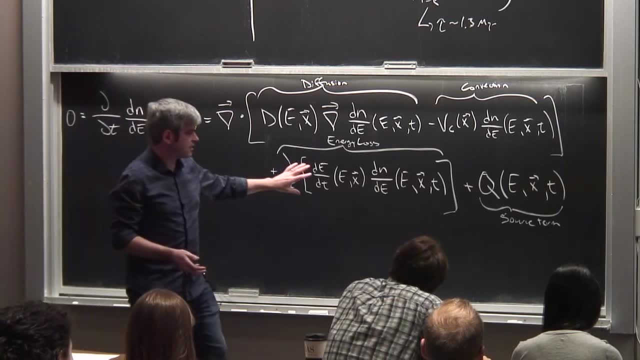 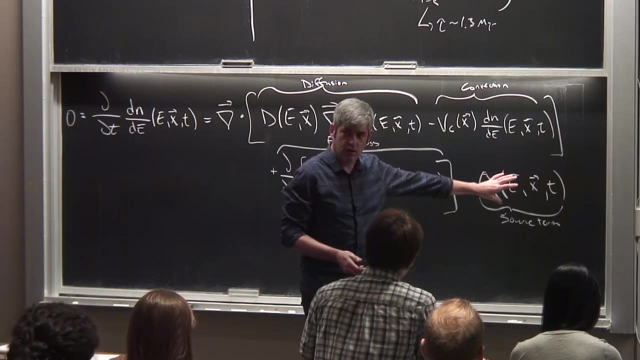 At least one number associated with this. At least two numbers associated with the boundary conditions. At least some numbers associated with the gas and radiation distribution. At least a couple of numbers associated with the injected spectrum. At least a few numbers having to do. 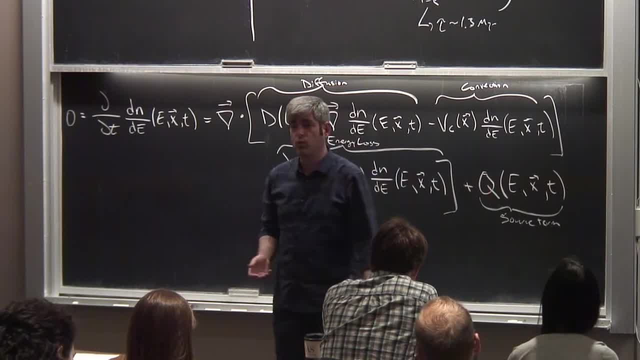 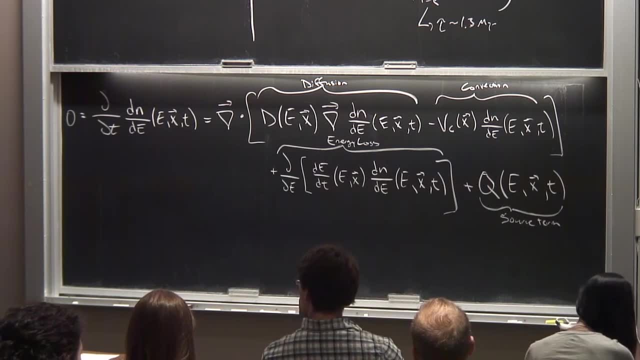 with the distribution of those sources And probably one having to do with the time profile of those sources. If you try to then put in new parameters having to do with how the diffusion constant is different in different places, you'll find you have more free parameters. 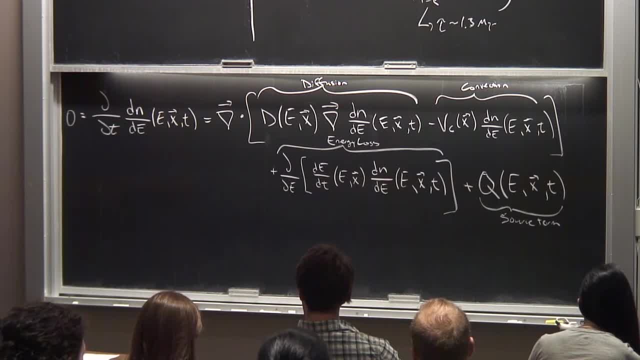 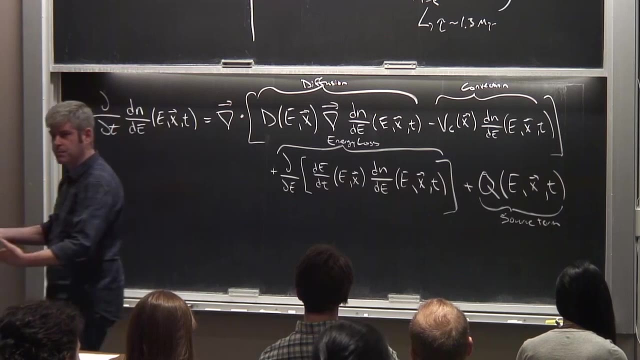 than you have data points to fit them with And you're under constrained. People have tried to do this, but my main criticism of those efforts is that they assume some parameterization. They assume it scales with the something or other of the something that we observe. 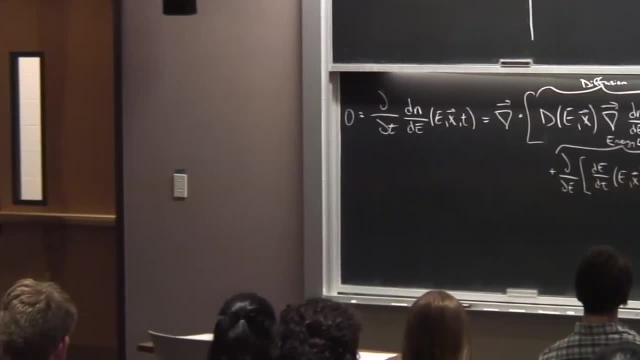 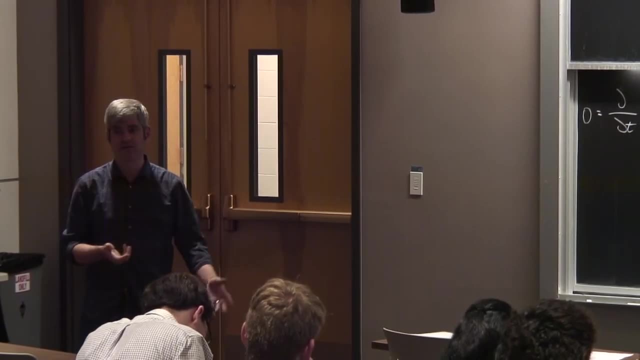 Maybe it does, but probably it doesn't, And then you get out what you put in. I don't think it's particularly predictive and therefore not particularly useful, Even though you can get kind of adequate fits by doing that sort of stuff. 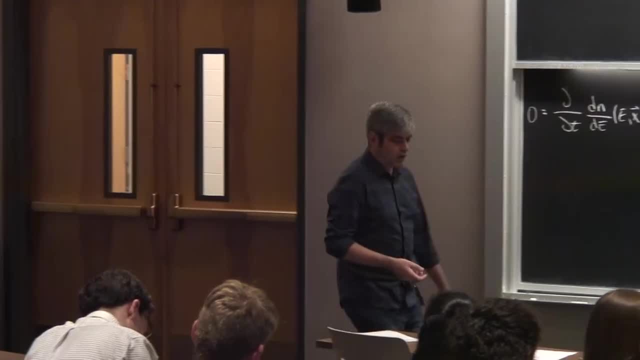 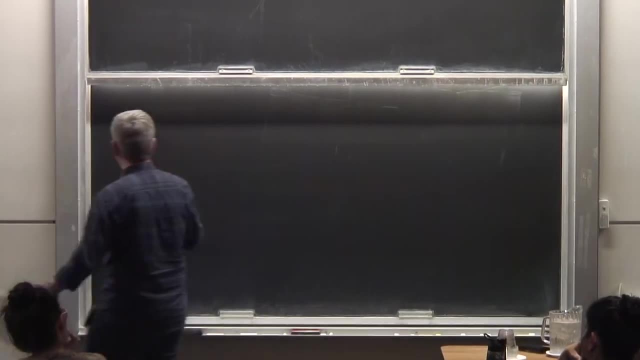 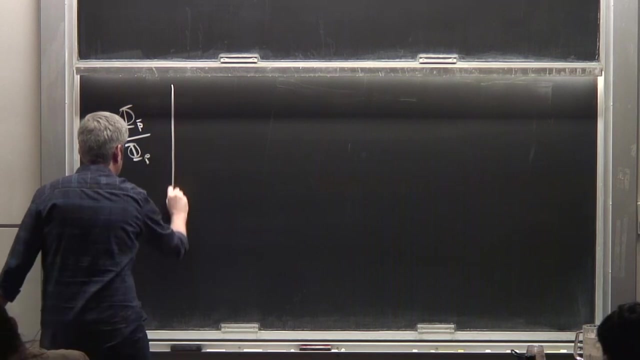 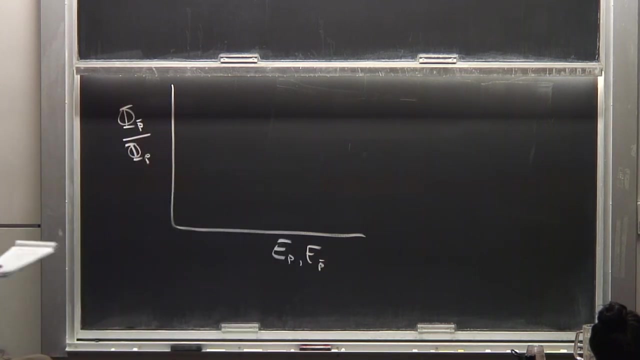 But I just don't trust it. Okay, So let's talk about real measurements. In this case, I have in mind the anti-proton to proton ratio. So this is the flux observed of anti-protons over protons as a function of their energy. So you should expect this ratio to be small, because the main way that we're making anti-protons is through secondary production. In other words, a very high energy proton hits a proton or a nuclear target at rest and that produces a cascade of particles. 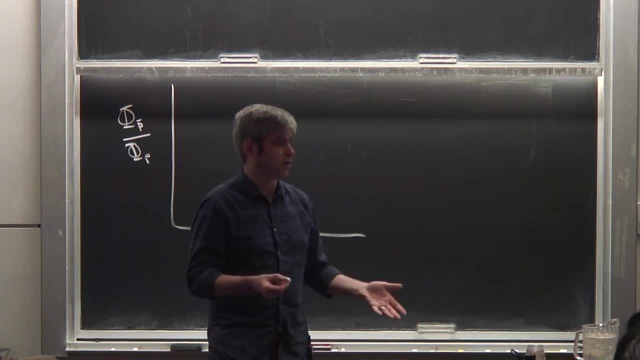 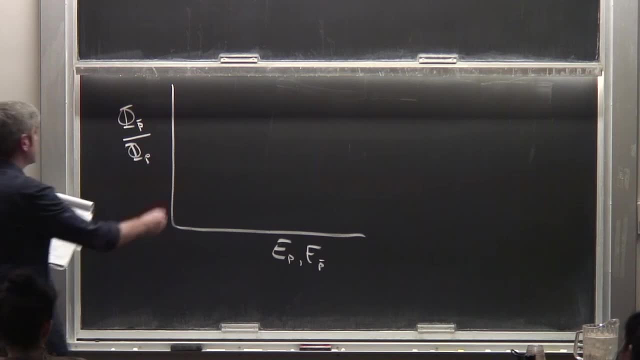 a very small fraction of the time That includes an anti-proton. That's where the anti-protons I'm talking about are largely coming from, unless dark matter is also contributing. So this plot covers, like a, a range from like 10 to the minus 3. 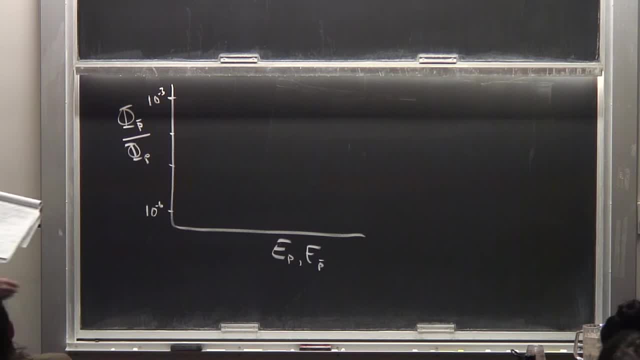 to 10, to the minus 6.. And I should also say this is not just energy. this is plotted as a function of kinetic energy. That's a weird choice, but it is a standard thing that they do in classical physics. So we have 100 MeV down there. 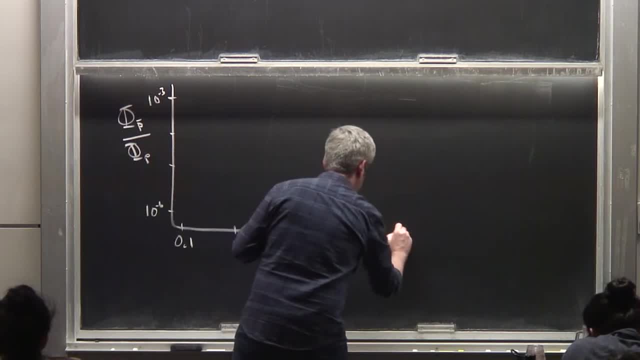 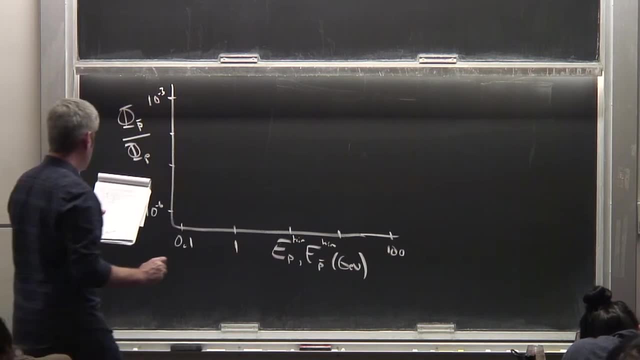 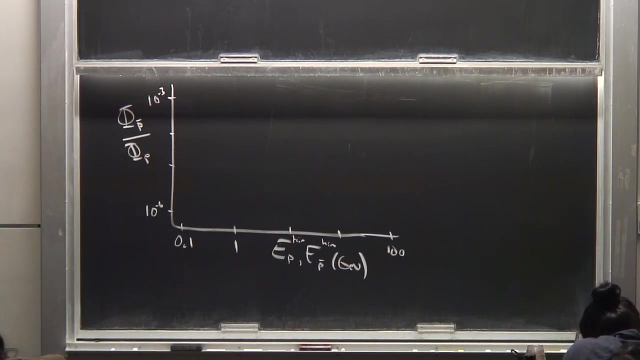 1 GeV, 10 all the way up to 100 GeV. So when you marginalize all over all the freedom in the model I talked about and you marginalize over uncertainties in the anti-proton production cross-section, which turn out to be pretty important, 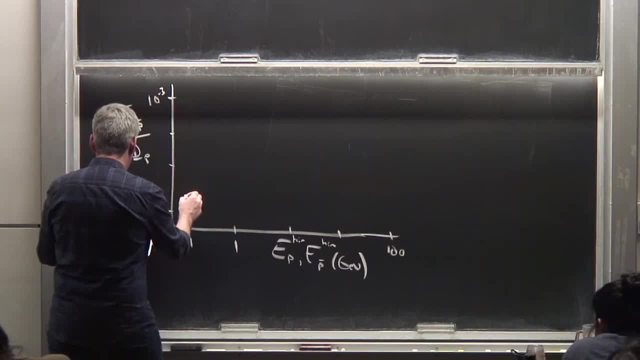 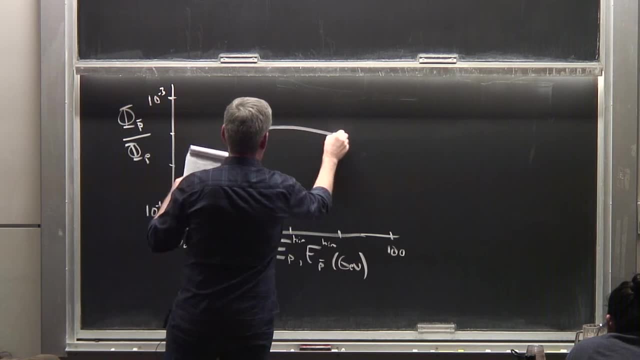 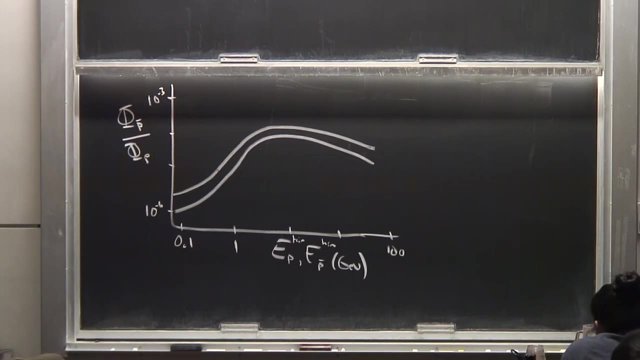 you predict that secondary production should give you a band that looks roughly like that. That is the prediction, independent of anything you've actually measured. about anti-protons, Again, we're using a spherical cow model and things you should expect there to be uncertainties associated with this. 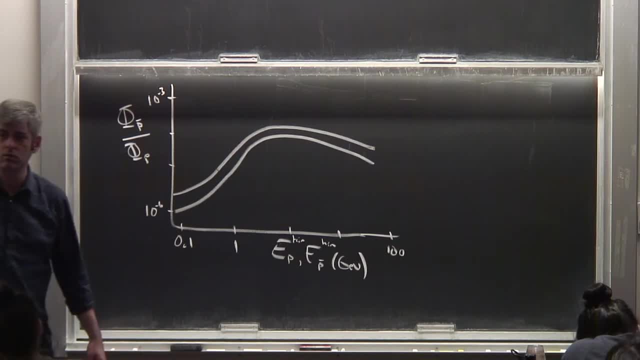 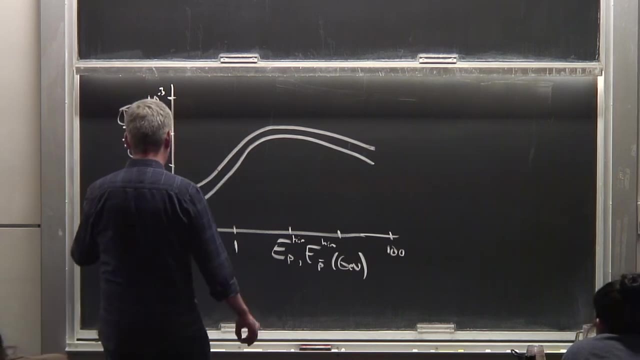 but I think this is probably a pretty fair depiction of the situation And then I'm going to kind of sketch this as an artistic depiction. but you really should look up the AMS paper if you want something more realistic. But AMS has tiny little error bars. 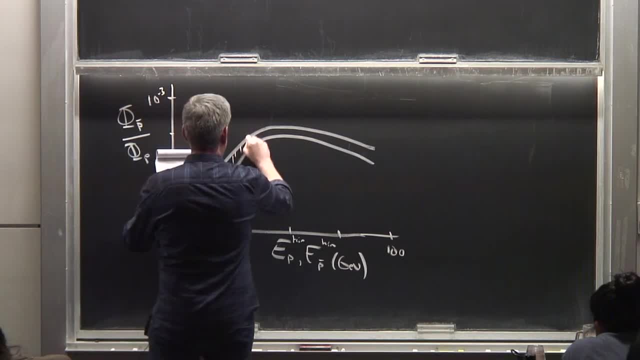 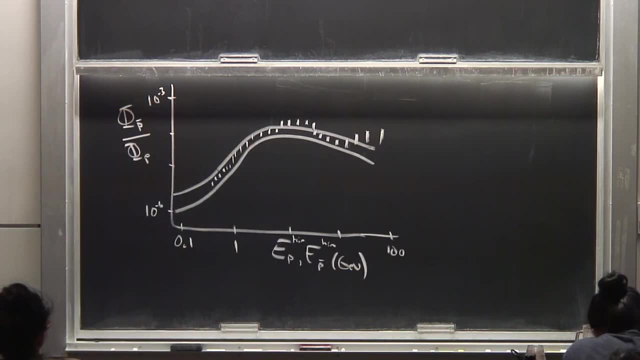 that look like this. So at first glance you look at this and you say, okay, this tells you that the model is working pretty well. The spectrum we observe is in broadly speaking, good agreement with the secondary, secondary production prediction constrained by borne to carbon. 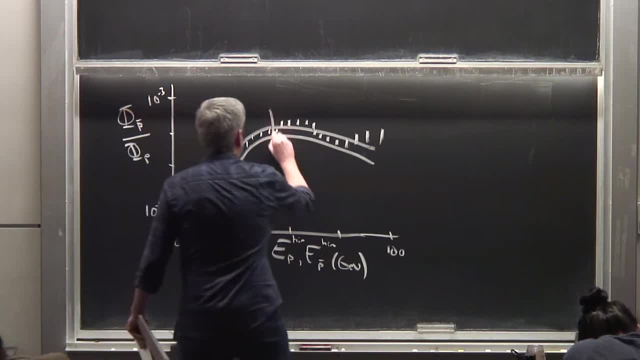 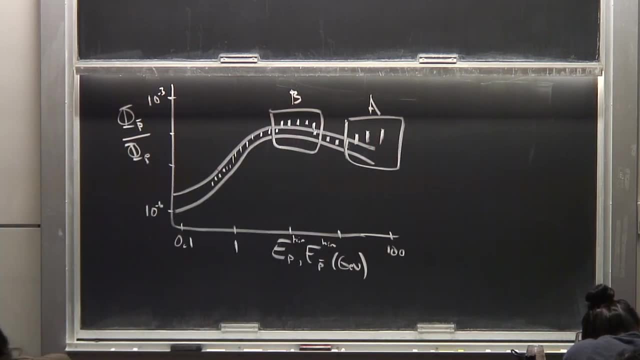 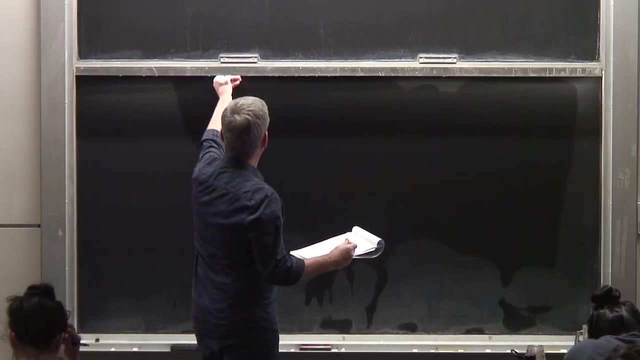 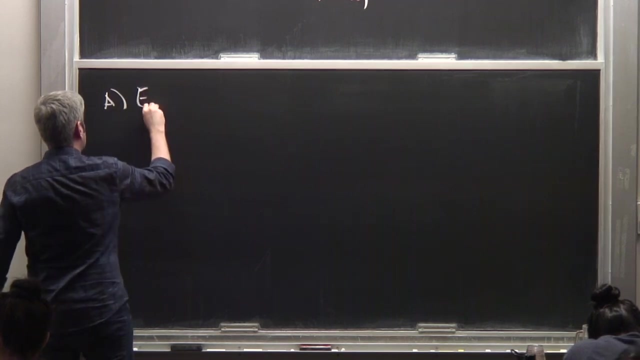 and beryllium and all these other sorts of things. There are a couple of places, though- I'm going to call this region B and region A- where the agreement is not as good. Let's talk about both of them. 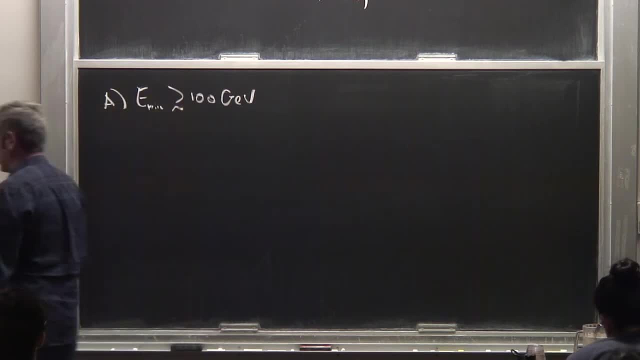 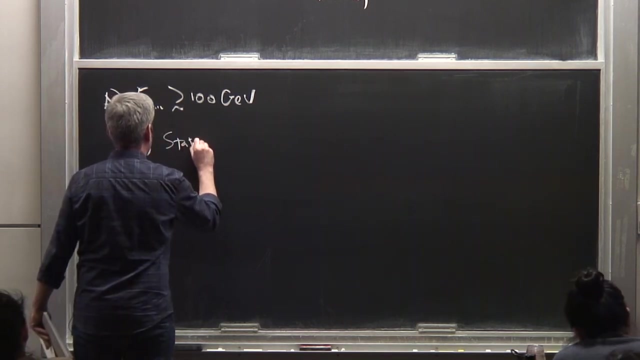 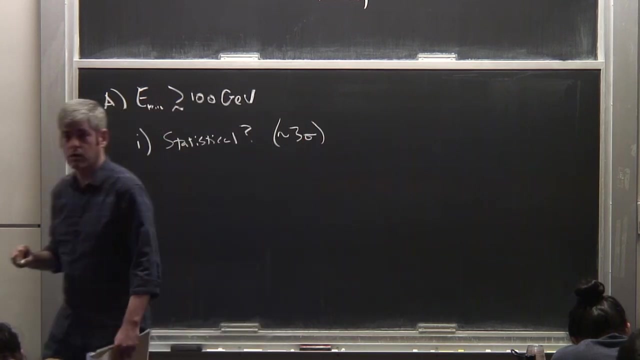 So the first region is right around- starts coming into some discrepancy with the data or the predictions: around 100 GV or so roughly. I want to make clear it's possible. this is a statistical fluctuation. It's about a three sigma departure once you take all the known uncertainties into account. 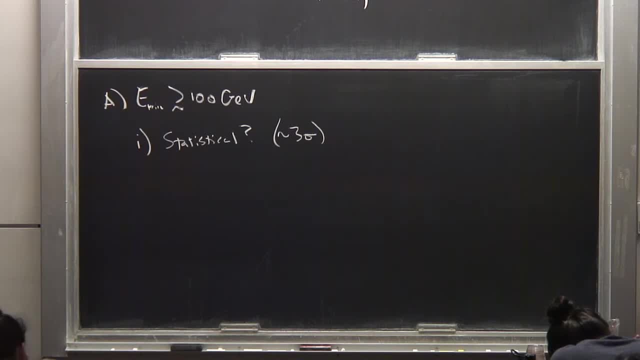 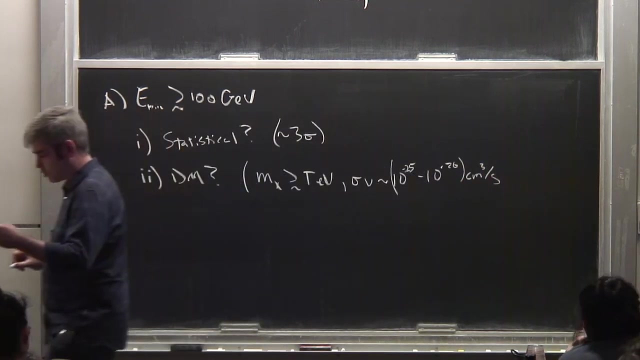 Three sigma fluctuations happen all the time, So maybe it's nothing at all. It could be annihilating dark matter, but this would require the mass of the dark matter to be a TV or more And have a pretty large cross section. 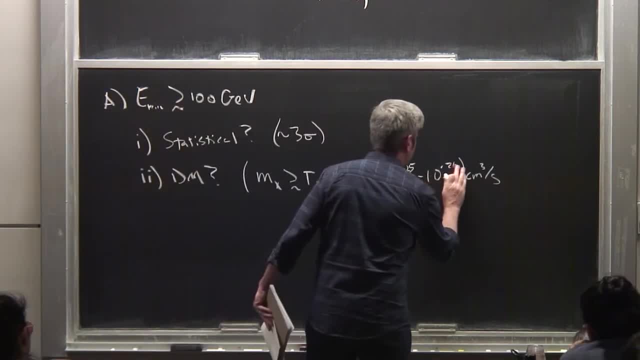 I don't mean that That doesn't make sense. That should be a 24. So well above the thermal estimate, Although not nearly as large as. But it's not that hard. And then the third possibility. 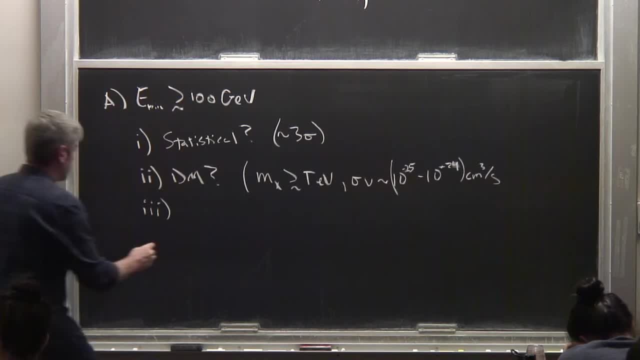 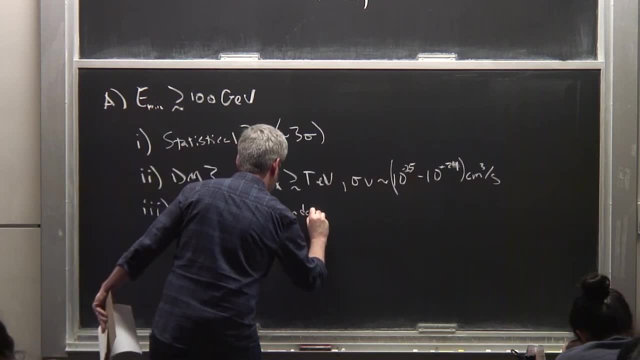 one which I think should be taken pretty seriously Is one in which you imagine that the objects like supernova and that accelerate cosmic rays In the acceleration regions, Some secondary production of antiprotons happen. So I'll draw a sketch. 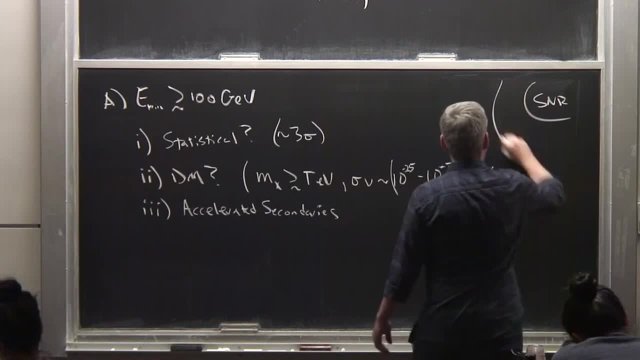 So here's a supernova remnant And there are all these shells of magnetic fields that the particles are bouncing back and forth, causing them to be accelerated. As a cosmic ray makes its way through this At some point before escaping the region, it interacts. 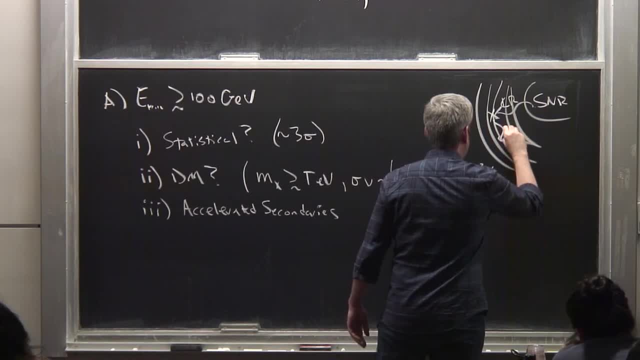 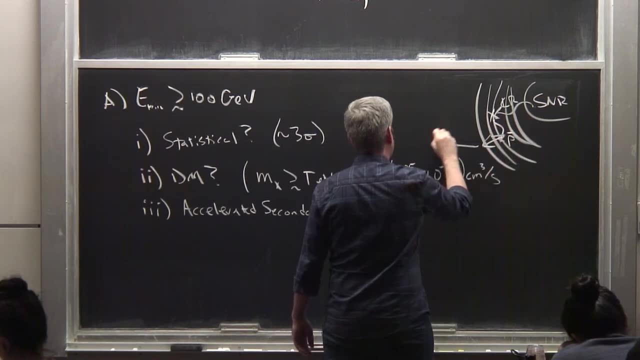 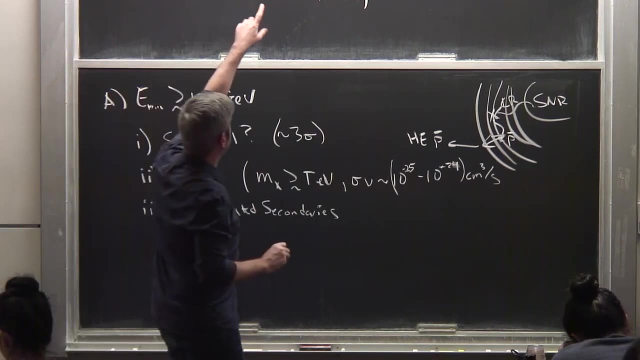 And now you have an antiproton floating around. It gets accelerated as it goes back and forth across these things And now you have a high energy antiproton being produced. And what you expect in a plot like the one on top. 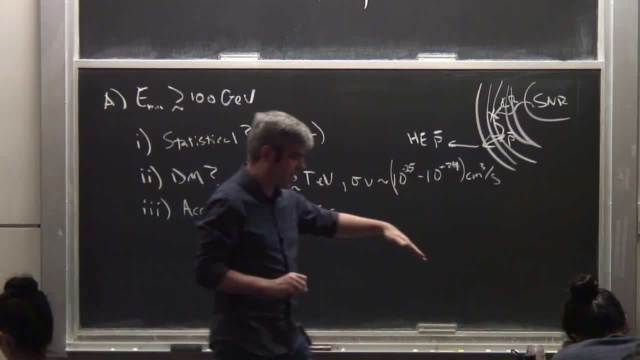 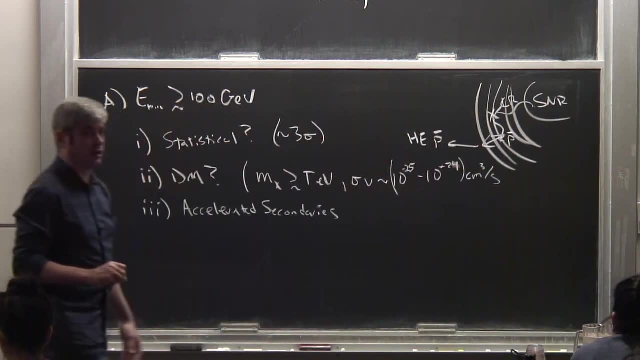 is that everything will look fine until it starts to drop, At which point the secondary accelerated component will come up. It will look just like the sort of numbers you're looking at here. We can't predict this very well Because, frankly, there are free parameters in that sort of problem. that we just don't have good handles that constrain. The way we would test this in the future is that if these supernova remnants are accelerating antiproton secondaries, then they should be accelerating boron secondaries, So the boron to carbon ratio should have a similar feature. 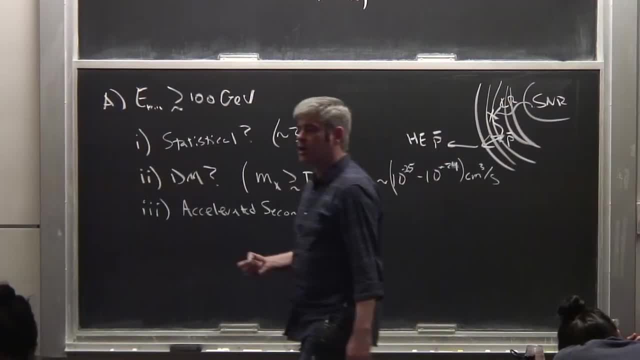 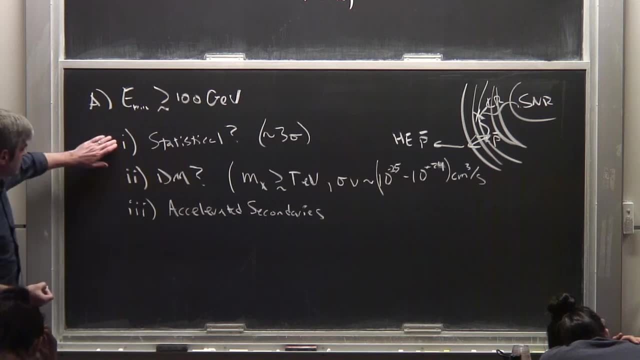 as should other secondary to primary ratios, So you can overcome this problem Right now. I think it's an open question. If I had to guess, my money is on some combination of 1 and 3 here. I don't think it's compelling evidence of new physics. 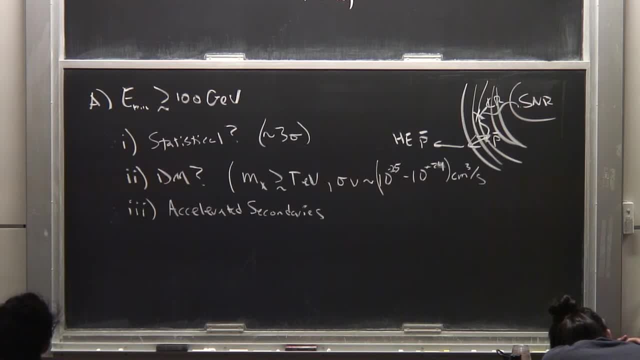 But I think we should keep an eye on it as data comes in. Yeah, 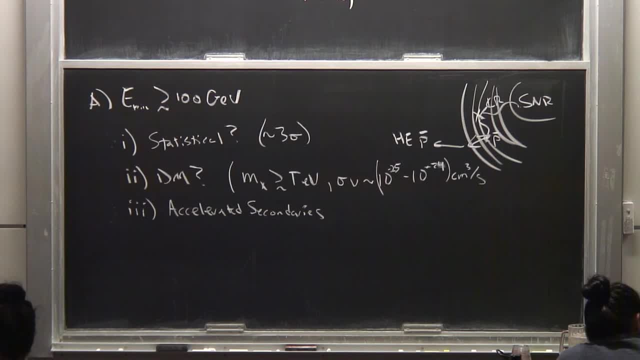 I mean that's a very model dependent statement. I mean, if you're right, if you're exchanging W's and Z's, then you tend to expect at a few TV for Sommerfeld enhancements to typically be important and then that's a perfectly acceptable. 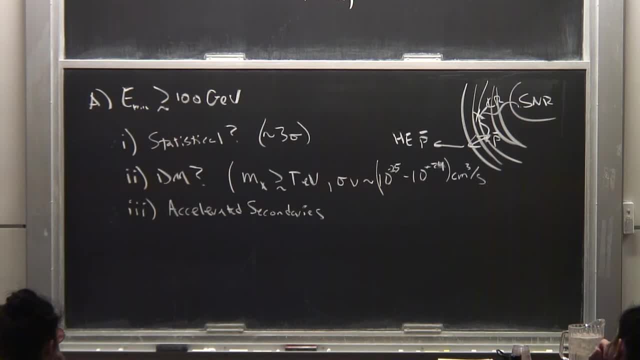 option. That being said, you know I can write down any number of other perfectly acceptable options, So any programs that are digital and, since, the new things that you're doing, the programs that you're working on. So Maxwell's equations are entirely symmetric with respect to charge. 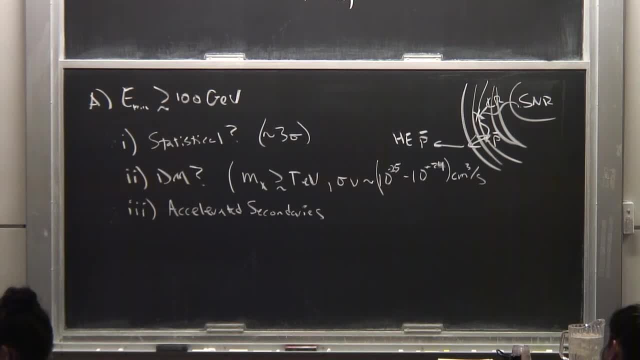 So if I describe a statistical distribution of magnetic fields and I ask statistically how a positive or negatively charged particle will behave in that, you get the same answer, Even though an individual trajectory will be reversed, as you say. So let's go on to talk about region B, So I'm going to unfortunately have to cover it. 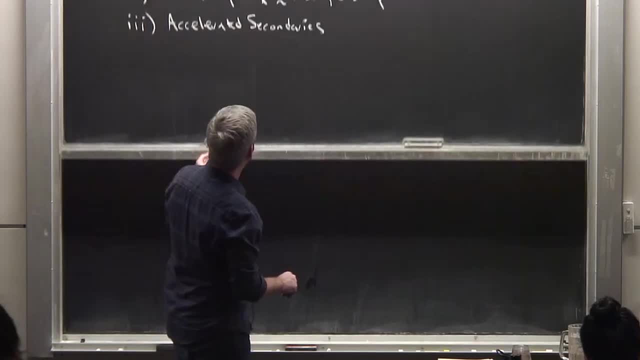 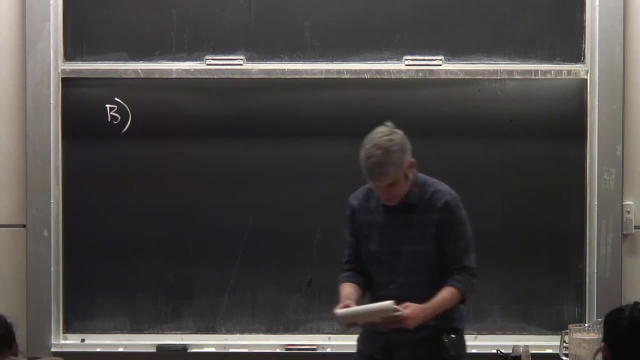 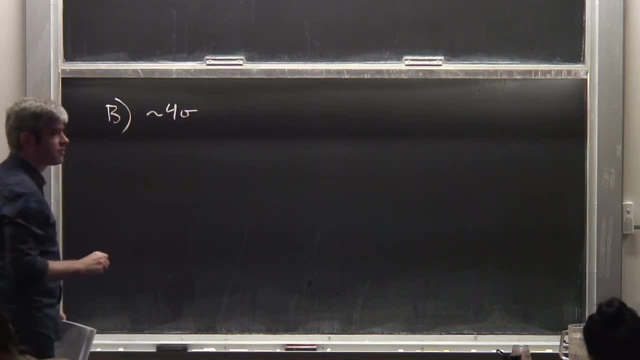 I think region B is a little more interesting. It's probably about 4 sigma. Some have claimed 5, but to be conservative about 4 is probably what it really is, Again, in the context of this model, and you can imagine lots of departures from this model. 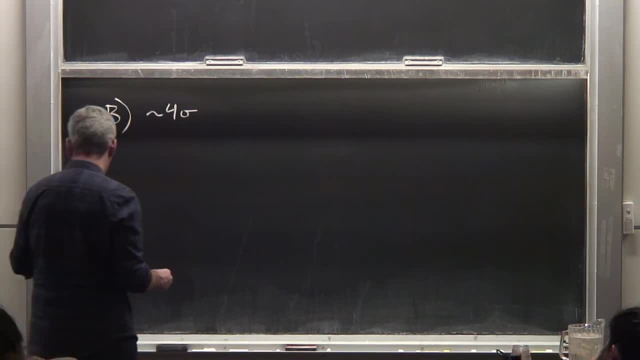 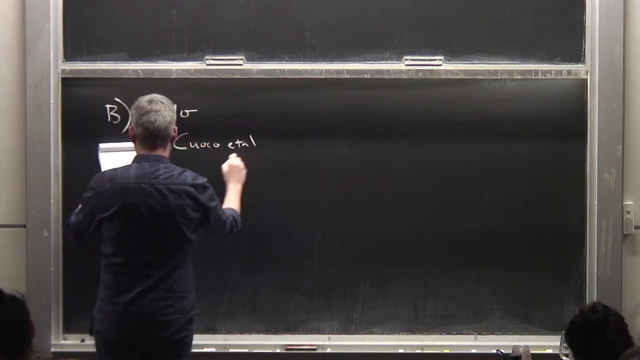 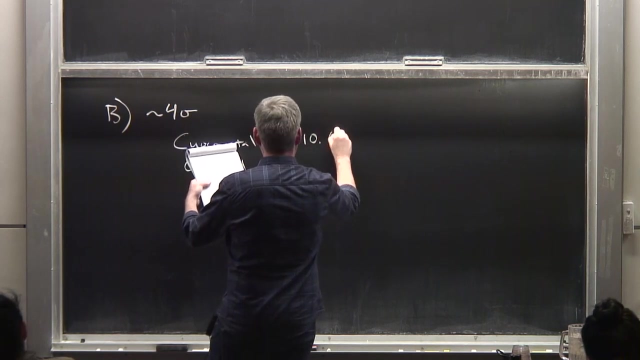 But at face value it looks like it's about a 4 sigma excess. Some papers that talked about this originally are Cuoco et al, Cuoco et al And this group, And they came out practically at the same time, Reaching effectively identical conclusions. 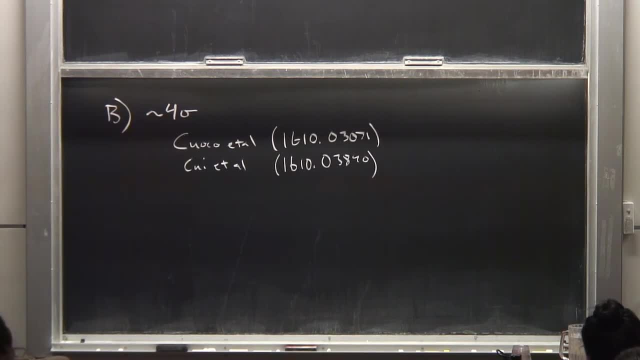 And since then several other groups have found the excess. Efforts have been made to try to make the significance of the excess go away by adding new uncertainties in various parts of the problem And you know, the best case scenario is it's maybe 2.5 sigma. 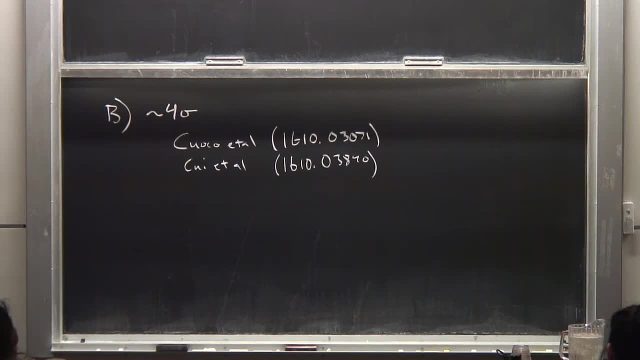 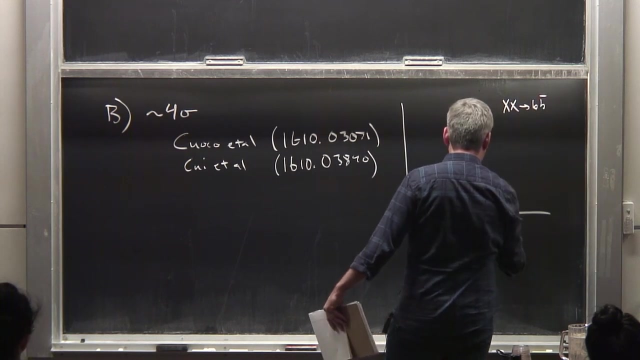 2.5 sigma, 2.5 sigma, A statistical fluctuation on top of large systematics Like that's the sort of thing you can imagine If I interpret this as dark matter. And here I'm going to say: Consider the BBBAR channel. 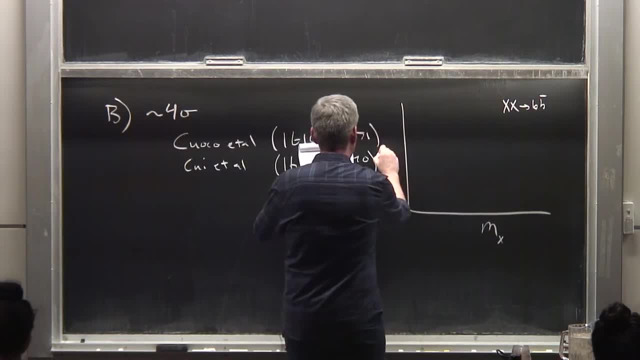 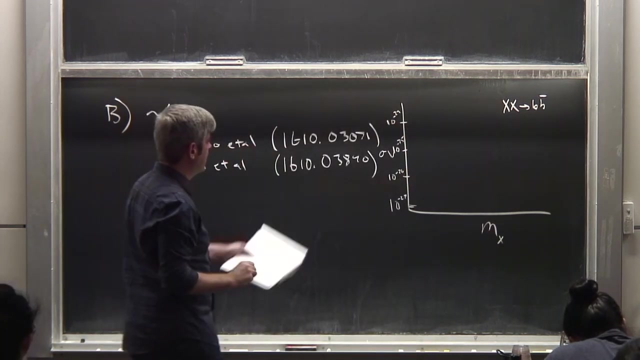 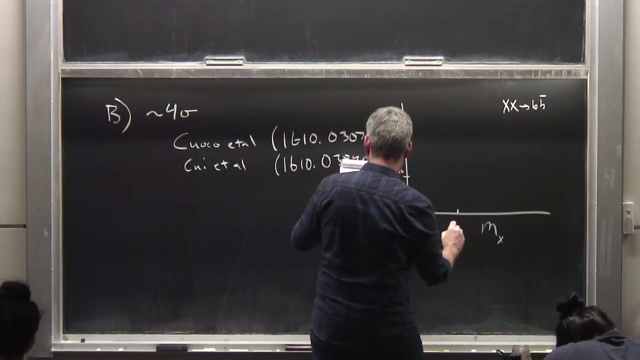 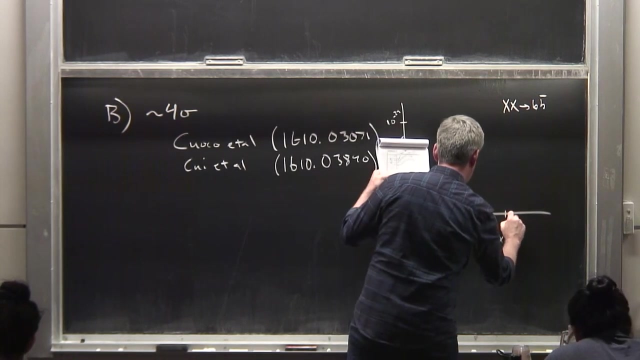 But you know, I could again consider other hadronic channels to do this. There we go. Great, these are in cubic centimeters per second. again, 10 to the minus 24, 25, 26 and 27, and I'll go all the way down. oh, I'm doing this wrong. 10, 10, GV, 100 GV and TV, and the limits look like this: 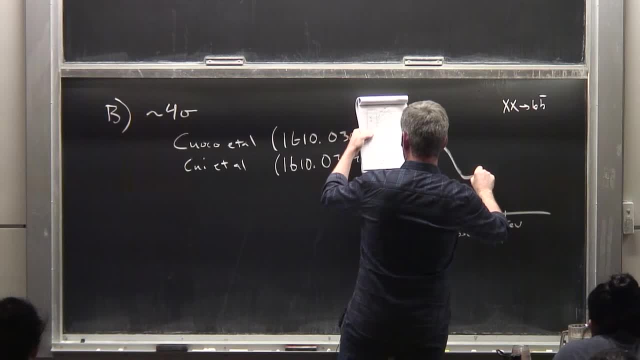 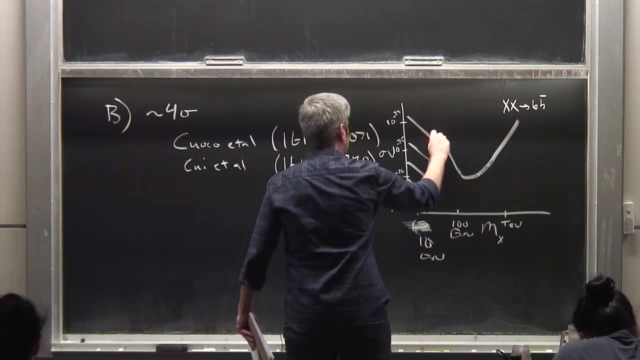 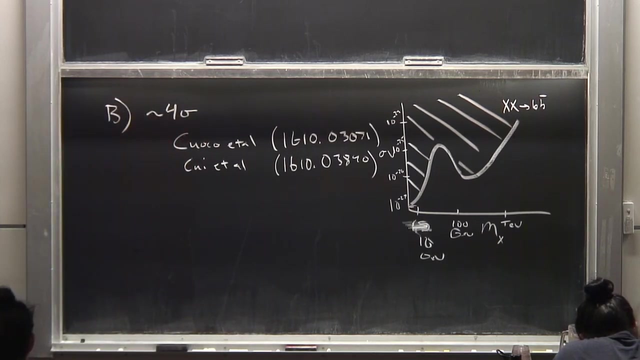 about. so everything above that curve is excluded, at least if you take this sort of transport model strictly speaking seriously. whenever I look at a limit like this, I multiply all the limits by a factor of two and three or something, and then I think I can trust it. 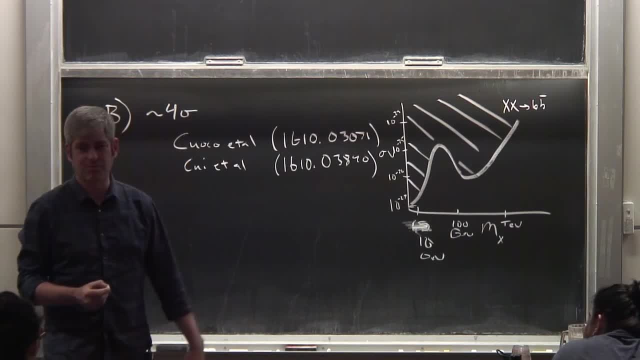 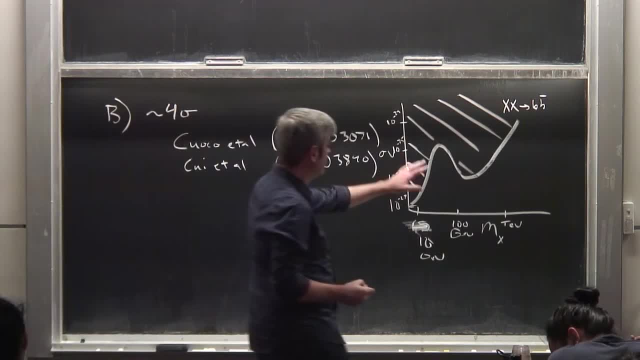 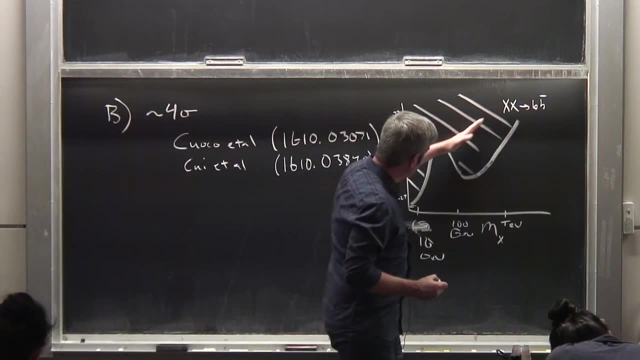 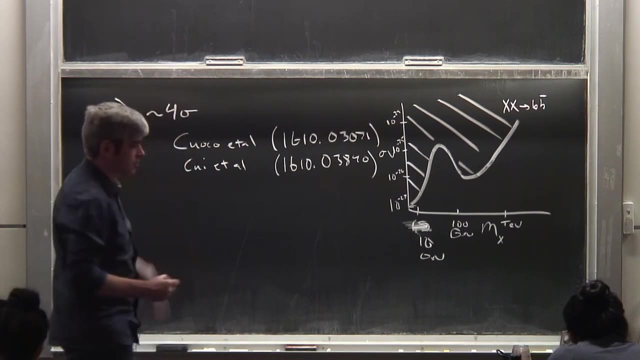 reasonable, fair thing to do. so if I compare this to the constraint from Fermi dwarfs, it's a very strong limit. Fermi dwarfs lie like something like this: okay, so unless you're near this feature which corresponds to it to the region B I was talking about, unless- 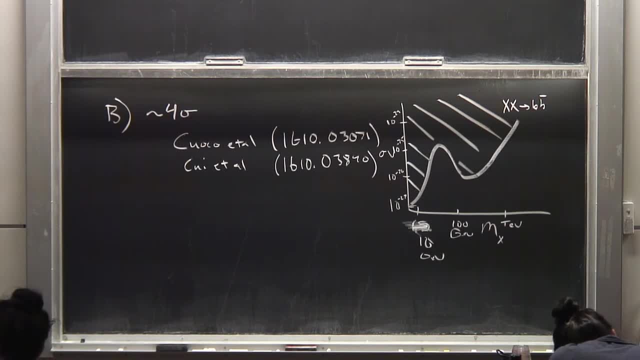 you're talking about the feature. this is the strongest limit we've got on hadronic annihilating dark matter. okay, so B's is strongest limit for B's, but for any kinds of quarks and, frankly, for annihilations of W's and Z's as well, or Higgs but right around. 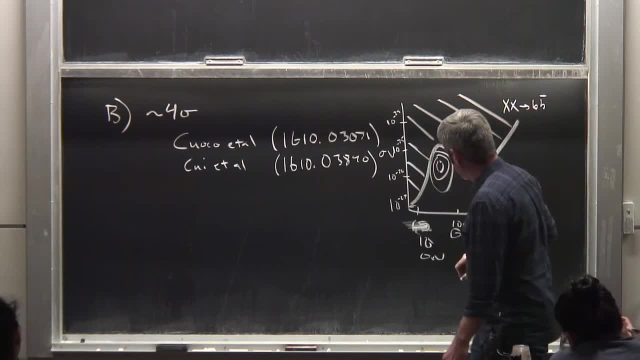 here. this is where that axis lies. so I will just note in passing- and then move along- that that's about the same place that the galactic center axis lies, and it's about the same place that the recticulum to another dwarf axis is lying. so I don't know what to think of. 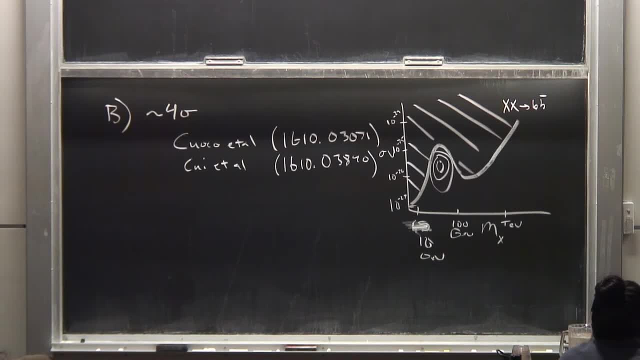 it. I'm putting it out there. I'll I will simply say there are a lot of different opinions about what this might originate from and I certainly don't have my mind made up. so that's the current state of dark matter: searches with antiprotons. I think this limit 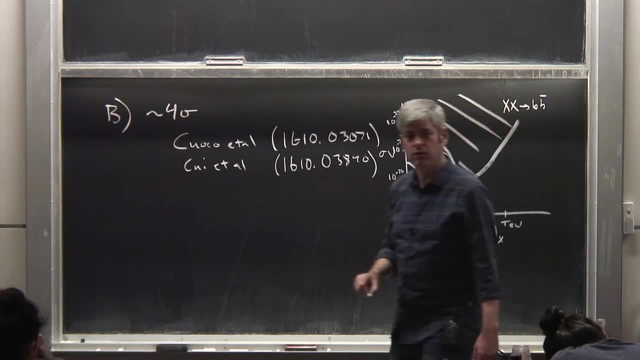 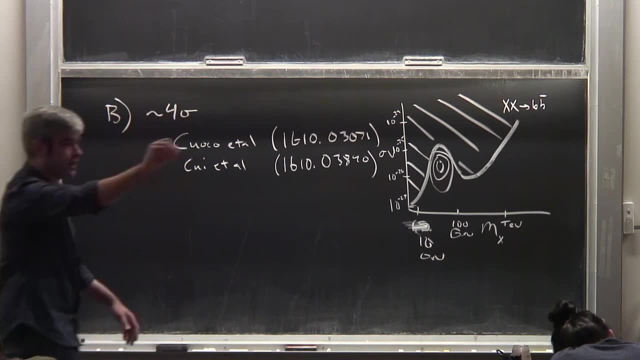 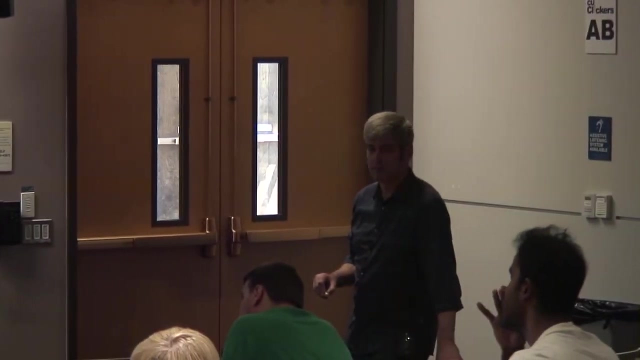 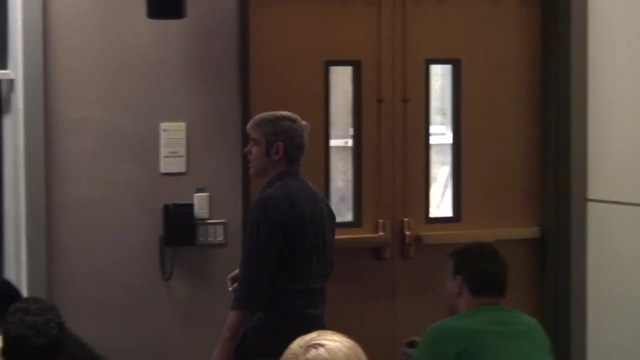 should be taken very seriously. I think this access should be explored more in the future and probably the higher energy access should get some more attention to, but I think that will solve itself with with more time. Quark data: yes, okay, that's right, this is a limit on the dark matter annihilation cross-section to in this particular plot, BB. 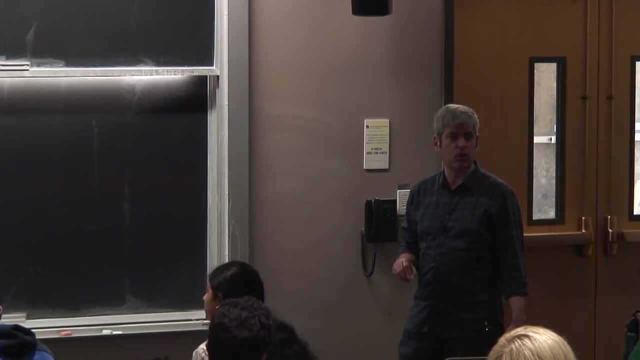 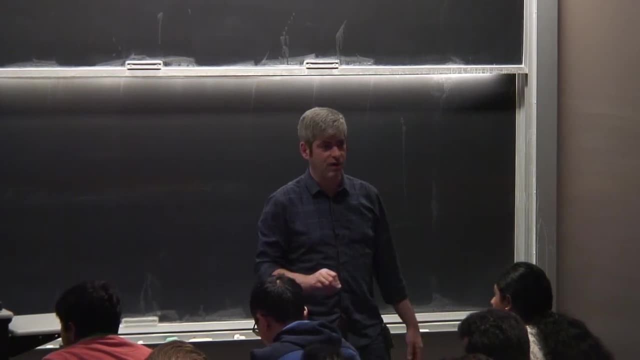 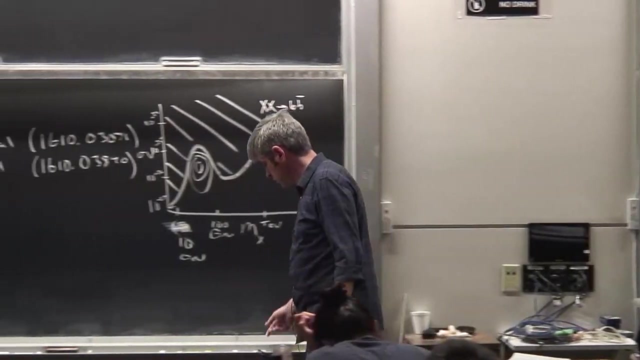 bar, but I could do it for other types of quarks and get similar answers, and it's been done for other types of quarks. I'm just showing a common benchmark for the sake of brevity. the literature definitely contains results like this for other channels. 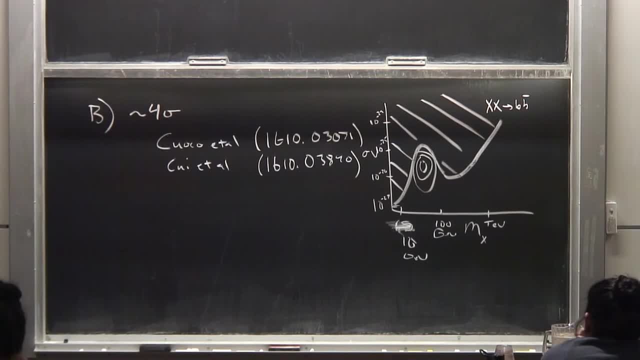 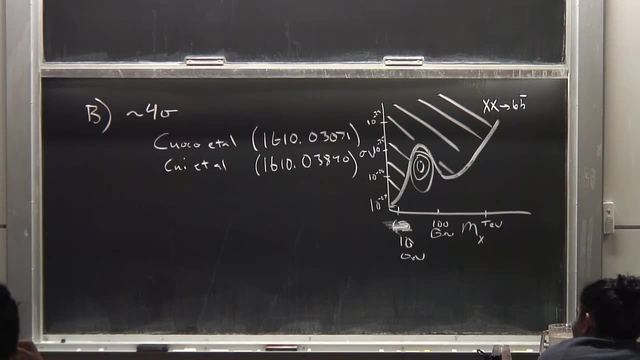 it is, but you could scale it easily if you're only if you're going 50% to BB bar and 50% to invisible, then it just scales by a factor or two, that's it. if you're going 50% to BB bar and 50% to tau plus tau minus. 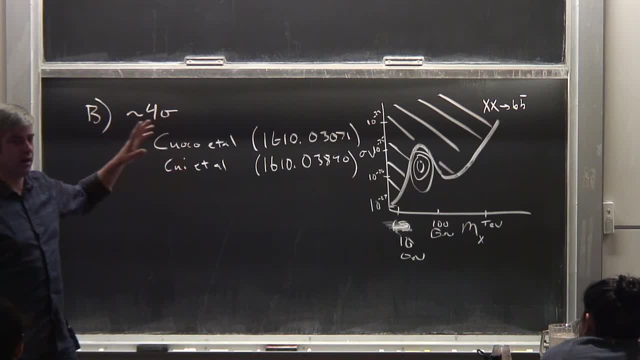 actually know it, that would scale exactly the same way, because taus don't make antiprotons, but 50% to BB bar and 50% to W plus, W minus. then it would be more complicated and you'd probably have to use pithia and run the spectra and 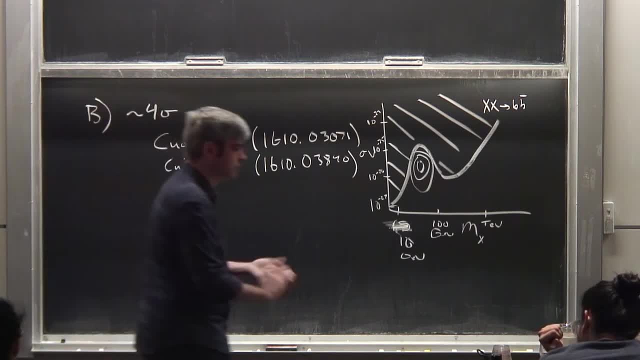 add them together and things like that. So in the A case, that's an accelerated sample that you were saying here, that people were suggesting was systematic. so they're like specific mechanics: people could try and track down and test whether or not they're going to be able to do it. 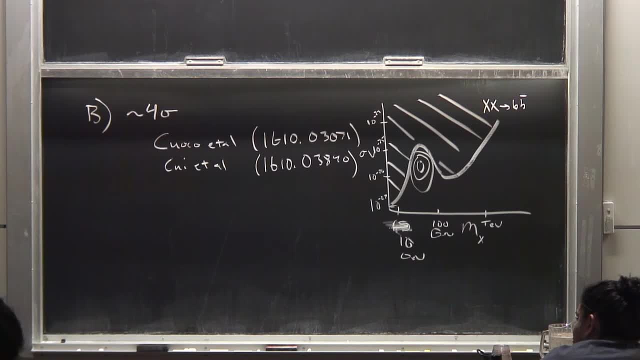 Yeah, That's a thing. So there are different groups that are talking about different things In the accelerated secondaries thing. the beautiful thing about that interpretation is this: is the data look like what it should look like if that was what was going on? 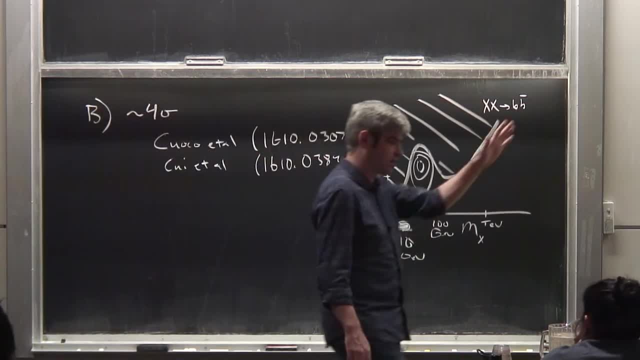 You should expect it to agree very well with the model at low energies and then to turn up in almost exactly the way that's being observed at high energies. and the other beautiful thing about it is there's a very clear path forward. you measure born to carbon better. 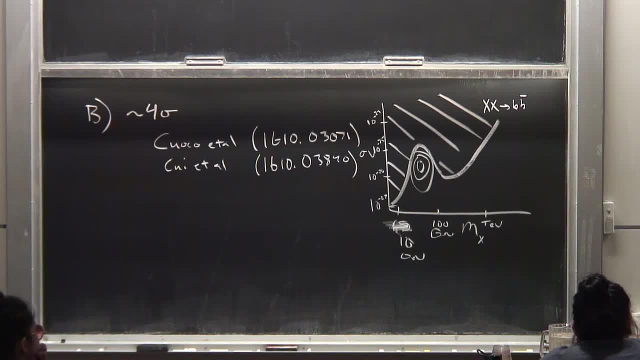 you measure other, secondary, primary Better and you just see: is it doing that at the same same way and either answers yes or no. it will, we will. we will be able to answer that with AMS data in the case of XSB. basically, instead of there being some physical mechanism people are talking about, they're just saying 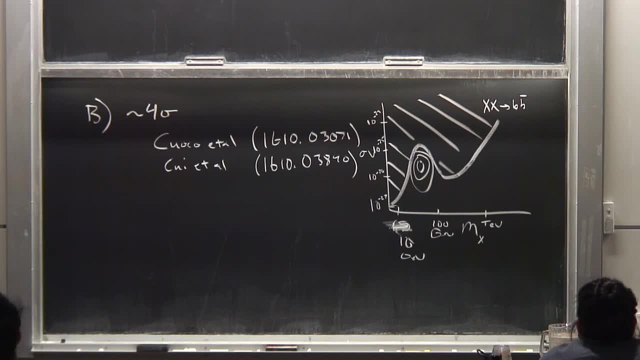 well, what if the anti-proton production cross-section has a little bump in it here- and it's a bump within the errors- and you could parameterize it that way and not have a terrible fit, And that could cause this feature to flatten out. It's not very compelling. there's no reason to think that's what's going on, but I think 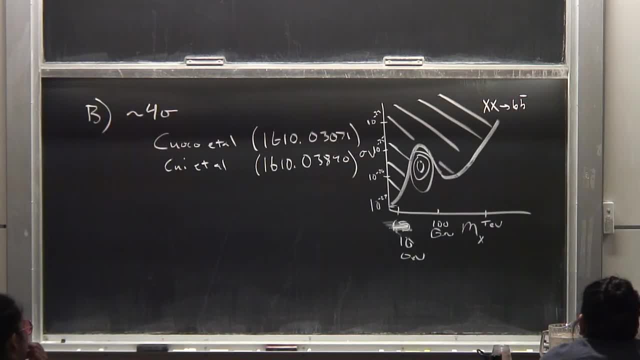 one has to be open-minded about that sort of thing until you measure it well enough to be confident. that's what, not what you're seeing. And even when you do stuff like that, like I said, there's still a two and a half sigma excess of recent roommates. 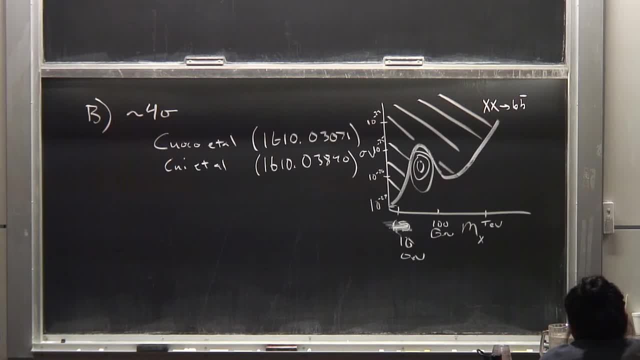 Oh, those are the, you know, one, two, three sigma preferred regions. Oh, I said that it turns out. you know, if you look at the galactic center XS and ask- and I put the ellipses there- it's about the same place. and if you look at the dwarf XS as excesses. 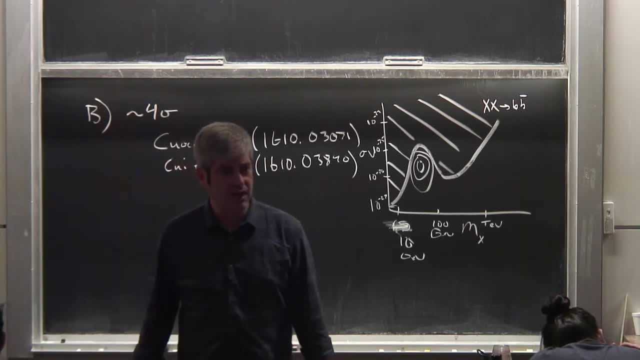 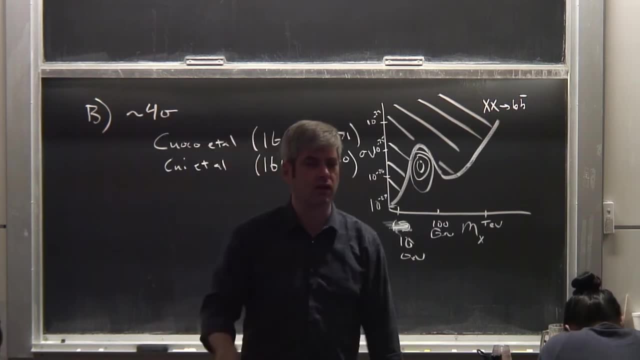 have been seen by Fermi, although those are modest and statistical significance. they prefer regions in the about the same cross-section mass values. So all those, those excesses kind of favor the same sort of dark matter interpretation. That being said, I do not want to convince anyone. 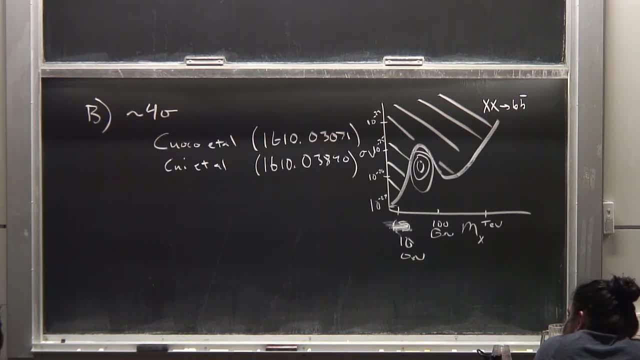 I don't want to leave anyone with the impression that this is a settled matter or anything remotely like that. These are our various hints and suggestions, and I think there are things they get excited about, but not things to reach strong conclusions about At this time. 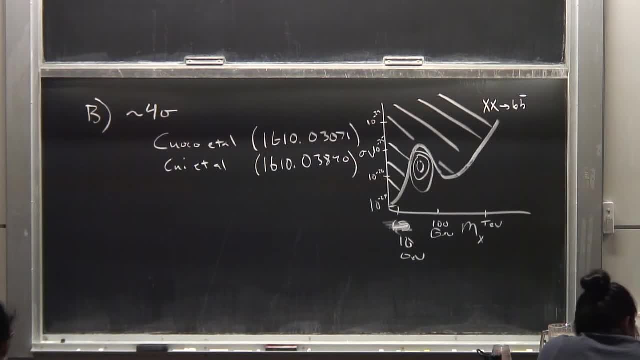 Yes, Having both existences like this, one assumes that the norm is a constant and the other they're all going to be proton and antiproton, and the other one seems to be like proton excesses, And so these limits will change. if we say we could annihilate either photons or 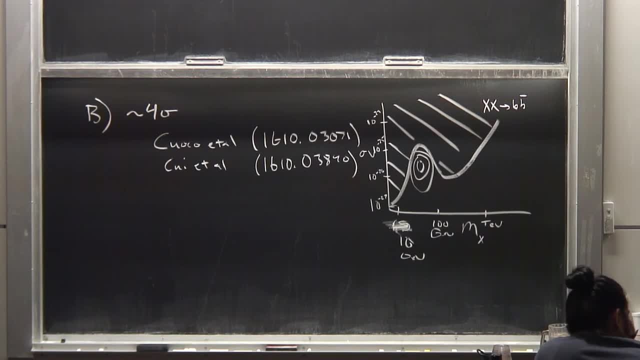 Well, so we're not annihilating two photons or two antiprotons, We're annihilating the BB bar, and we use what we know about QCD and other in the standard model just to determine what happens when a B decays. So so I the only thing that goes into this comparison is this choice: the BB bar choice. 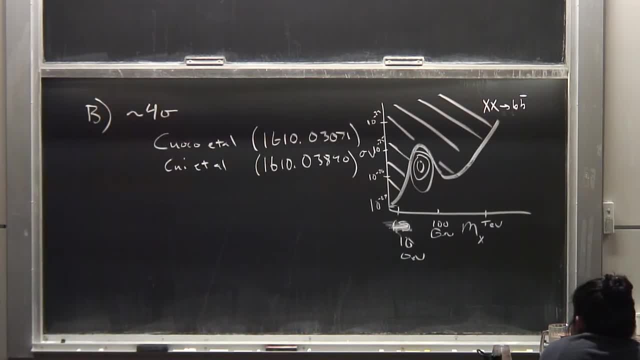 And you can do it for others and it works approximately equally well. So I don't. This is just an example, but it isn't a cherry picked example. It's just the benchmark I chose to use throughout these lectures and, frankly, it's the most common. 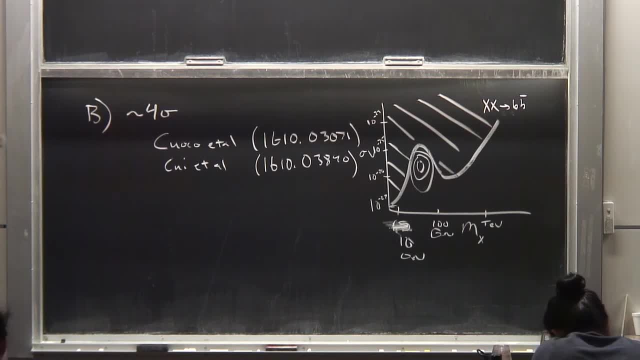 benchmark in the literature. So is there any suggestions specifically to do the test, whether or not this is free? Is there any direction to bring this and determine anything? So people have been making suggestions that we should do a dedicated laboratory experiment to measure the 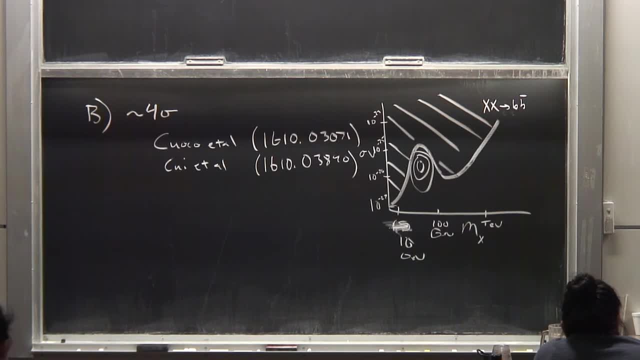 Antiproton production cross-section better. I'm one of the people who have argued that for some time now. I think it's kind of strange that we put a multi-billion dollar experiment in the space to measure this thing without doing the, you know, 10 million dollar experiment on Earth. 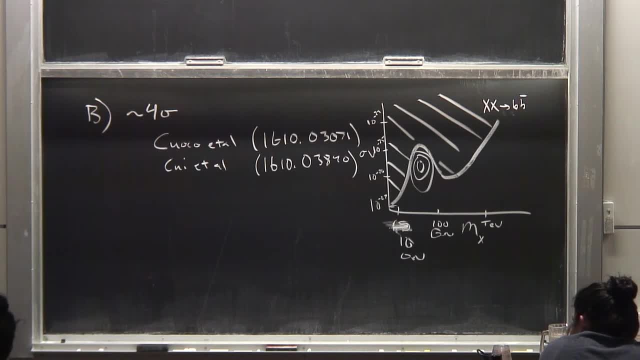 that would allow us to make full use of that data. So I don't want to divulge into or digress into politics, but but yeah, I think something like that makes a lot of sense. But it's also just the case That as the data gets, you know, accumulates, and this will either become more or less statistically. 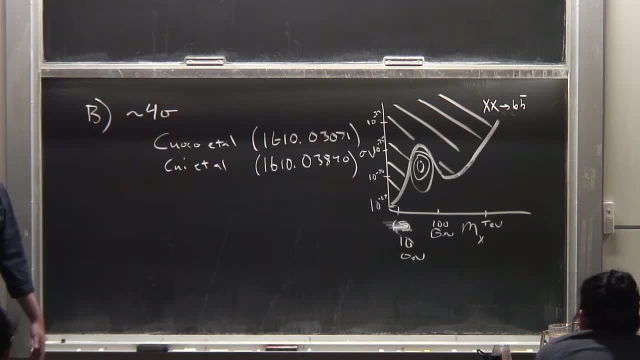 significant as time goes on, And I think we'll know more about it in the years ahead, even if we don't do any new strategic moves to do so. What would it mean if the census was exclusively a judge of that? What would that mean for the other? 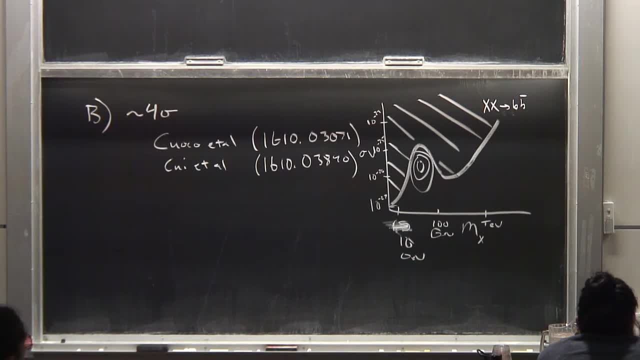 I mean, Would you have both, Or is it a question of what? would it be? Oh, A and B you mean? So like if A? they tested and they found that there definitely wasn't the moron, so this was definitely the moron. 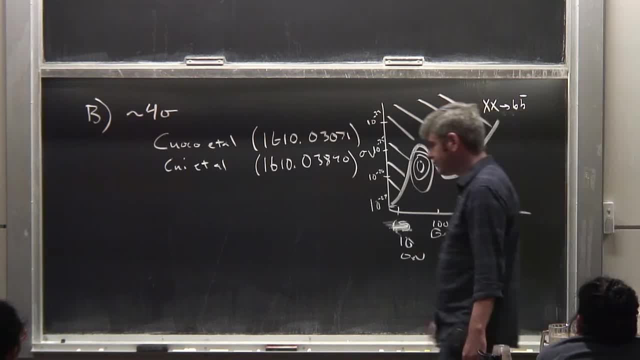 So if A they tested and they found that there definitely wasn't the moron, So this was definitely the moron, So this was definitely the moron, So this was definitely something new. What would that mean for B and vice versa? I mean, I guess you could always invoke multi-component dark matter, but you know, that seems 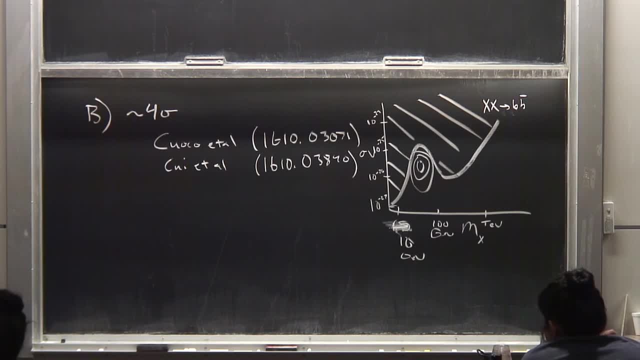 This data does not seem to call for anything that desperately. But if one day it became very, very clear that you couldn't explain either of these, maybe people would start talking about that sort of interpretation. But not anytime soon. Alright, so let's go on. next to positrons: 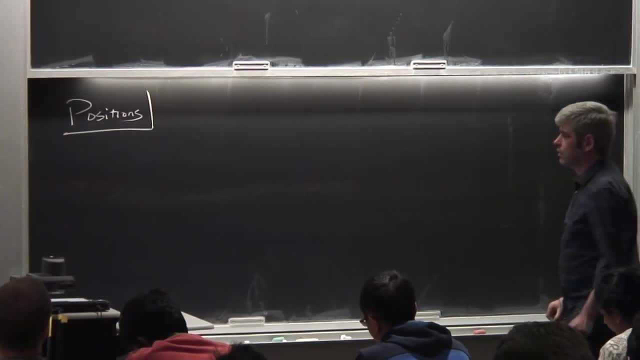 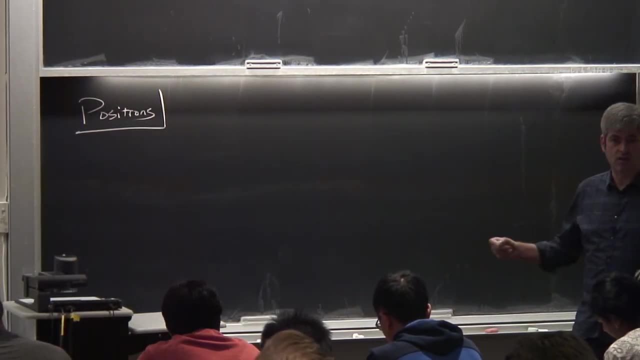 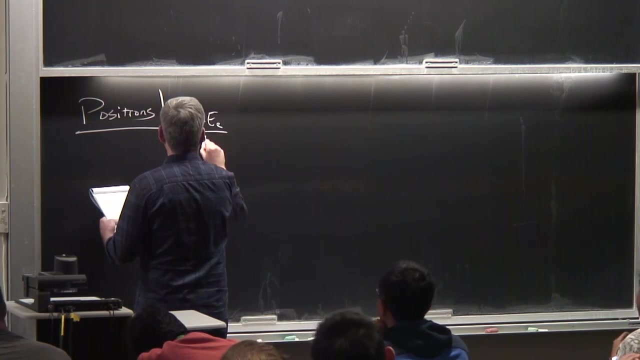 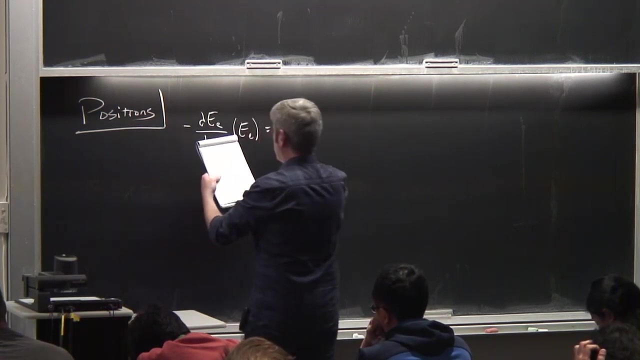 Which are different than antiprotons and anomalies. So this is a number of important ways. In particular, they lose energy as they travel in a non-negligible way And this has all sorts of bearings on these calculations, So that energy loss term in the equation in the far left board, there for an electron or 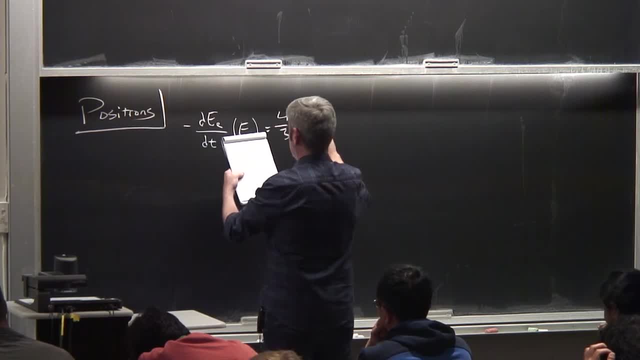 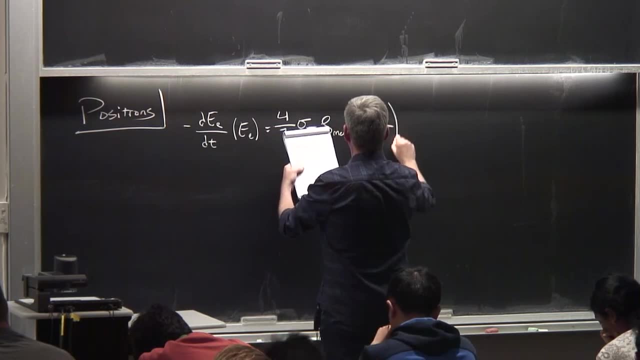 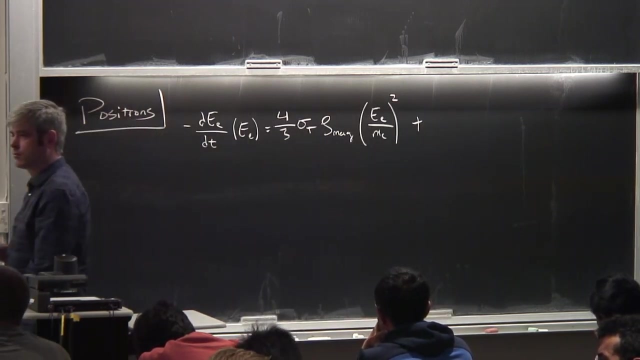 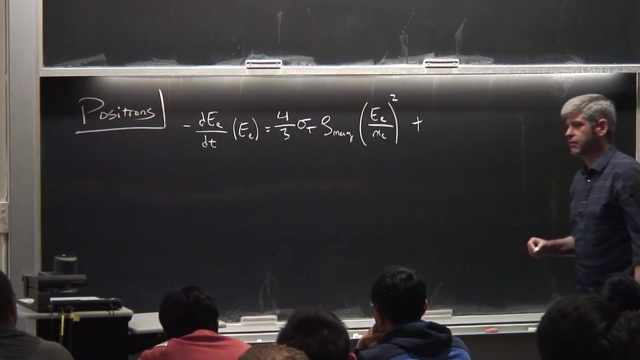 a positron looks like this: Okay, Okay, Okay, Okay. It turns out that antiprotons have a fairly high chance of annihilaing with something It doesn't. actually, though, I can see why you might have imagined that intuitively, but if 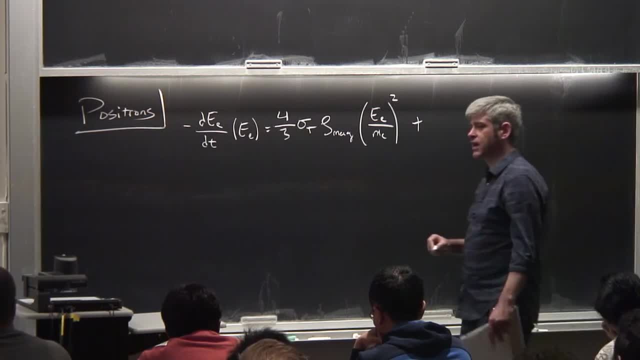 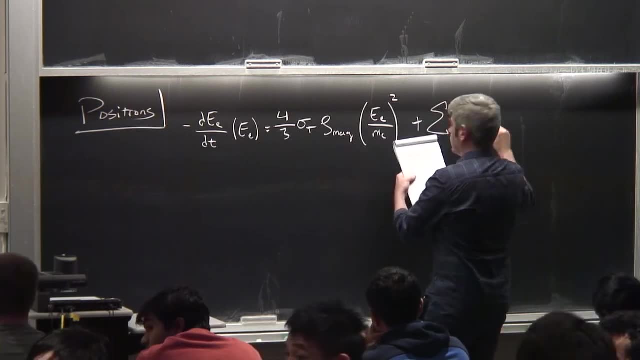 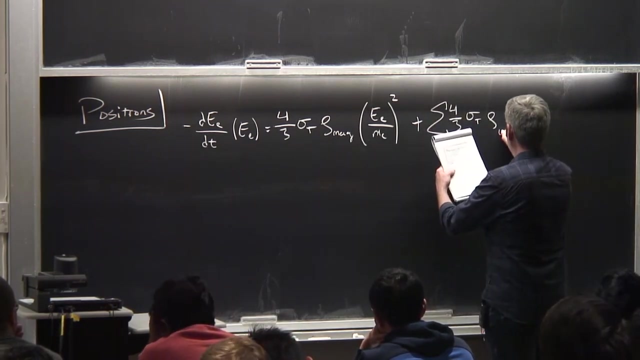 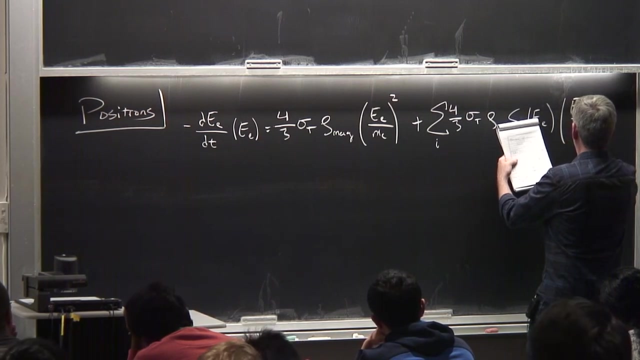 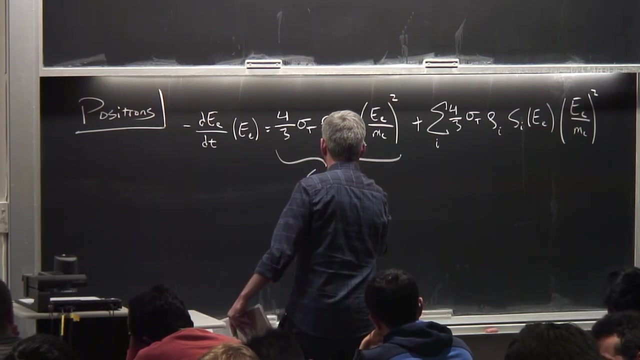 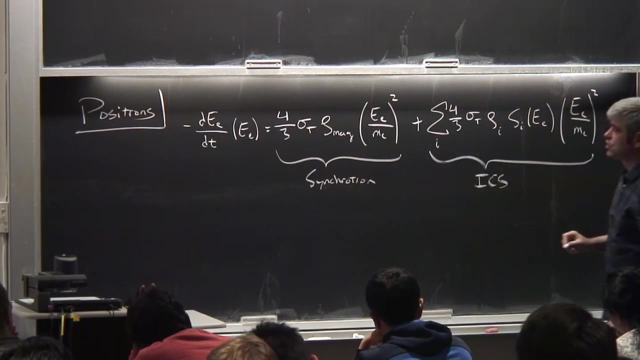 you do the calculations, it's a negligible chance in the kind of time scales that these particles travel. Sorry, Magnetic, That's the energy density in magnetic fields It is. I'll explain this in a second. Okay, So this first term is our energy losses from synchrotron. 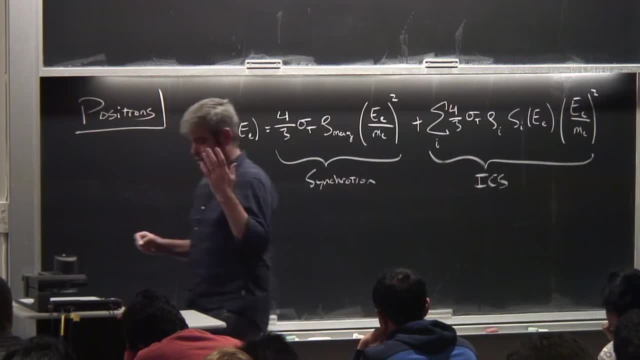 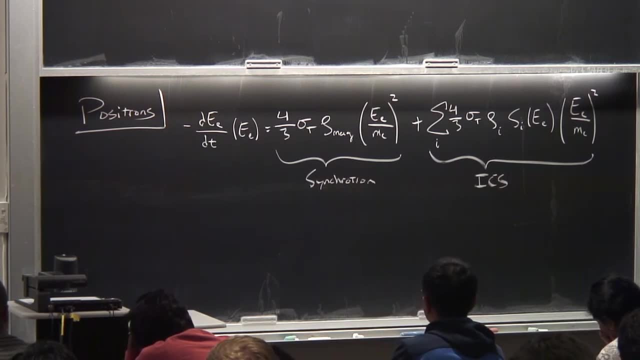 So what I have in mind here is the electron or positron scatters off of a photon in the magnetic field, emitting typically radio waves as a consequence and losing energy at a steady rate. This is the Thompson cross-section. This is the energy density in magnetic fields. 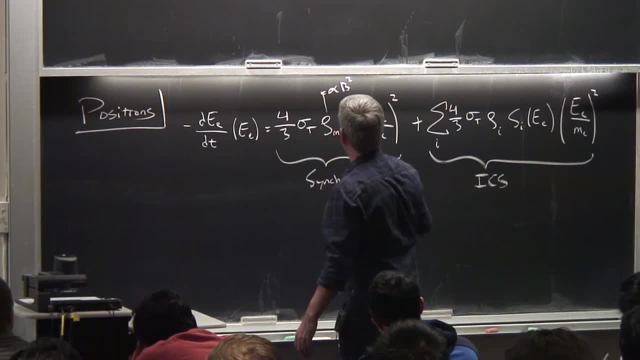 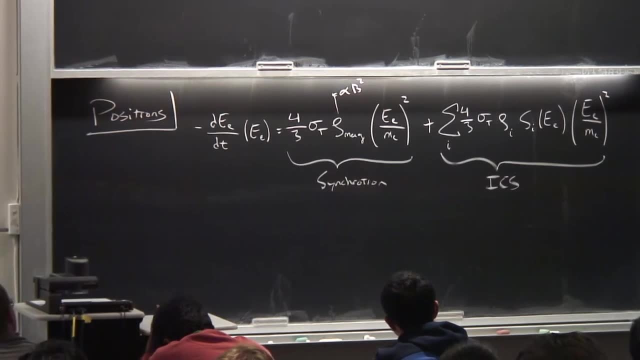 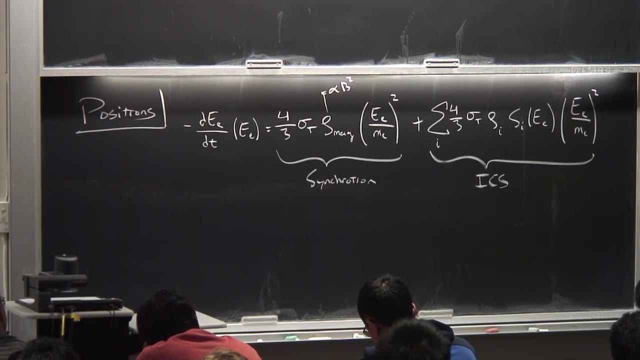 This is proportional to B squared, by the way, And this is just the You know Lorentz factor of the cosmic ray in question squared. The second term are energy losses from inverse Compton scattering. So again, what I mean by inverse Compton scattering is that cosmic ray electron comes along. 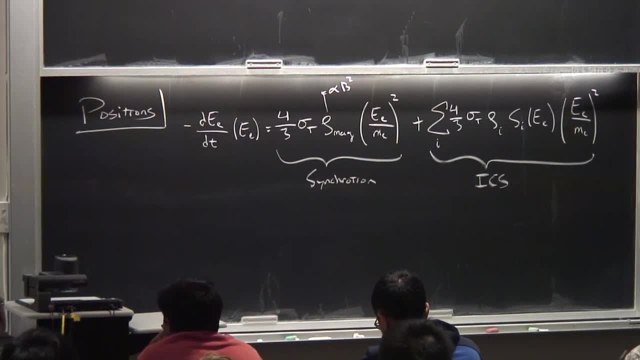 strikes a photon in the background, radiation transfers some or a lot of its energy to the photon and it repeats this process over and over again. What I'm summing over here are different radiation backgrounds, So obviously it's not as simple as a summation should be really an integral, integral over the the spectra. 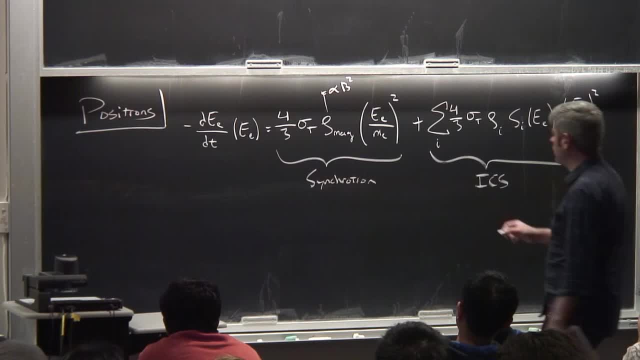 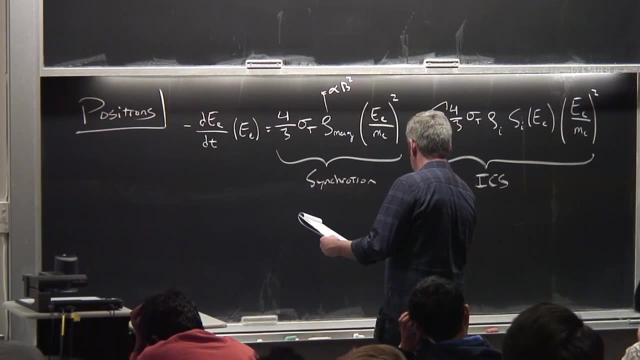 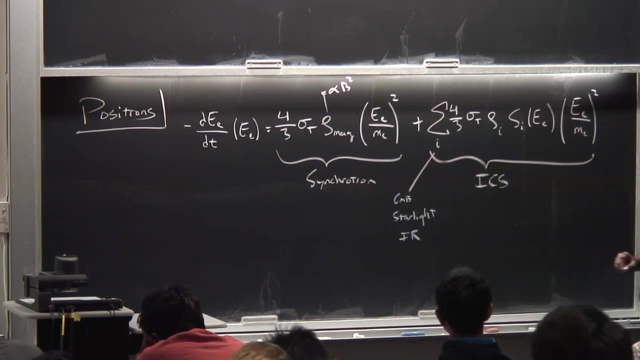 But for our purposes I think we can think of this as a few different components, So it can be the CMB, It could be starlight, It could be infrared backgrounds, and there are UV components too, but these are roughly the main pieces. 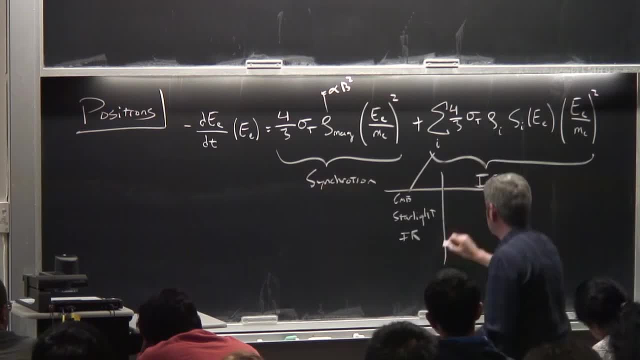 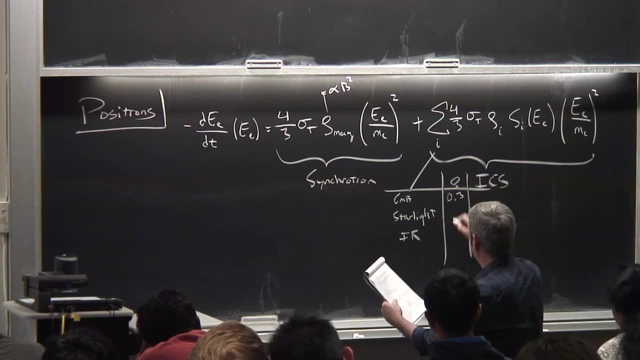 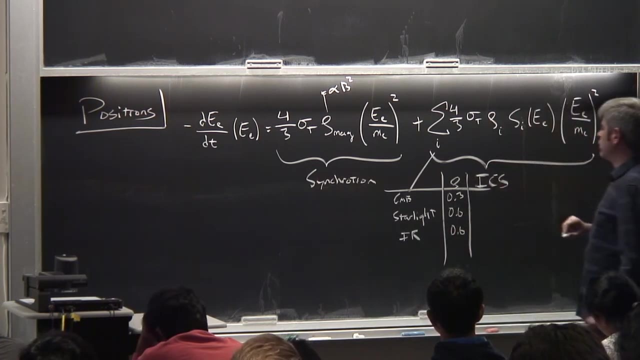 The energy densities in this are around 0.3, and these are in eV per cubic centimeter, and then 0.6 and 0.6.. So these, in terms of energy density, they're all comparable. This thing S of I is a suppression factor. 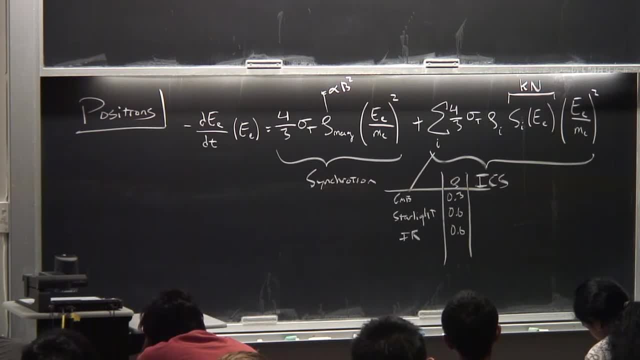 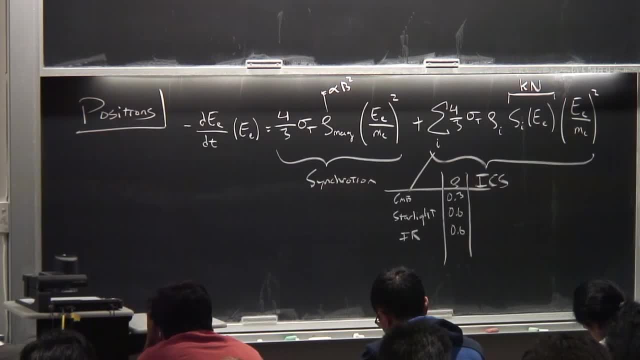 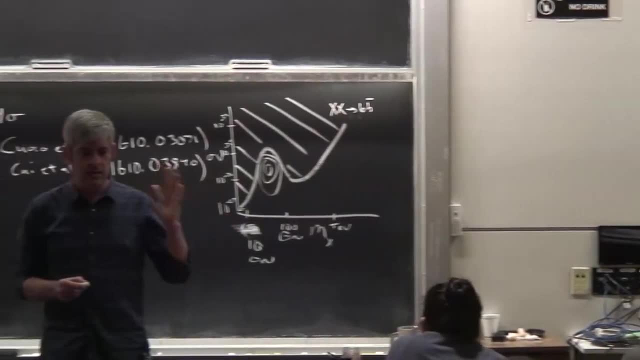 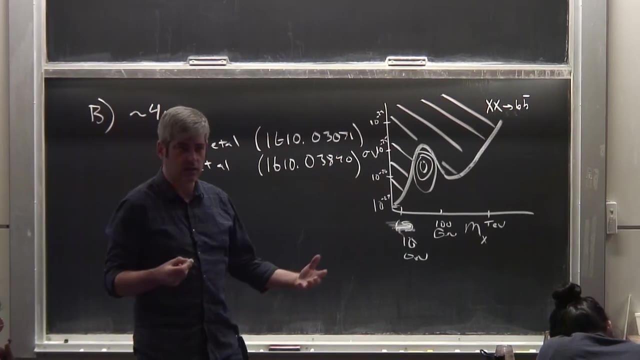 the E and M of this problem. you'll find that if you're scattering off of your cosmic ray and the target are sufficiently energetic, they do not scatter with the same kind of efficiency that you get in the low energy limit. I'm going to do this. 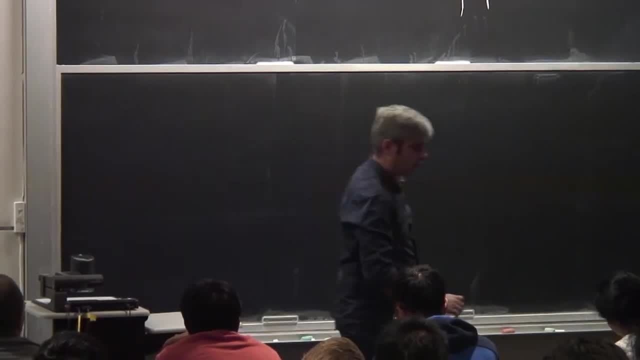 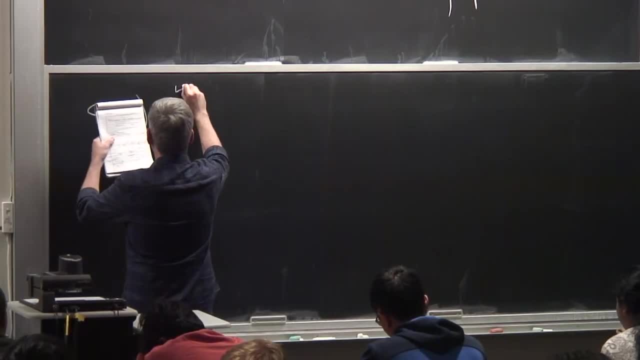 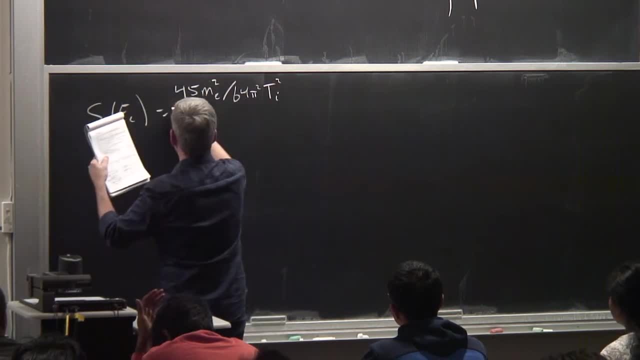 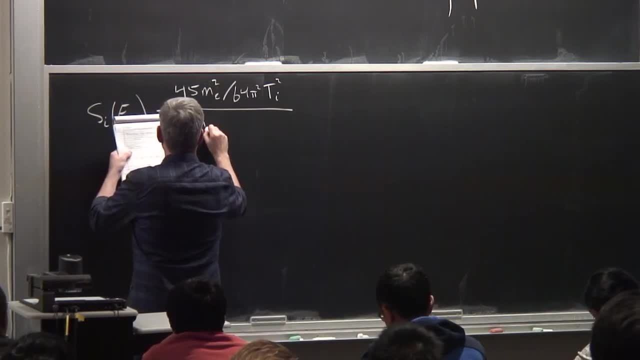 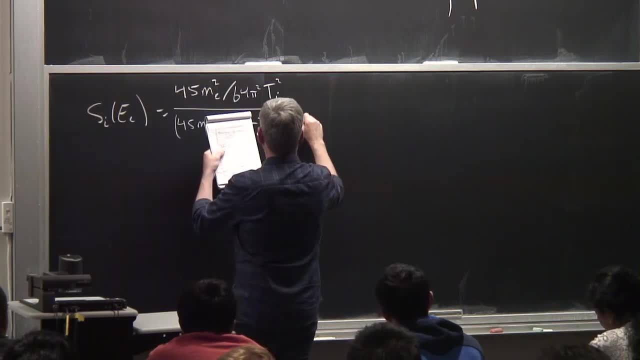 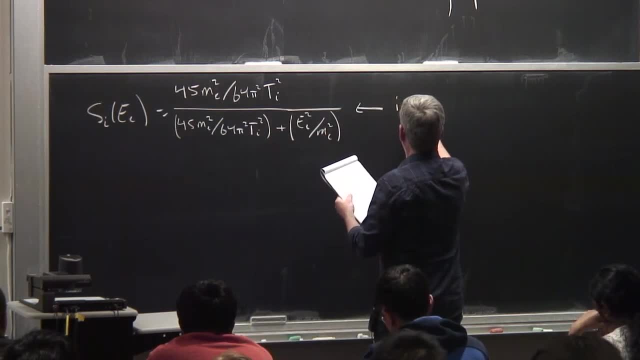 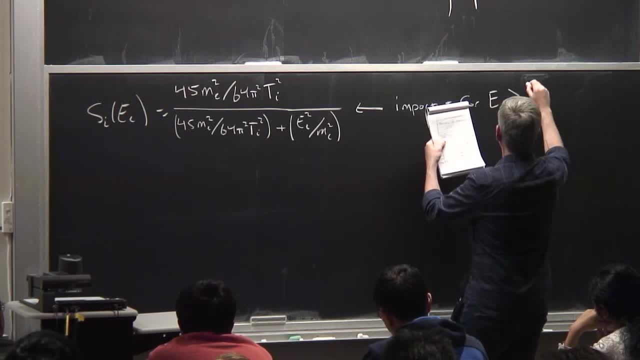 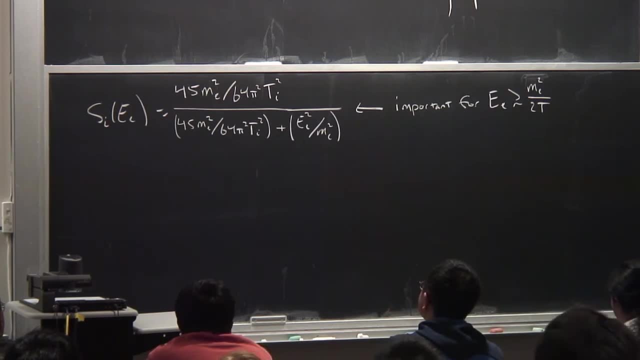 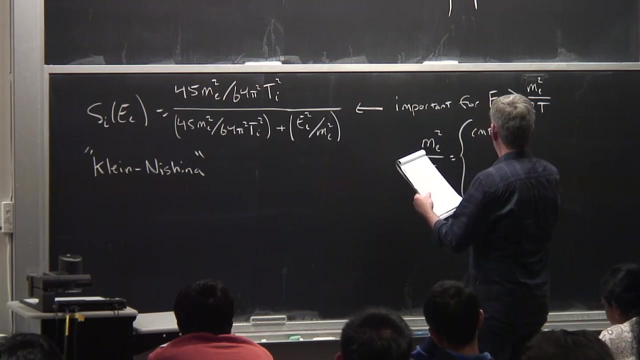 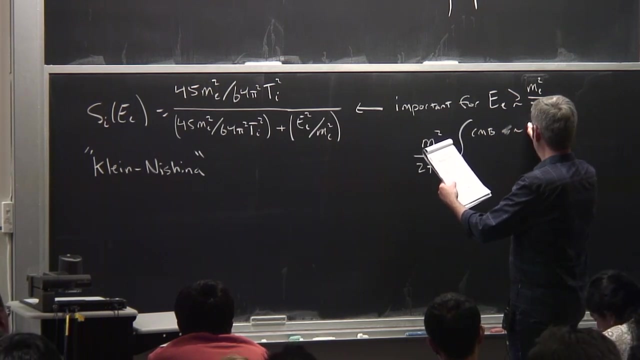 It will say when the energy of the electron in question is approximately equal to or greater than the mass of the electron squared over twice the temperature of the radiation component. So for the CMB turns out that this starts to kick in only at around 500 TeV. 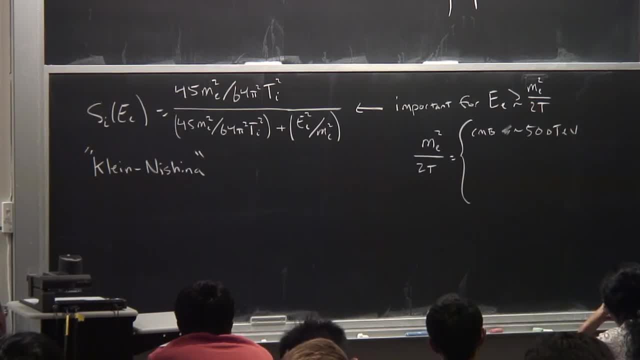 So for any electrons lower than 500 TeV, which are the only ones we're going to talk about, there isn't any Klein-Nashina suppression to speak of. For starlight, this kicks in at around 300 GeV, And that means this is important. 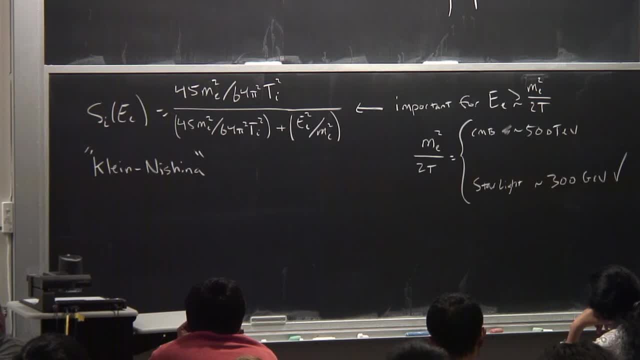 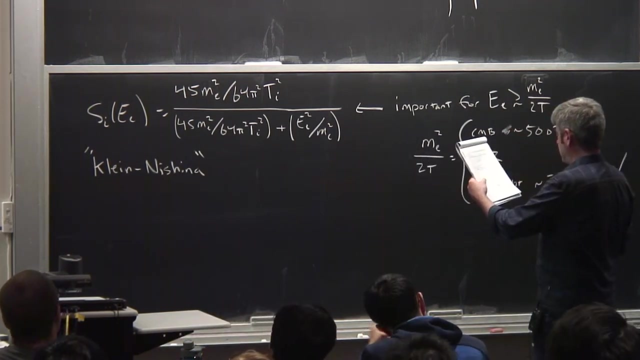 So we're definitely going to be interested in electrons around 300 GeV and more, And therefore you expect a transition From unsuppressed to suppressed scattering of starlight to occur in the measured range that we're dealing with, And in between we have the infrared stuff, which is around 70 TeV, which we can usually 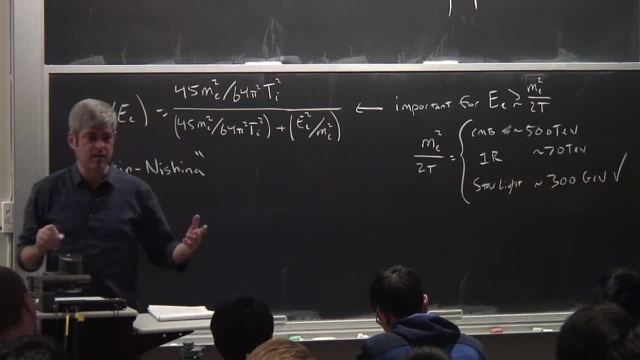 pretty much ignore. So it's really the starlight component that does interesting things in this kind of problem. Yeah, like I'm imagining a. So starlight is approximately described as a black body with a Several thousand degree temperature, right, I mean, that's that typical surface temperature of a star. 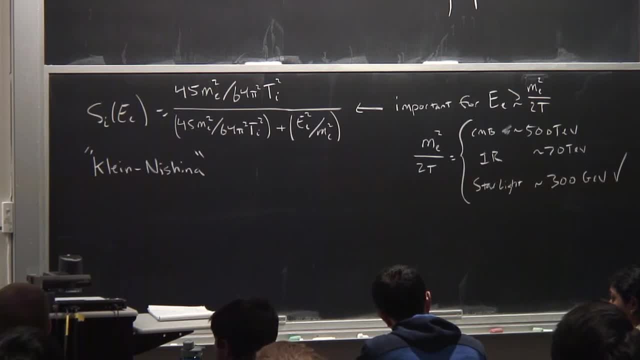 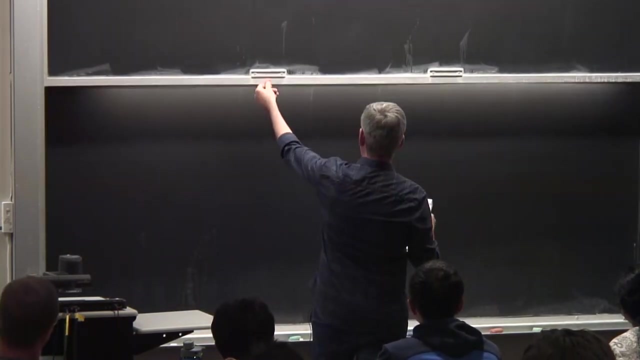 You can think of it that way. CMB is obviously a 2.7 Kelvin. whatever, it's a good way to think about this. All right, I'm running out of time, so I'm going to skip a few things. 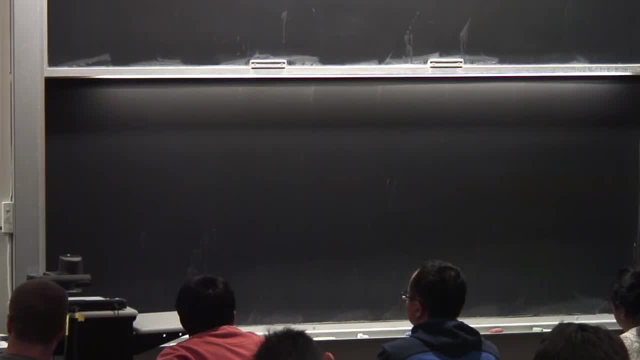 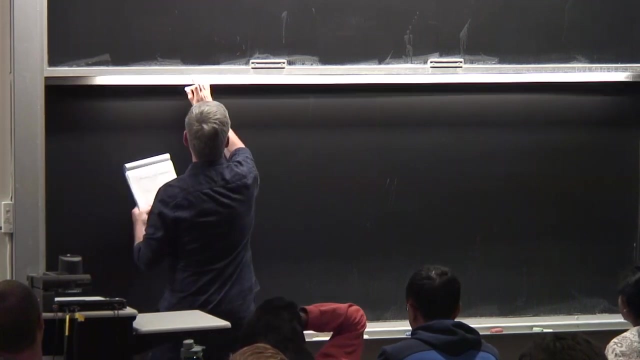 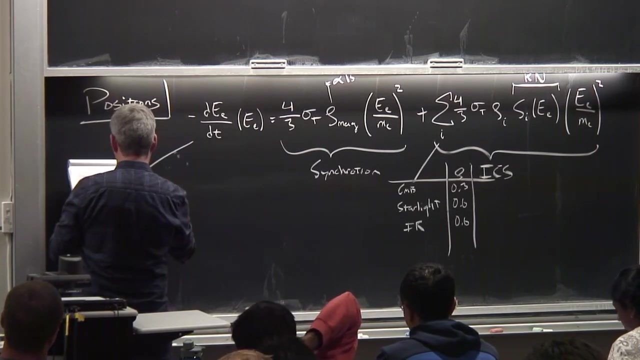 So let's consider an electron or positron that's dumped into the, Dropped into the halo and traveling around Because I said the Oh okay, sorry, I know I missed one step. This is important. If I put in reasonable numbers for these sorts of things, I find that the energy loss rate 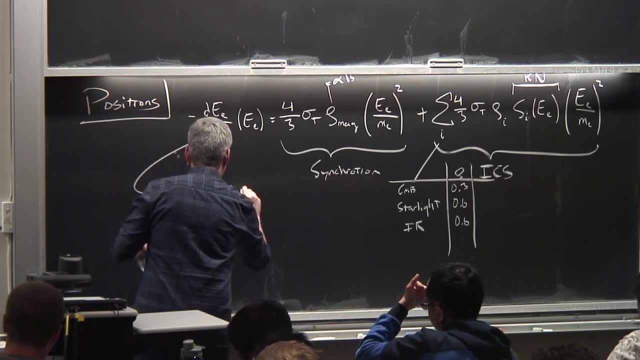 is about 10 to the minus 16 GeV per second. Right, Yeah, And you can see that it's a very I'm going to do this again. You need to be able to see this. You're going to have to be able to see this, but it's a very simple video. 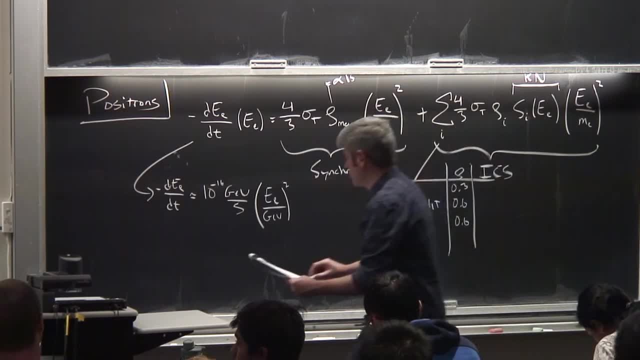 It's about the energy that's dropped into the halo. I haven't tried to draw the energy out of the halo right. It's a very simple idea And it's a very smart formula, So it looks like some sort of a? uh baki. 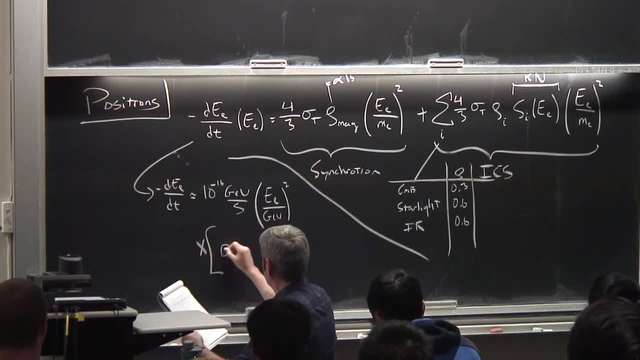 It's a very simple formula. It's kind of quite simple. If you we're going to săi say I'm going to try to say this, You're going to give me some real estate. so let's get to this. 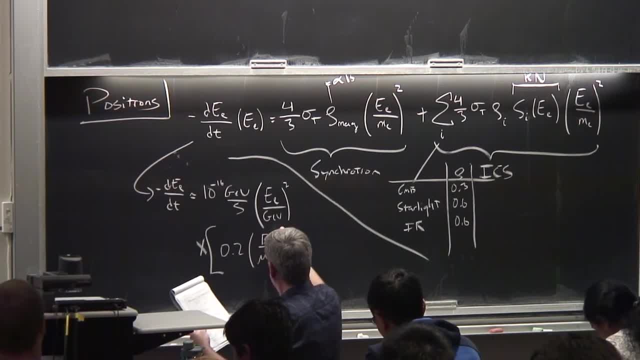 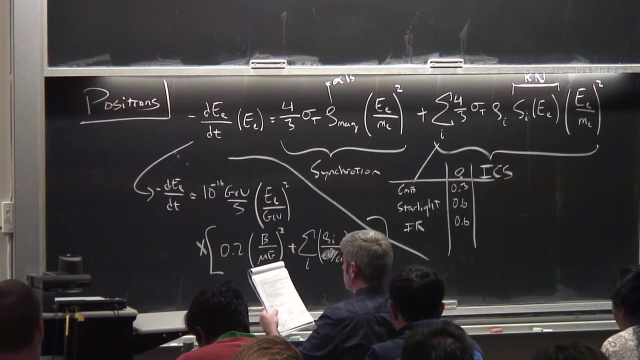 And you're going to see that the energy that's dropped into the halo, this is going to be 10 to the minus 16 GeV per second, this term and that term. So you can think of the thing in big brackets here as an order. 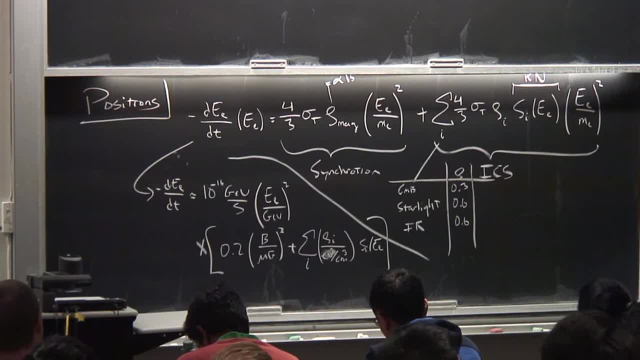 one factor, Say these things are going to lose at a GeV about 10 to the minus 16 GeV per second, which is a very slow rate. So 10 to the 16th seconds is tenth of the age of the universe or something. So you can immediately see that a GeV electron is not going to meaningfully. 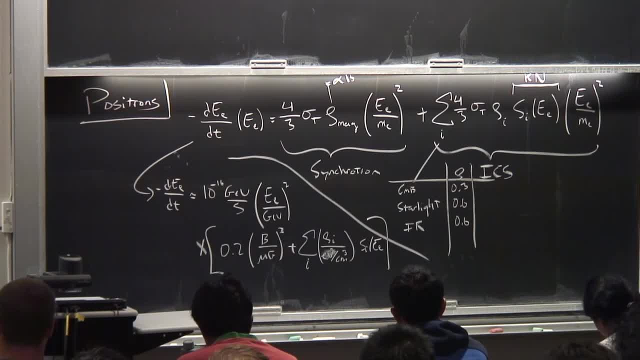 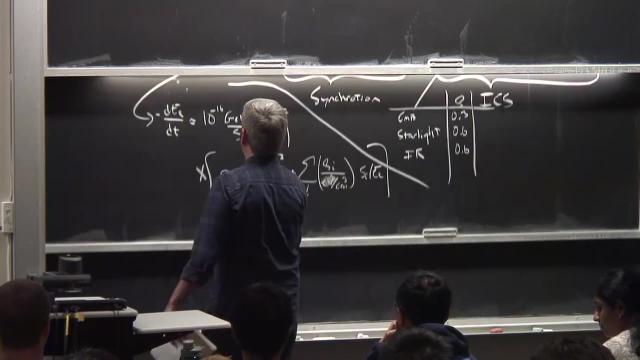 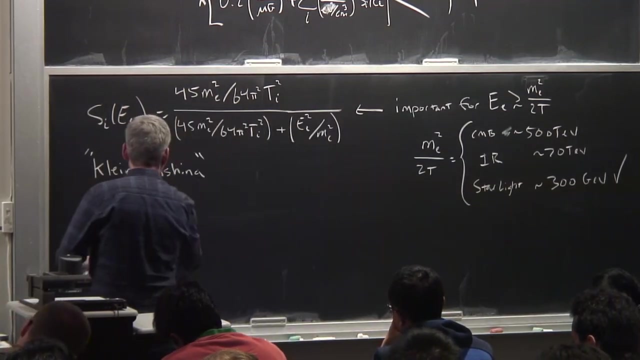 lose energy. However, a TeV electron now loses 10 to the minus 10 GeV per second, which is substantially faster, and that is actually quite important. So with that in mind, let's do a numerical estimate: The cooling time of an electron, meaning the energy, the time. 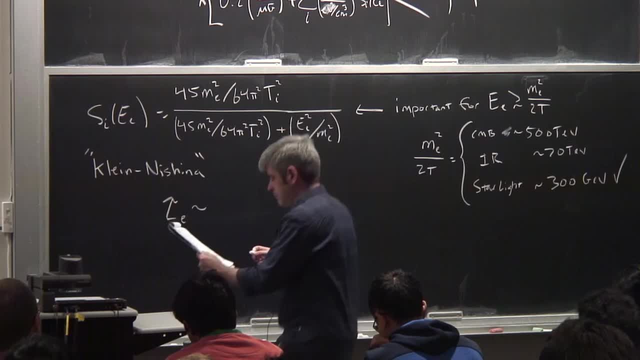 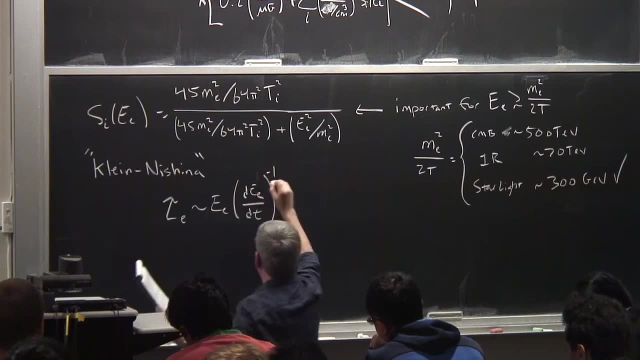 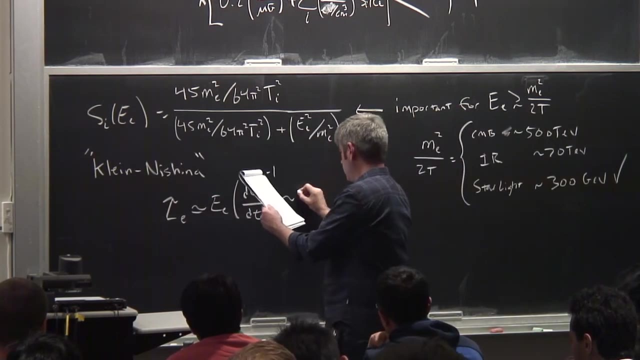 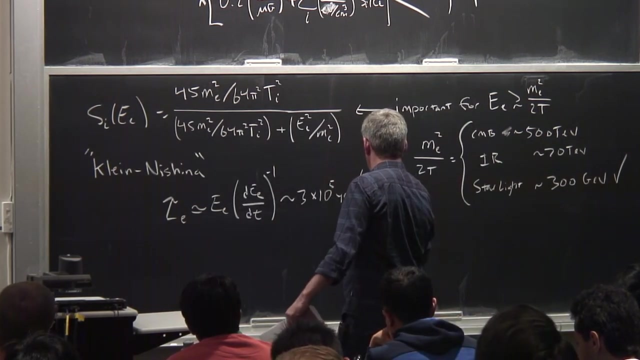 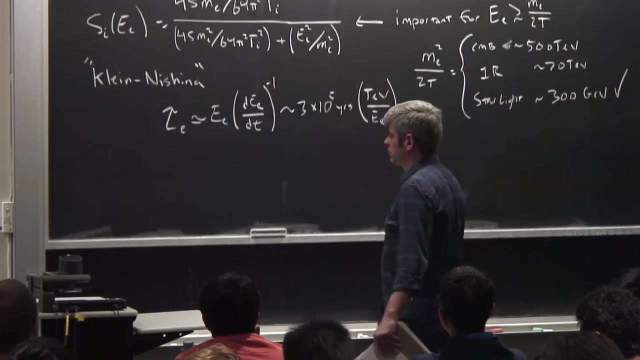 scale over which it loses an order, one fraction of its energy. I can define that. I can define as this: And the scale is like one over the energy. In this case it's about three times into the five years. And now we can take what we remembered from yesterday's. 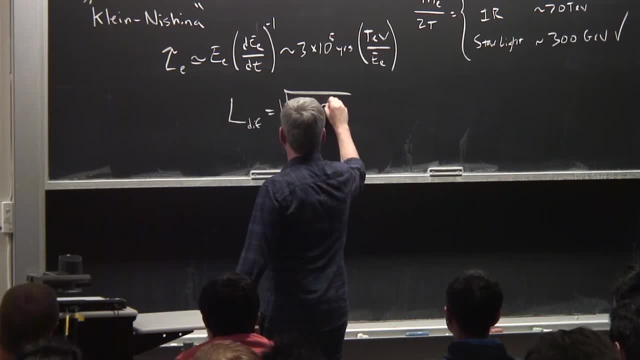 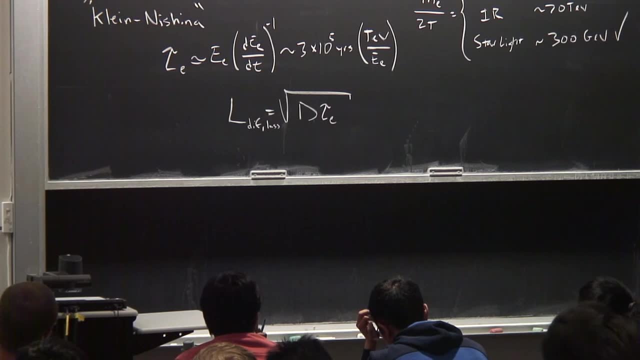 lecture and say that the length or distance scale that a typical electron will diffuse in a lost time. I can just put in for T the lost time here, tau, and I can put in the standard four times 10 to the 28th square centimeter, second times a TeV. 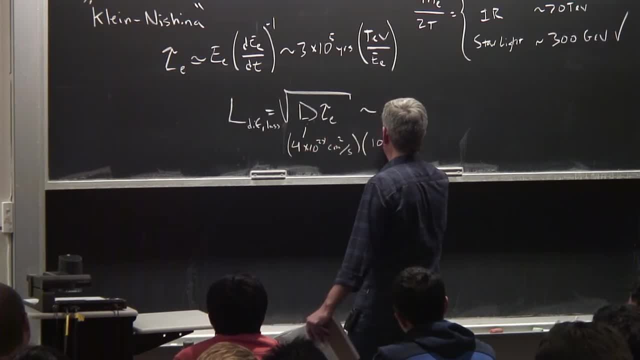 So I can put in the standard four times 10 to the 28th square centimeter second times a TeV. So I can put in the standard four times 10 to the 28th square centimeter second times a TeV. I can also put in for the T to the 28th square centimeter second to the 28th square centimeter. 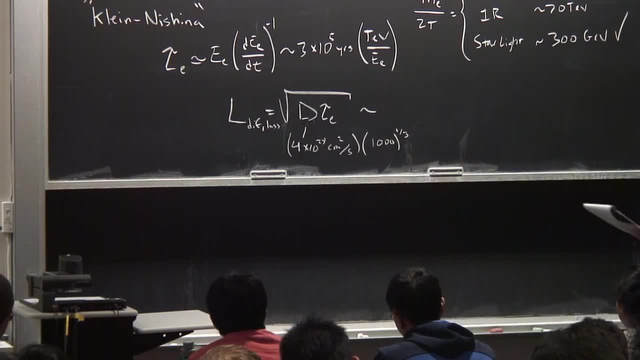 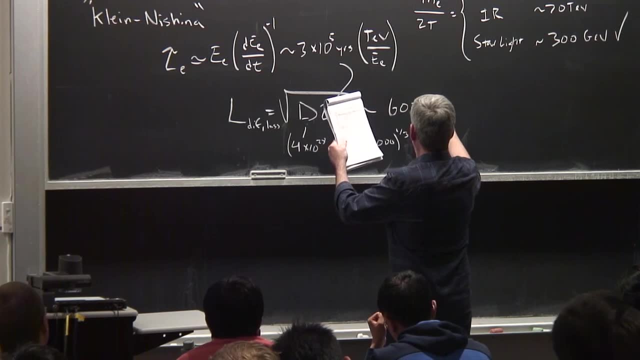 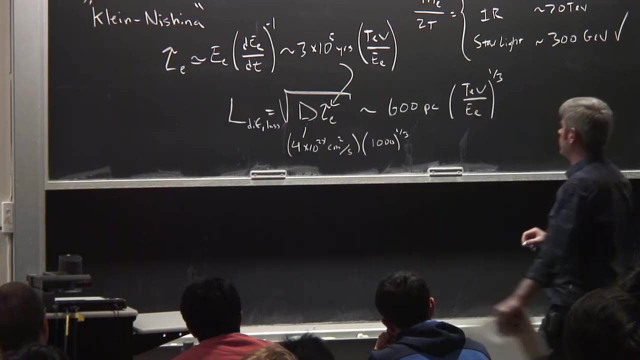 second times a T to the 28th square centimeter second. That's what my Born-to-Carbon and other fit tells me And I can put this in for here, And I get a number which is about 600 parsecs for a TeV electron. 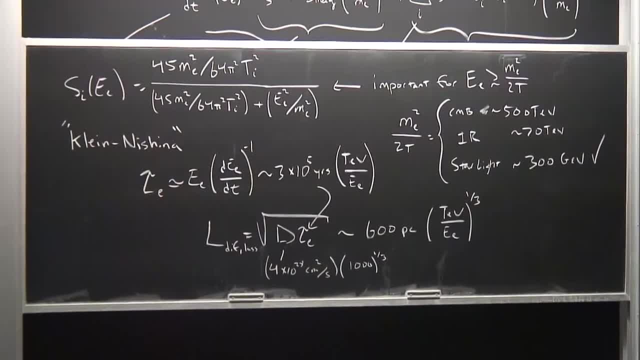 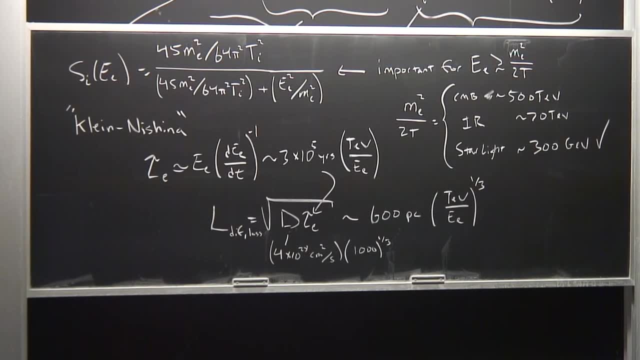 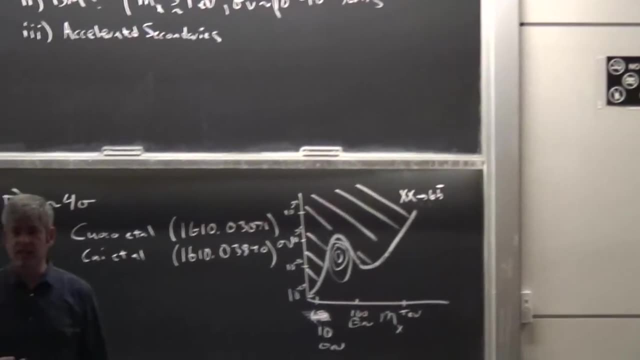 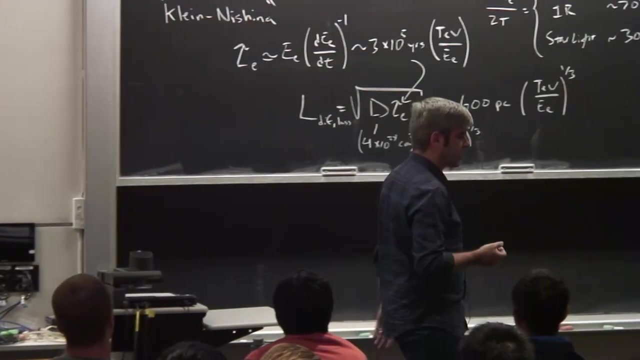 This is pretty local. So at a GeV I am sampling electrons and positrons that are produced in several kiloparsecs in all directions. A substantial fraction of the galaxy contributes at a GeV. By the time I get to a TeV I'm really looking at a very small sub-kiloparsec region There. 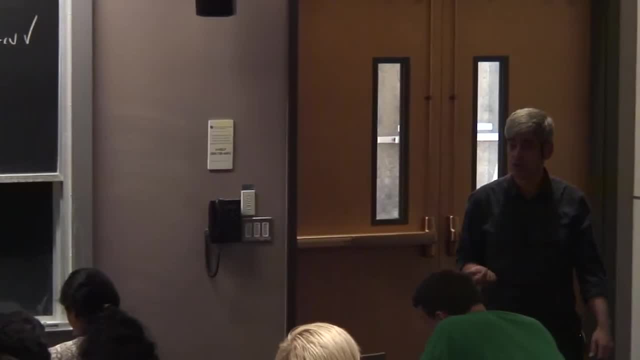 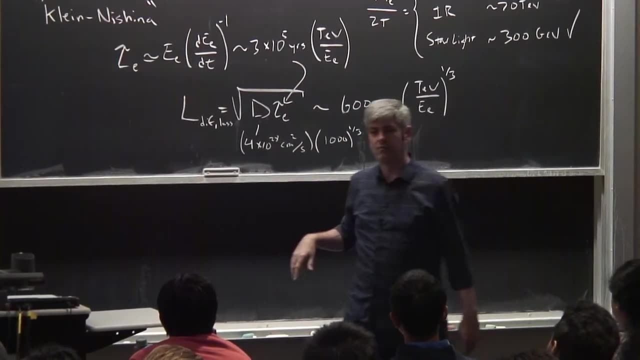 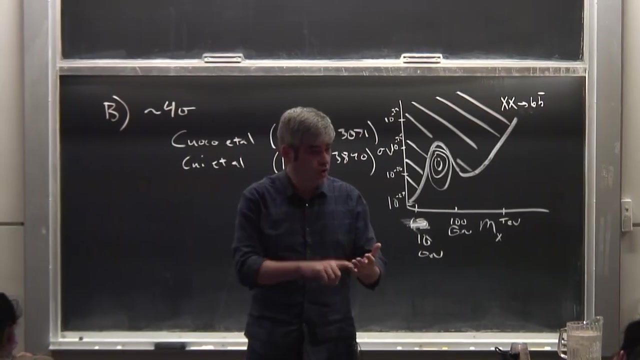 are not many sources- plausible sources- of cosmic rays in that region. Also, I'm looking at a very small piece of time, I'm looking at only a few hundred thousand years, And that means I'm only looking at cosmic ray sources that contributed locally and recently. That's a very special kind of source. There are not, for example, supernova remnants that meet these criteria. There are some pulsars. They are probably primarily responsible for this. just when we did the boron to carbon stuff, you found that this quantity is. 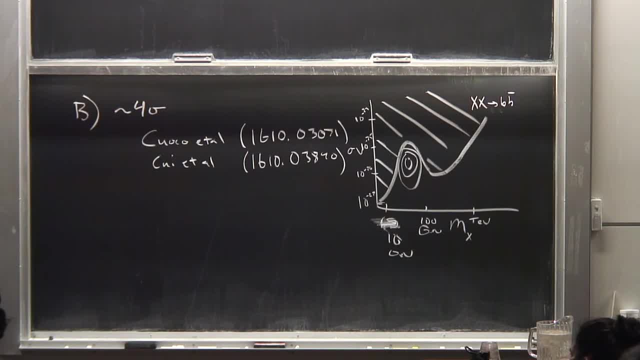 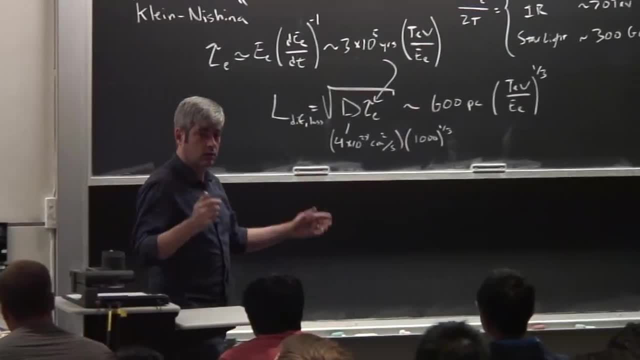 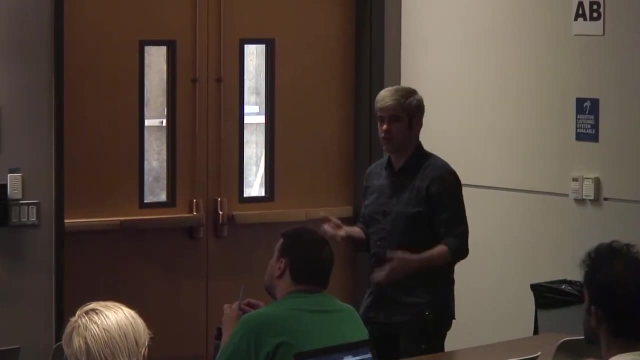 constrained to have this coefficient of two times or four times to the 28, and has an energy dependence which is about e to the third. that's, that's just a fit to the data. however, theorists who work on turbulence and stuff call this the Kolmogorov spectrum of inhomogeneities, and that, in fact, is long been. 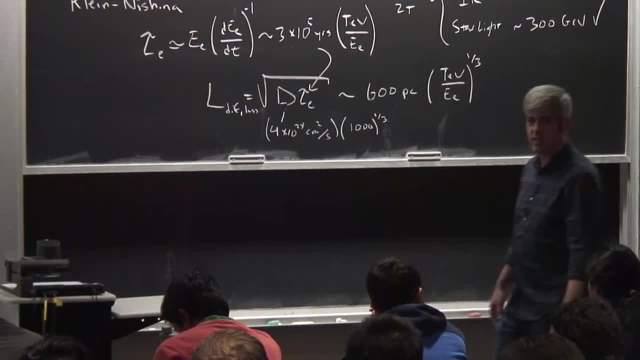 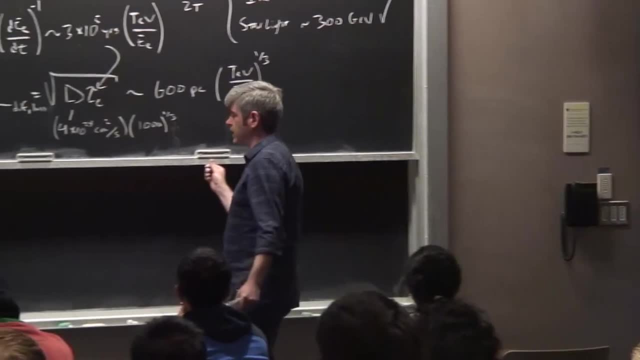 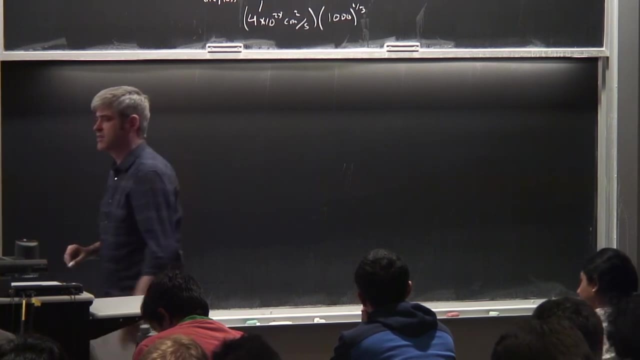 predicted, so it matches with theory pretty well. that being said, I was entirely agnostic until it was measured about that choice. all right, so let me draw the data now and we can talk about what it might mean. so in antiprotons they talk about the antiproton to proton ratio. for some reason we do it a little. 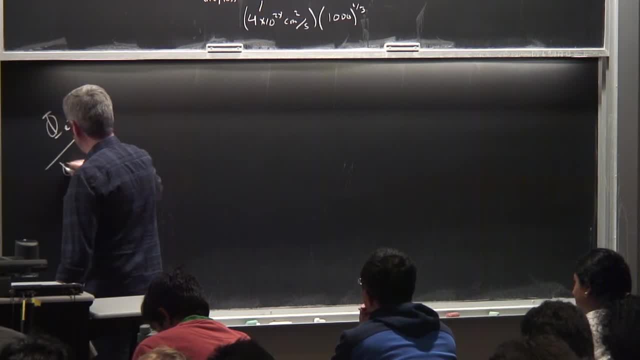 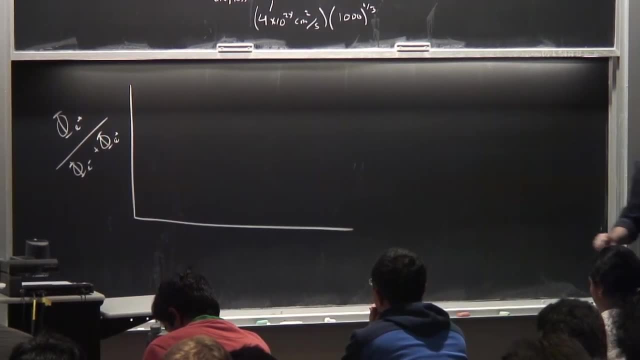 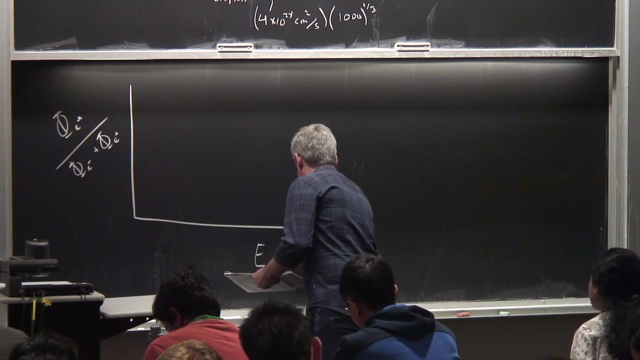 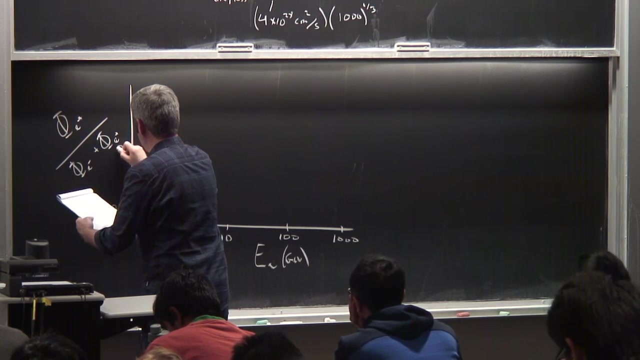 bit different and when we're talking about positrons, we talk about the positron fraction, which is the ratio of flux of positrons to positrons and electrons. so it's a fraction of positrons and electrons that are positrons. okay, and because it's easier, 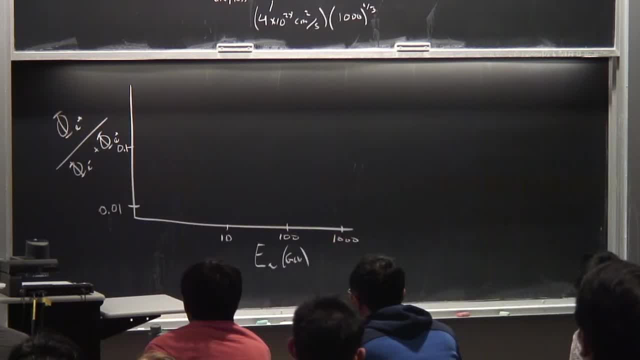 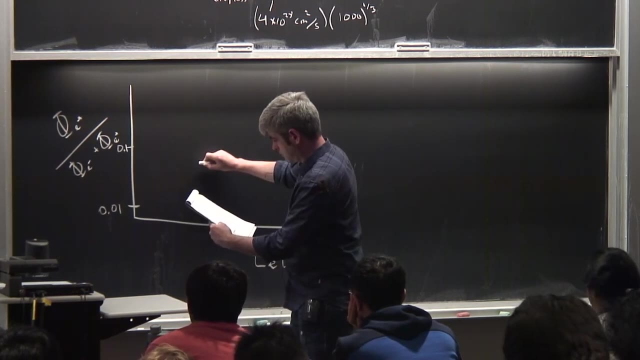 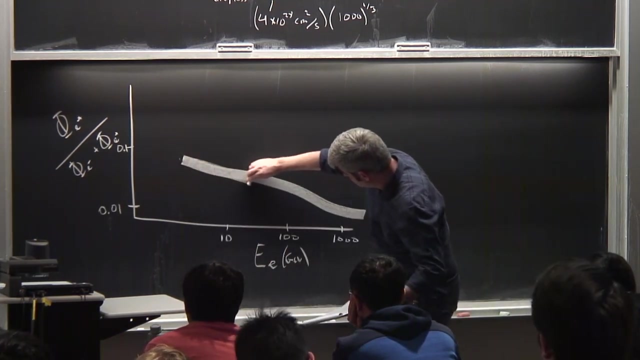 to make positrons and antiprotons. the rate- the numbers here are much higher than in the ratio of of antiprotons. but what we had expected this to look electron, what we had expected this to look like is something like this: there, that's not a wiggle, that's just me not drawing. well, that was the expectation of. 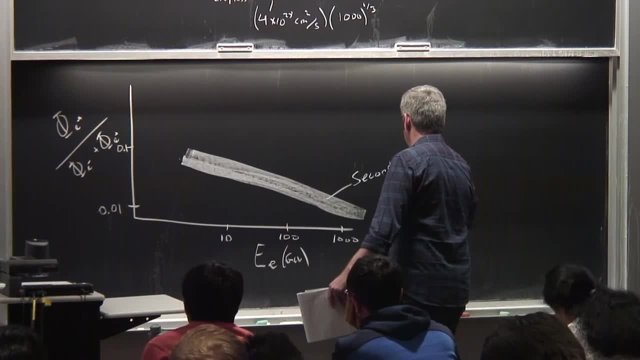 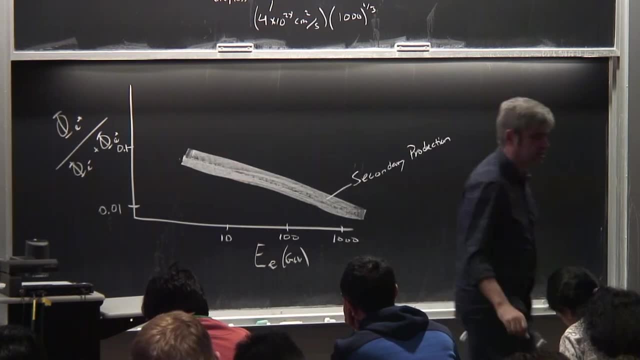 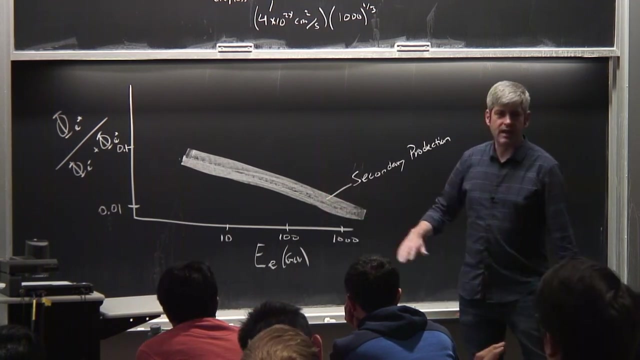 that was the expectation of the and down here at low energies, there were all sorts of reasons to think we might have the secondary prediction a little bit wrong. after all, you're sampling a huge amount of the galaxy, places you don't know much about, but up here you're sampling the local, the local Milky Way. we know a lot about that and I don't see any way that the secondary production could be very different up here. 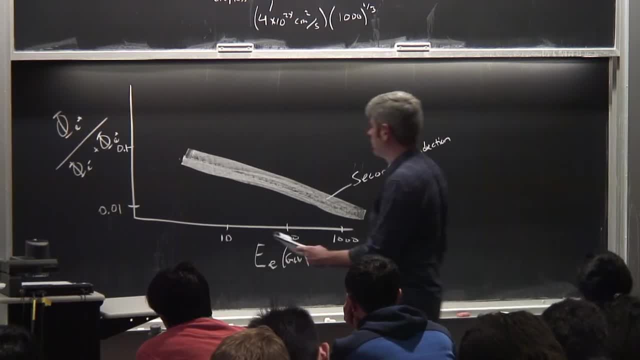 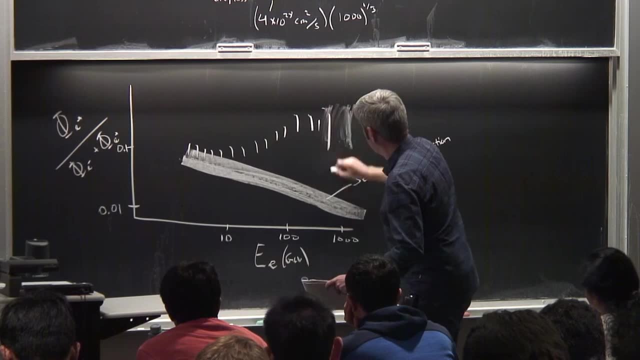 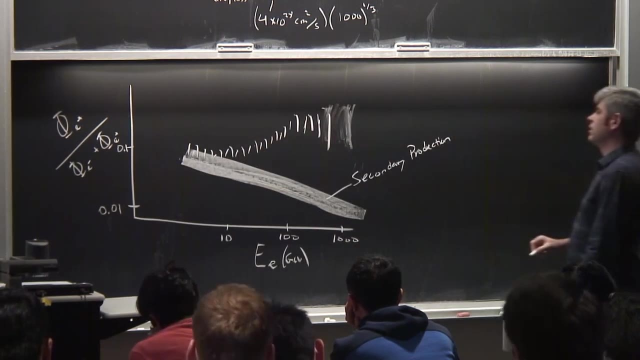 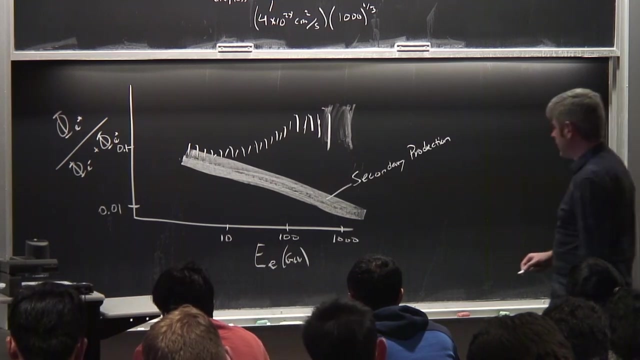 and I don't see any way that the secondary production could be very different up here. and then here's what we measure: something like this: I drew this like that. okay, nothing at all like what was predicted. there is some. I think it's is totally un-controversial now to say that. 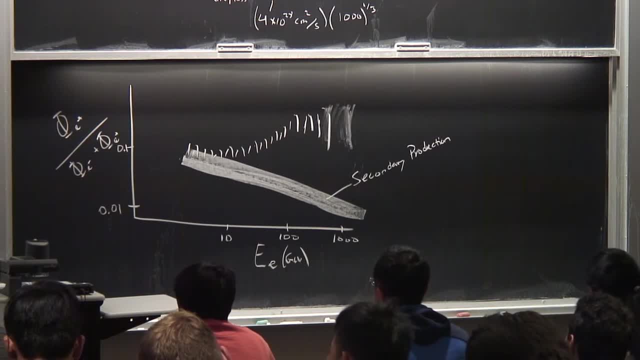 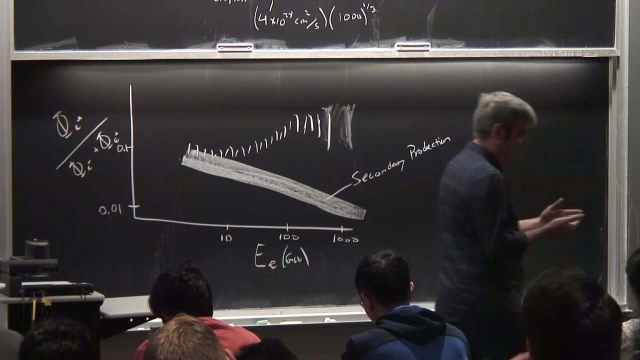 there's A-nutrキust, are more significant sources of primary positrons in the local part of the Milky Way. So the positron spectrum is not dominated by secondaries, as we had long imagined it would be. Instead, it is overwhelmingly dominated, at least at high energies, by something dumping very high. 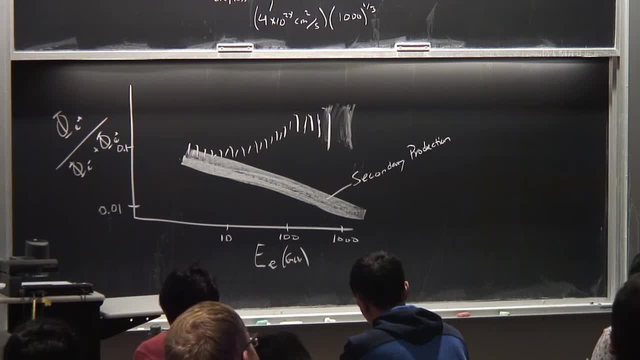 energy plus and minus pairs into the local environment. So obviously, being dark matter hunters, we got very excited about this. This is AMS data I'm plotting here, but there were hints of this for a long time Back when I was a student at TOSI. we were already then. 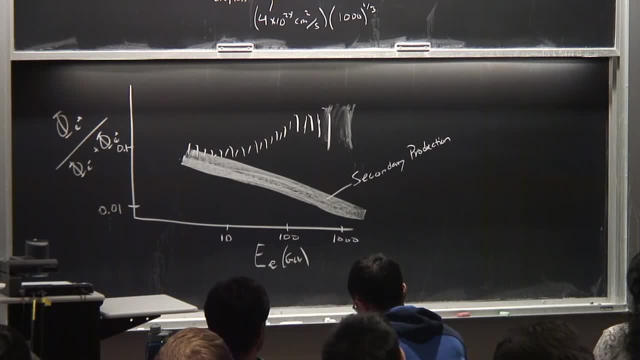 talking about something called the heat excess, which was a series of balloon flights that saw some hints that they had one bin here that was above the prediction. That was what we were running off of, And then Pamella was the first satellite to do this sort of thing. 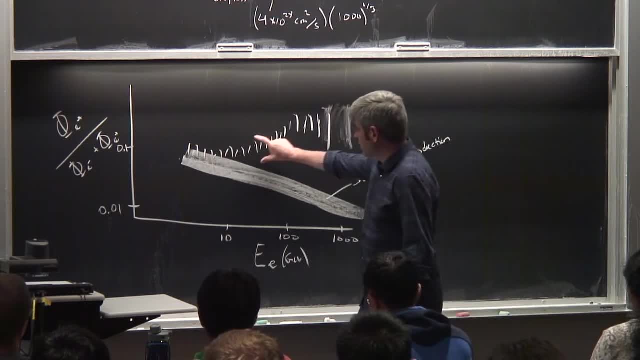 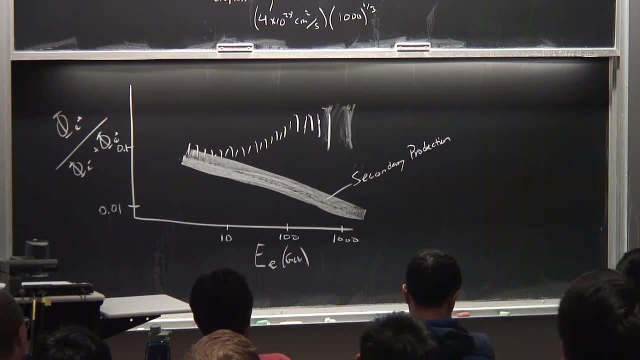 measured very clearly That this was climbing with bigger air bars than this, but clearly climbing up to a hundred or so GV. And then AMS came, made all those air bars really, really tiny and extended it up to, I don't know, 600 GV or something I think is our highest energy bin right now. It made it just abundantly clear that this was real. But every step along the way it made it harder to fit to annihilating dark matter scenarios, or decaying, for that matter. Back when you had the heat excess you could do this with, like your favorite off-the-shelf. 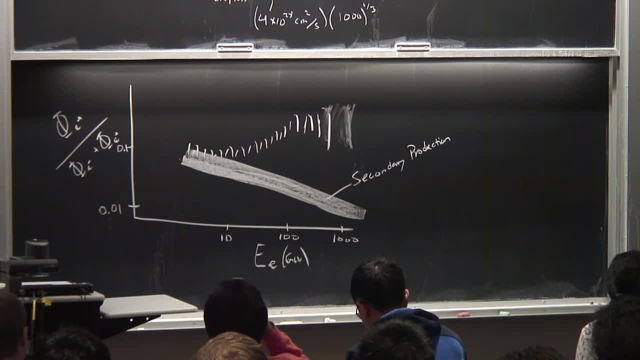 SUSY model. It wasn't hard at all. You wrote down 100 GV, WIMP, the thermal cross-section, have it, annihilate the Ws and bam, you got the heat excess. It was great. Then Pamella came along. We measured the spectrum pretty well. There were a flood of papers. 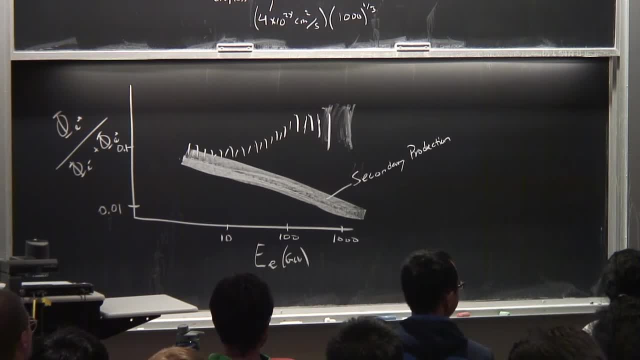 The first Pamella data. you could try to squint and make it look like something like a SUSY WIMP could work, But a little later on it knew some Fermi data came into bear and you just couldn't. You had to play with like leptophilic models where you're annihilating a lot to things. 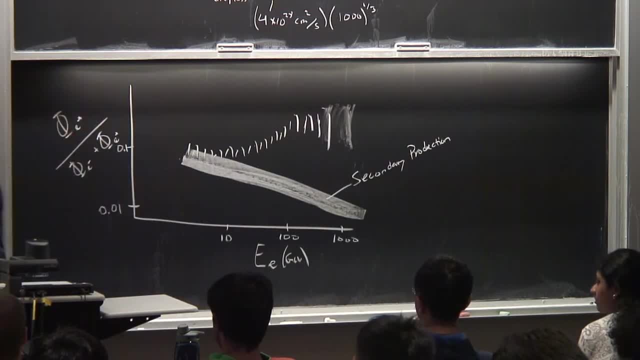 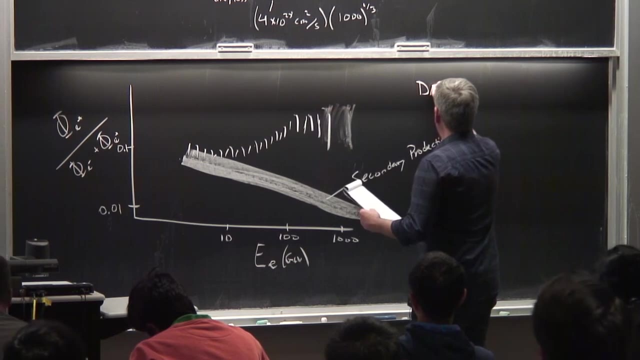 like muons, But you could do it. And then AMS came along and it was just much, much, much harder. There is a class of models that can probably well that in fact can- fit the data, the modern set of data that is. So if I want to interpret this as dark matter, what I roughly need is 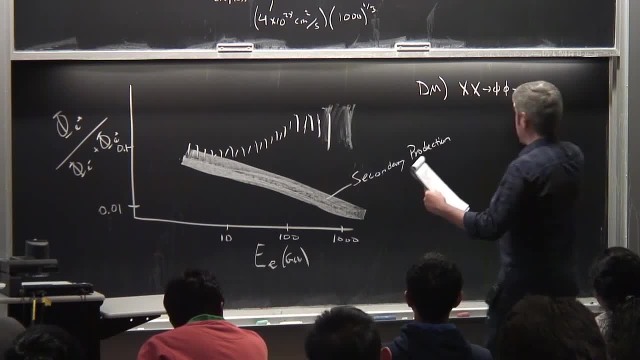 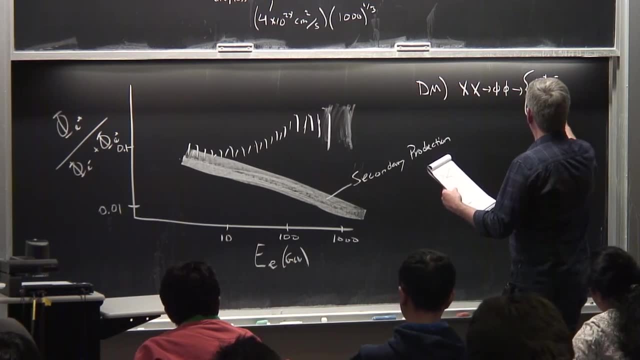 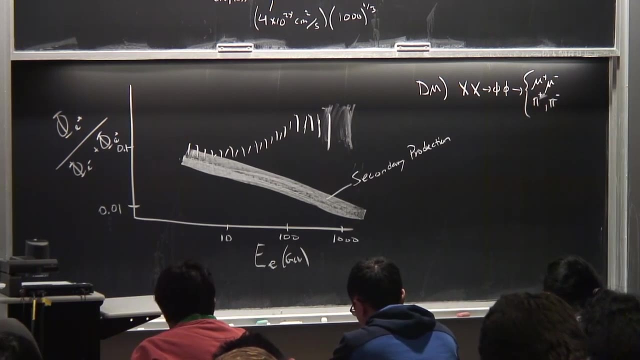 dark matter that's going to annihilate to some sort of intermediate unstable state, which then decays. At face value, a cross-section this big would be ruled out by Fermi data. but the people who try to save it do things like making sure that there are big flat cores in the several kiloparsecs around the galactic center and things like this. 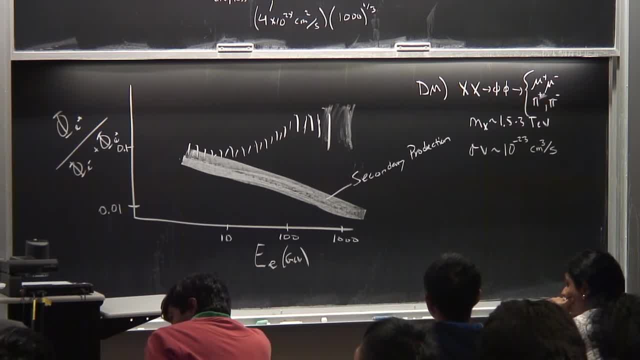 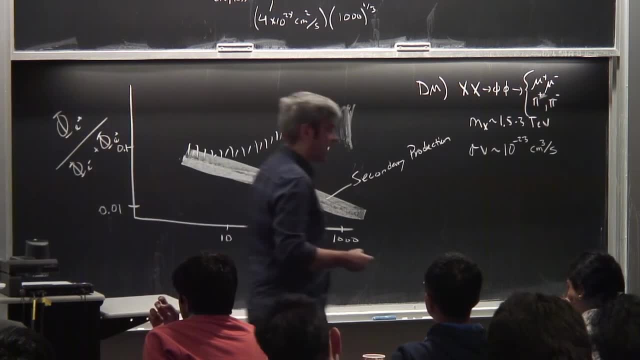 So if you're willing to put a lot of freedom in things like this, you can just barely make this work today. But interest in dark matter- interpretations for this excess- have declined dramatically as a result of it being harder and harder and harder to fit the data in this class of. 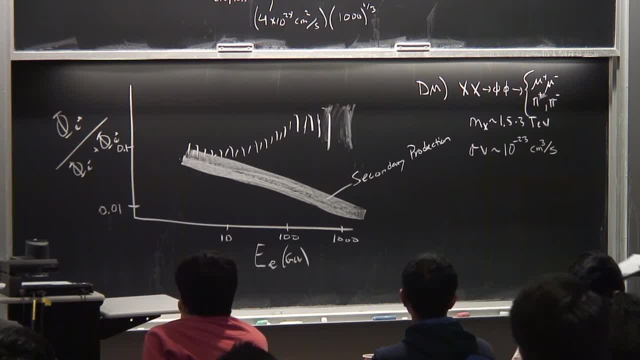 models. There are a couple of caveats. I want to mention other ways that you could try to explain this with dark matter. So when I say that this is the sort of candidate you need to explain this, it's assuming that the dark matter is distributed roughly, like an NLW-like profile. 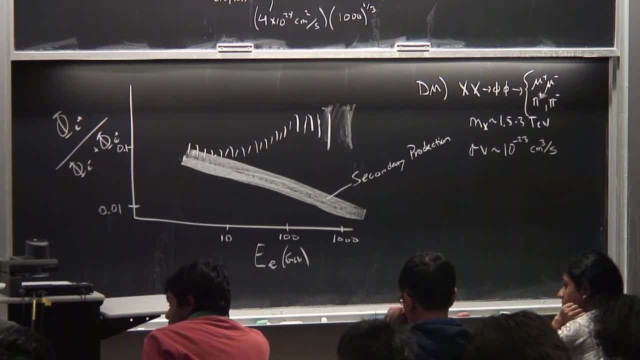 But we have every reason to think. dark matter also takes the form of clumps, Subhalos and things like this, And maybe one of those just happens to be really nearby us and it's annihilating like mad. That's the sort of thing that could dramatically change these sorts of calculations, both in 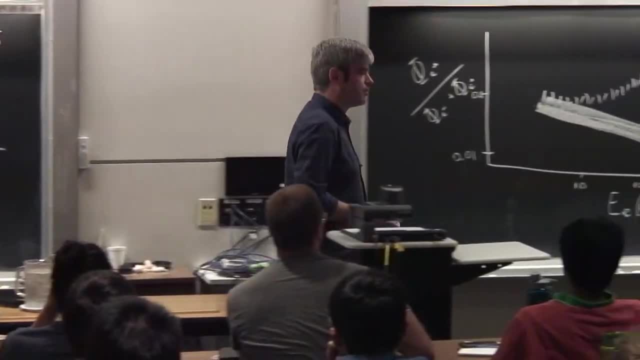 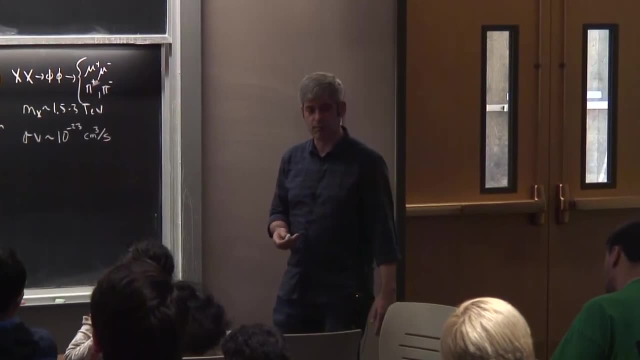 terms of spectral shape and in terms of the required cross-section. So once you do stuff like that, you're more free to consider a wider range of models. But then you should also ask yourself why Fermi doesn't see a big, you know bright. 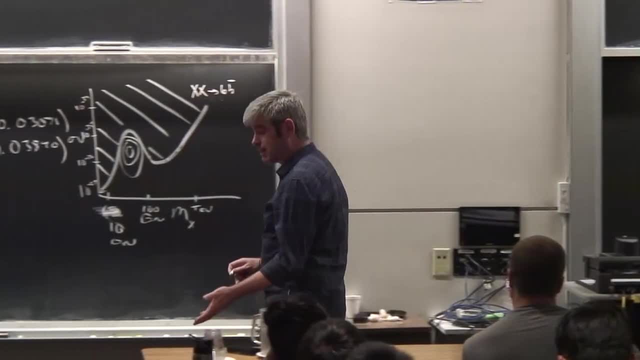 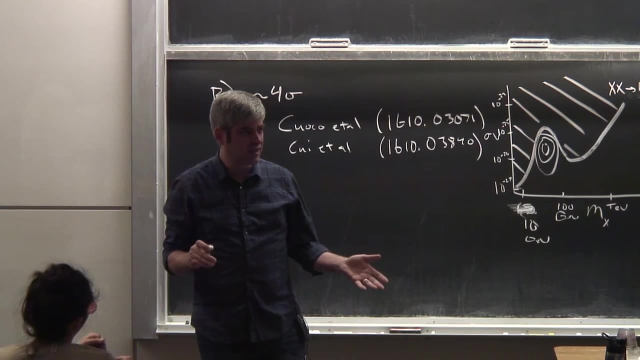 blob of gamma rays coming from wherever the subhalo is. If you want to really play games, you put that blob that just coincidentally in line of sight with a big bright gamma ray source like Vela, So it conceals it. 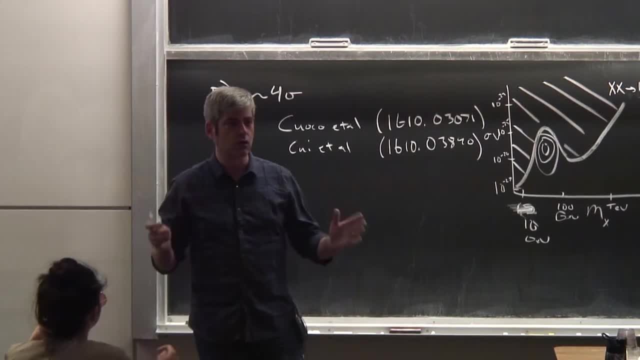 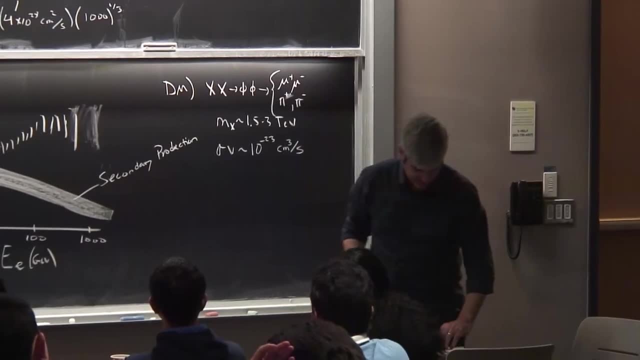 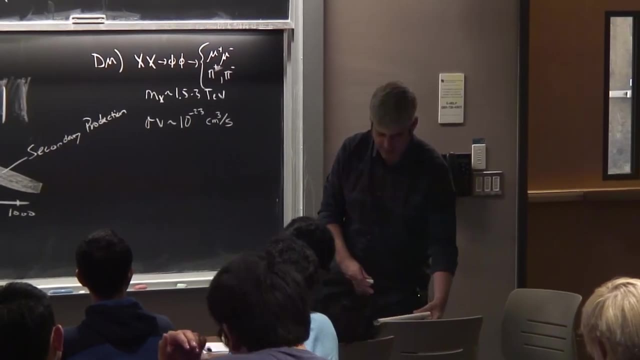 But you know, there's what you can do and what you can tastefully do, which is kind of drawing the line here. Yeah, that's my next pages. Well, it's my second to next pages. I'll come back to that. 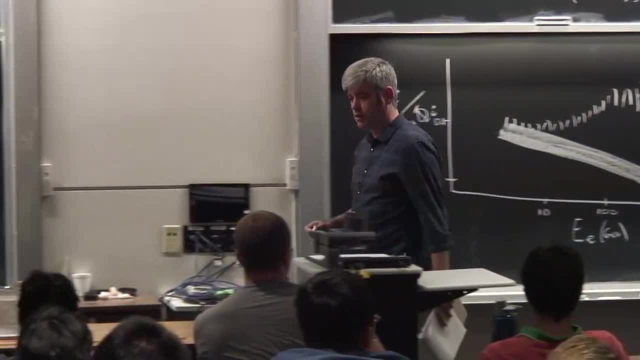 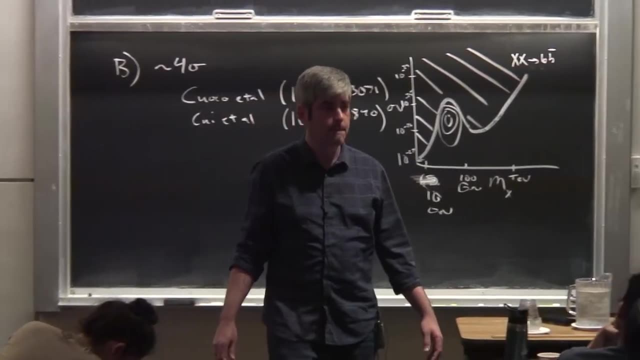 Okay, Sorry, Yeah. So all of this is because, I mean, it's a part of the question that this is very high energy, which means it's very local, and we understand it very well. The fact that it's very local depends on the diffusion length, which depends on the 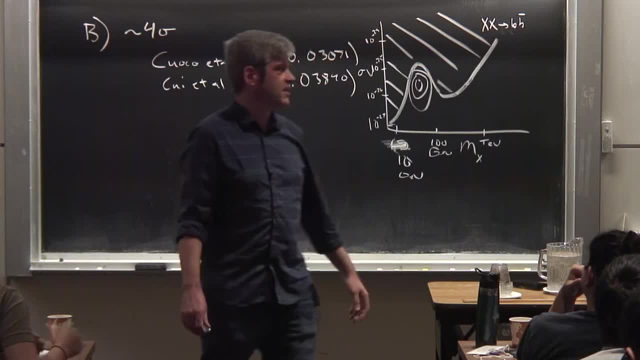 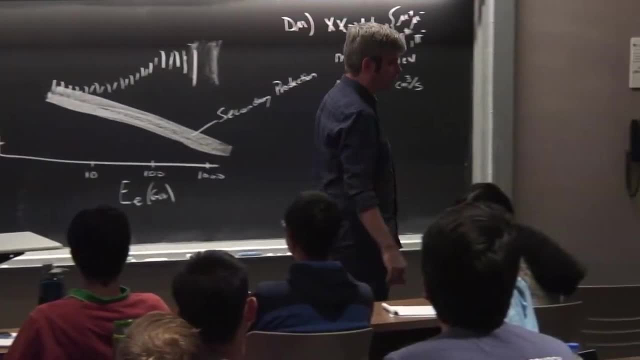 and that was spherical cow It's. Are we sure that DE is really supposed to be in our relationship with it? So this, this cow, this spherical cow, is a describing a cow that is not very depart, not very non-spherical. 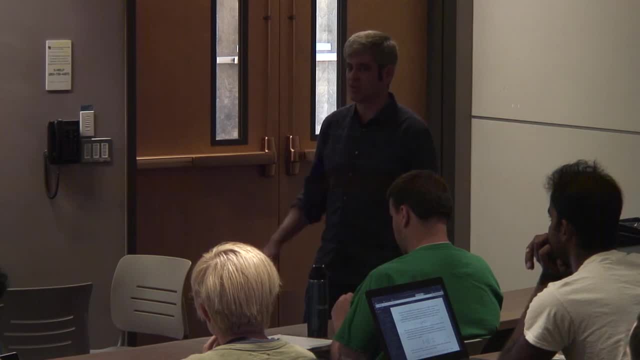 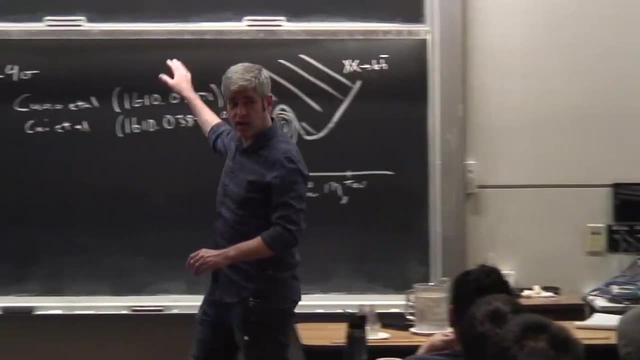 Okay, The cow that is causing the propagation is pretty close to the spherical cow we're talking about. So when I talk about the, the AMS thing or the sorry the AMS anti-proton thing and you get like small departures here and there, I'm totally willing to imagine that that has. 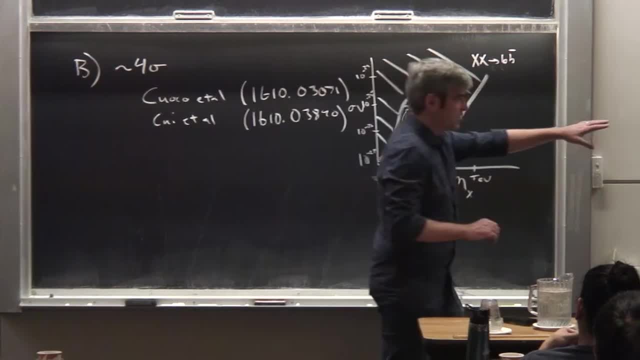 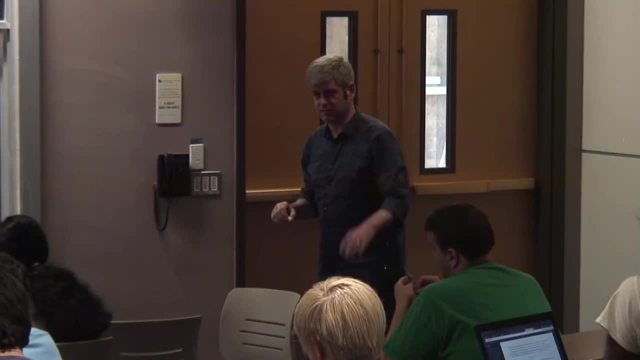 to do with failures in our diffusion model or our transport model, But when you're talking about being off by an order of magnitude and a really well understood regime. no, no, no, not even close. I, I, you know, people have tried it. 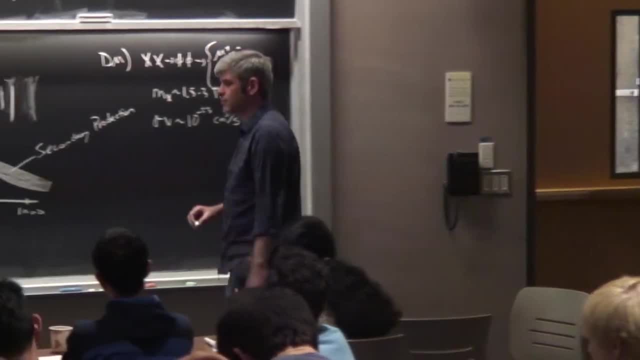 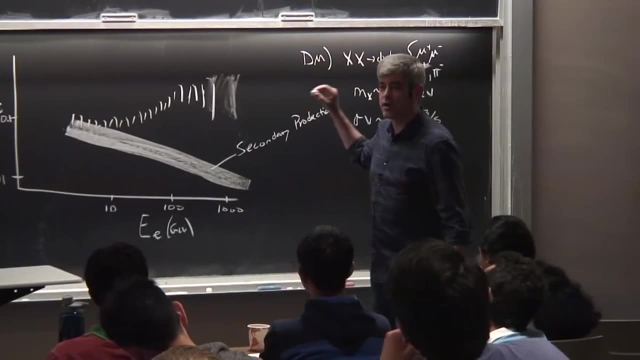 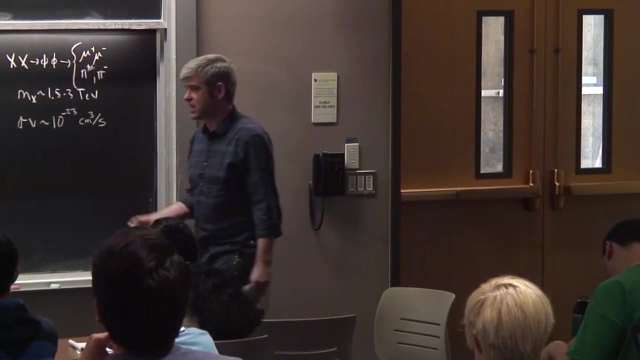 Not even close, Not even close, Okay. So, because there is a huge excess over background, it makes it hard to use the AMS positron data to constrain dark matter, Okay. So when, when you already see 10 times more than you expected you, you get very, very 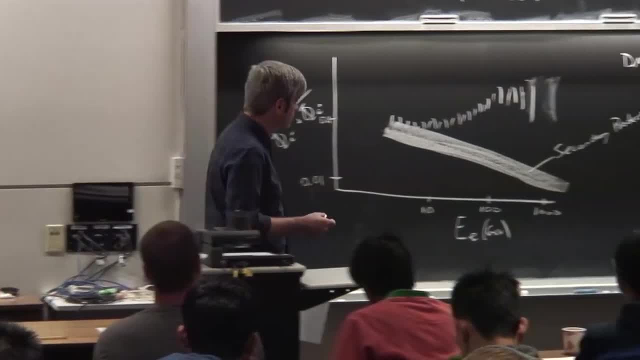 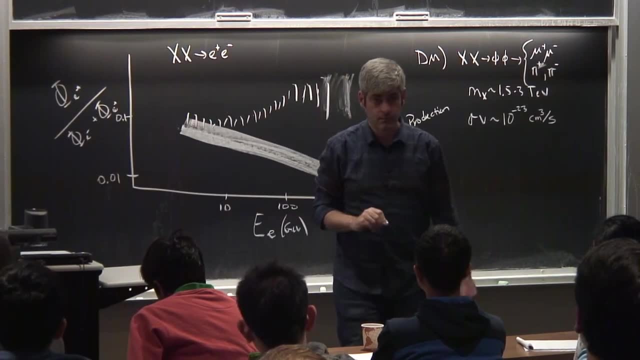 weak constraints on dark matter. There is an exception, though, and that's that if I have, for example, just imagine I had- dark matter that annihilates the E plus, E minus directly. That means that some mass let's- let's just say it's here in 100 GV I'll get a delta. 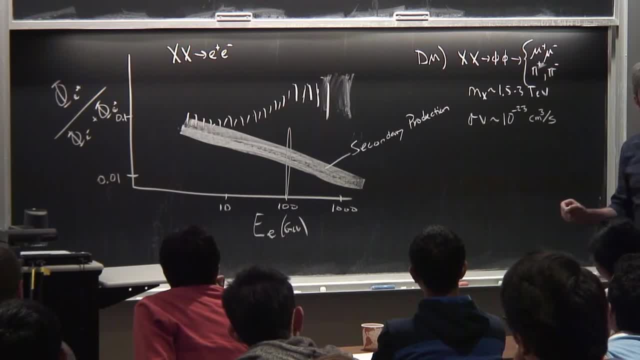 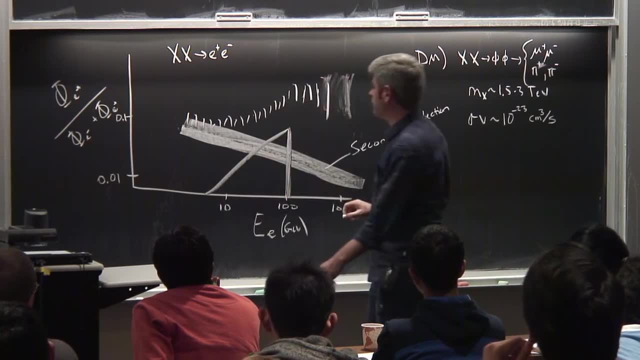 function injected. Of course, it doesn't look like that when it reaches us, because those particles lose energy steadily as they propagate. So what you wind up with is an edge like like feature like this, And if it's big enough you'll find you'll see a small feature like that. 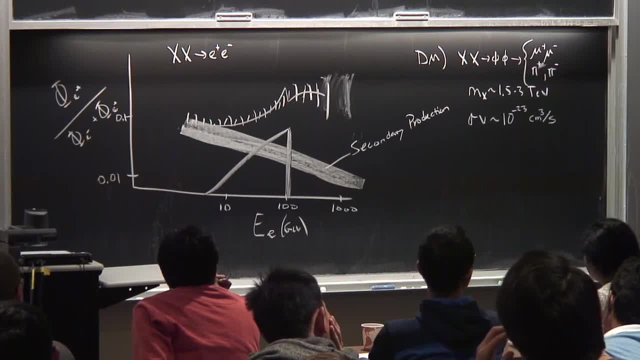 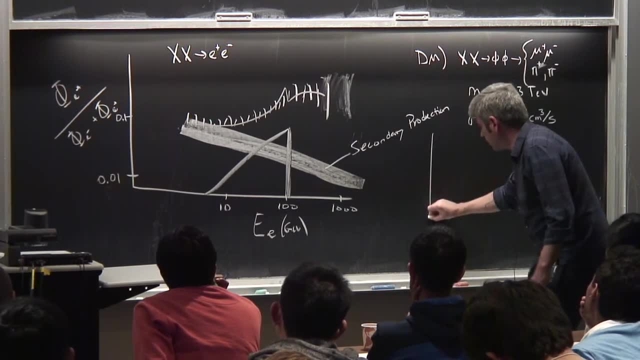 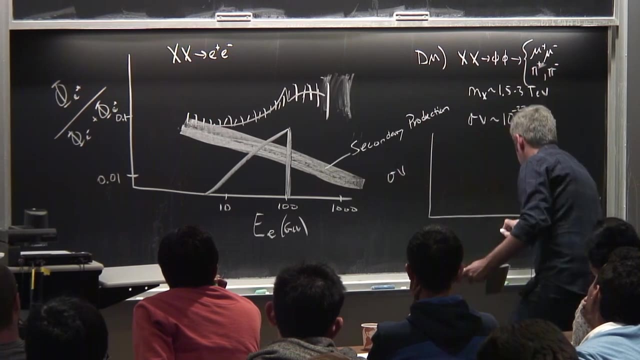 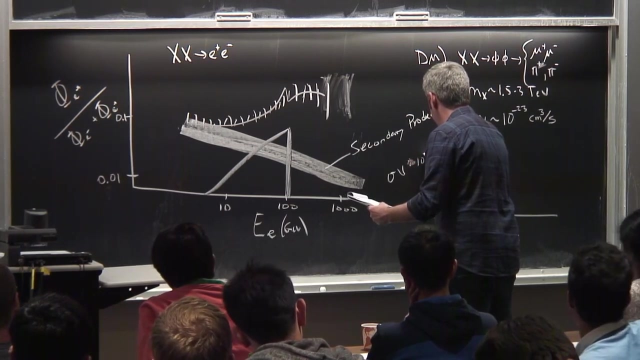 Okay, And you can look for that, even a small one. Okay, It's a distinctive feature that you can look for those sorts of of of departures from a smooth, smoothly varying spectrum And you wind up with constraints that look like this: 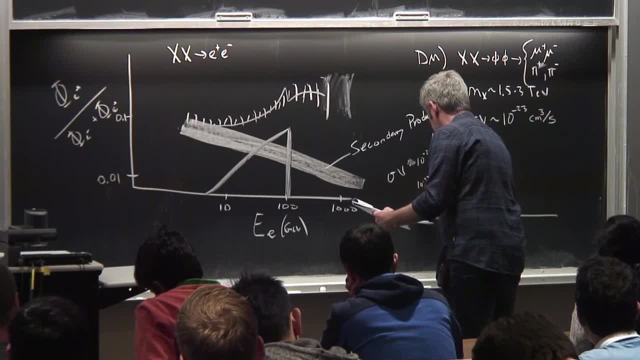 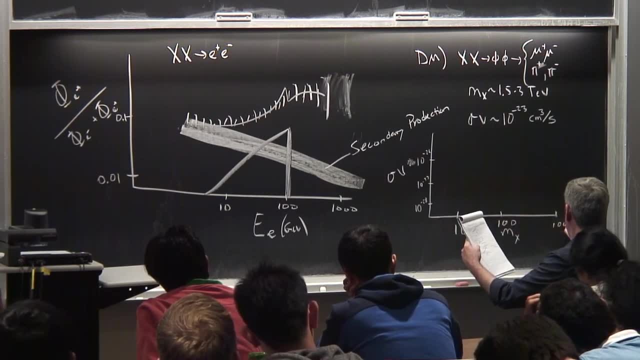 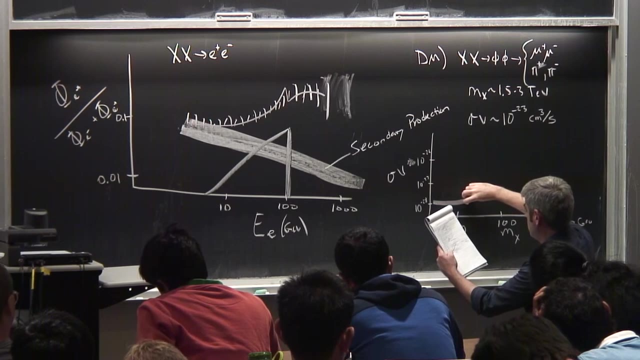 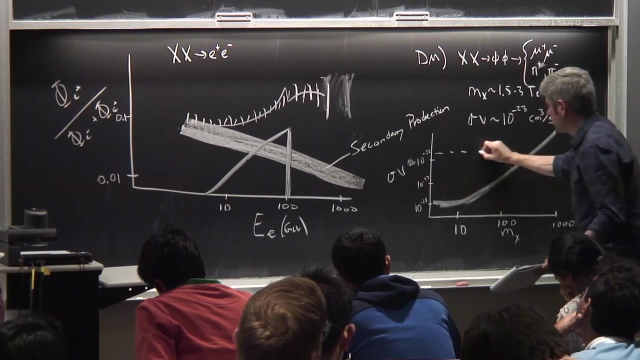 Okay, So for the E plus, E minus case we have a constraint. looks something like that: Okay, So bear in mind, this is the thermal benchmark. So if we have a dark matter candidate that annihilates directly the E plus, E minus all. 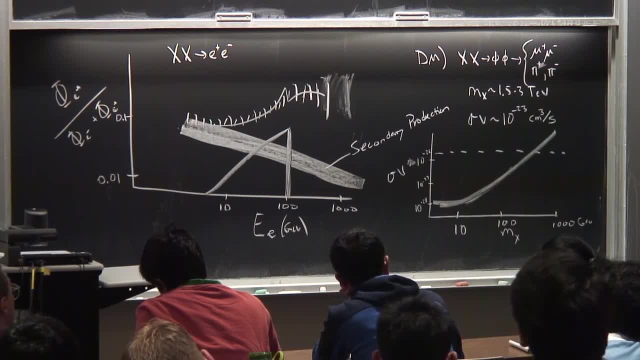 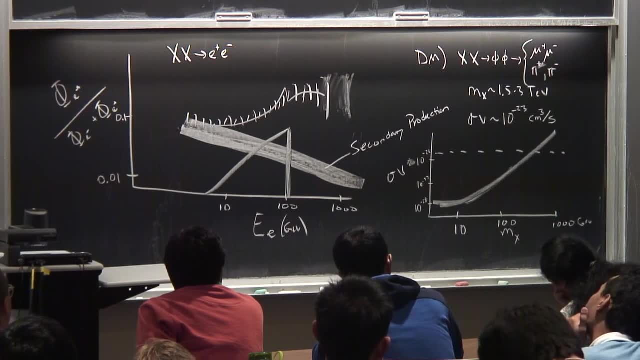 the time and it's a normal thermal WIMP and glossy independent cross section. all that stuff it has to be heavier than a couple hundred GV. So in that very special case this is a very strong one. Okay, So I'm going to label that E plus, E minus. 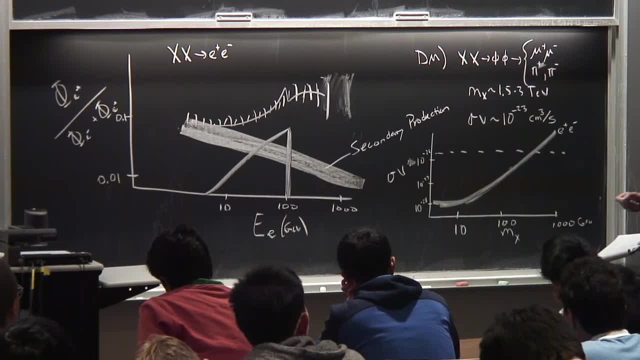 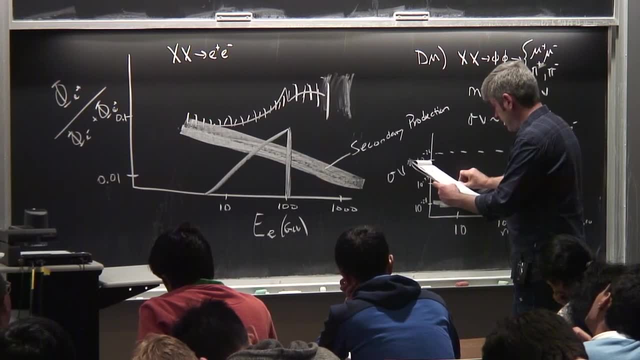 I can do something similar with muons, but it's not as distinctive of a, of a, of a feature. It's kind of a bump that appears over here. It's a little wider, So I get a constraint. in that case, that looks kind of like this and I can do the same thing. 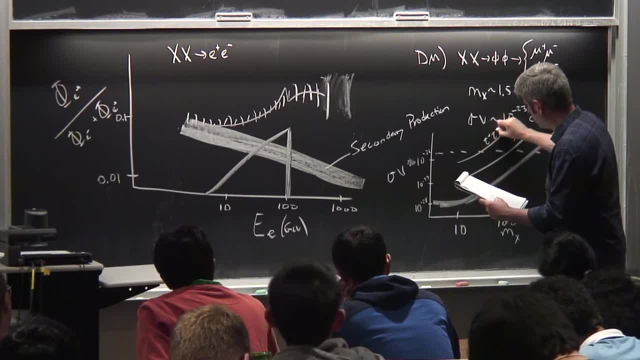 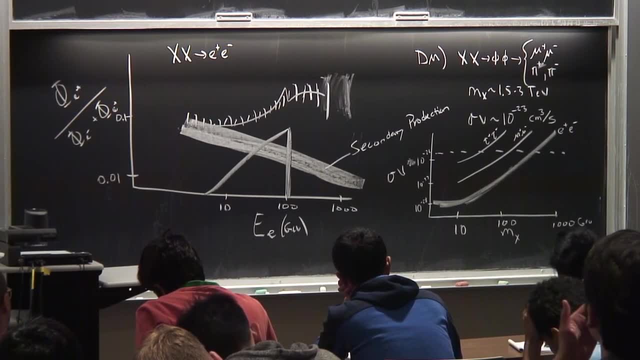 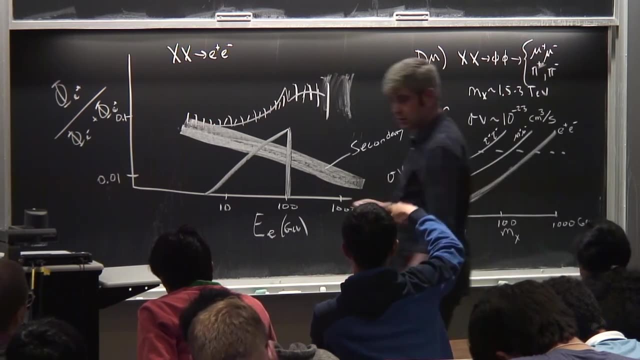 with TAUs and get a constraint that looks like this. So for dark matter, that mostly annihilates. If it annihilates to charge leptons, this is among the most powerful, if not the most powerful, constraint we can offer. Yeah, I have a question about that. 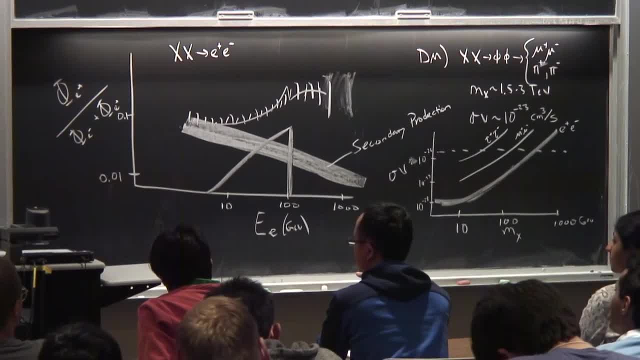 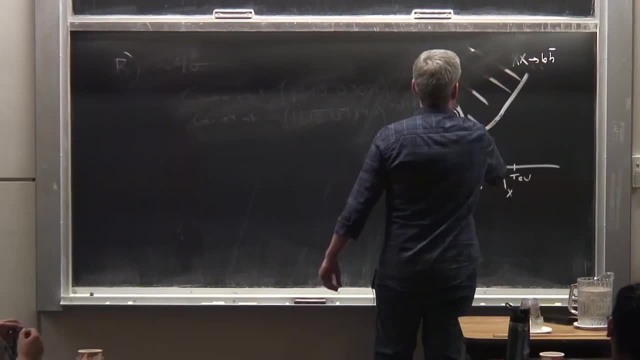 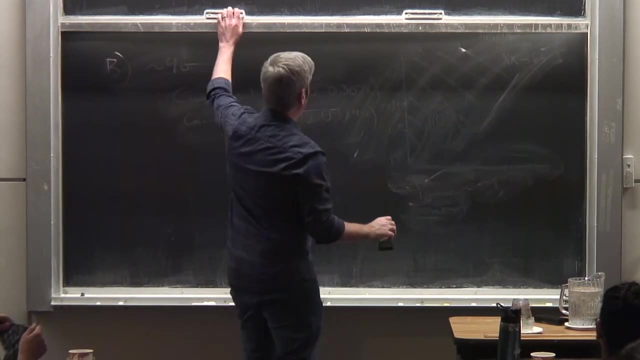 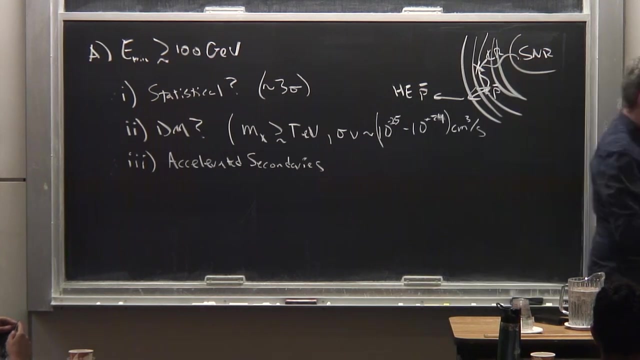 Sure. So are you assuming, other than dark matter, that there's other sources of? So yeah, so I'm saying that we are being entirely agnostic where the bulk of these positrons come from. Okay, My theory is saying that that, whatever make those positrons, they don't cancel out a bump. 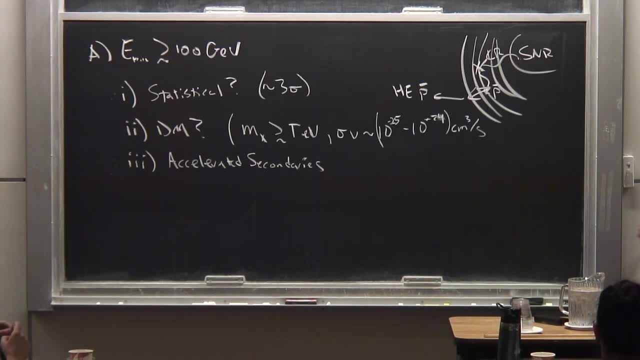 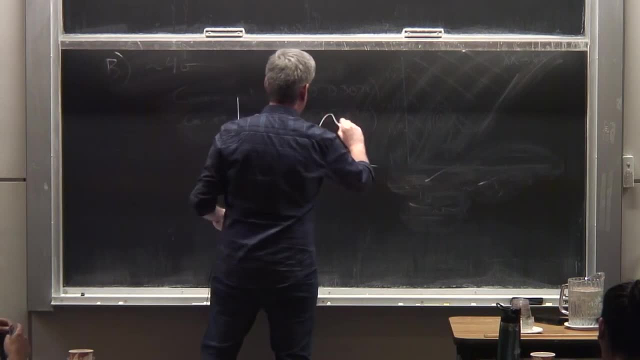 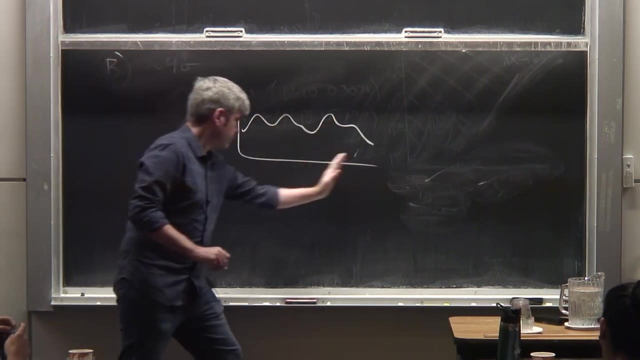 like this. So so let's just say, for the sake of argument, let's say I measure something and it looks like this: Okay, This is some arbitrary thing, and my theory says that at one particular x value there'll be a big spike. 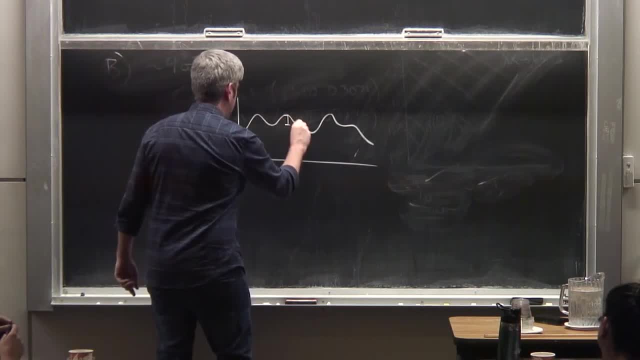 And I say, well, okay, Here There's going to be a spike, that that's. that's that high, but not higher than that, And here there can't be one higher than that, and you know, et cetera. 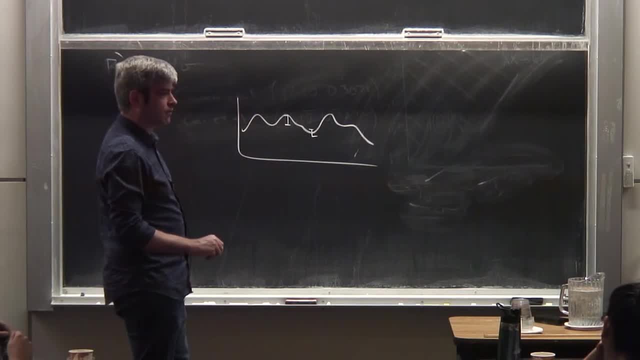 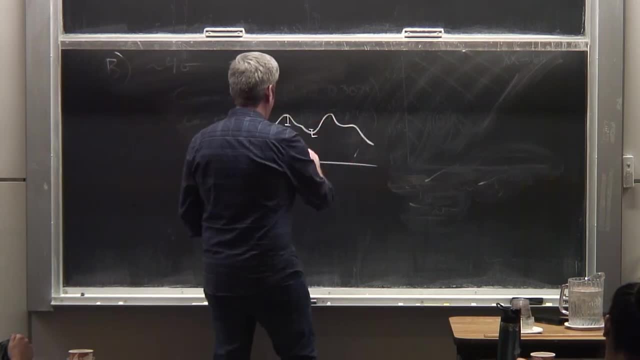 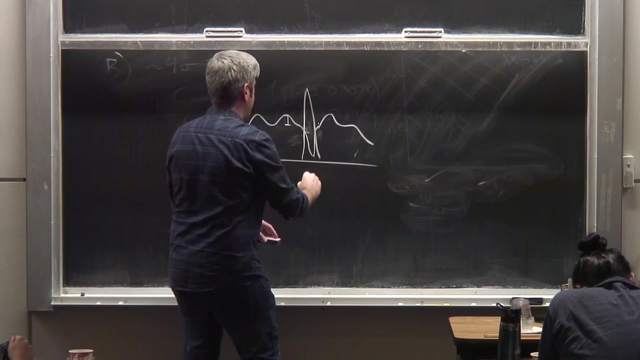 And I can place constraints on there not being a big bumpy thing I'm looking for there, Even if I don't know where that shape comes from. Now, occasionally I could be tricked because maybe the background here happens to look like this and my signal happens to look like this. 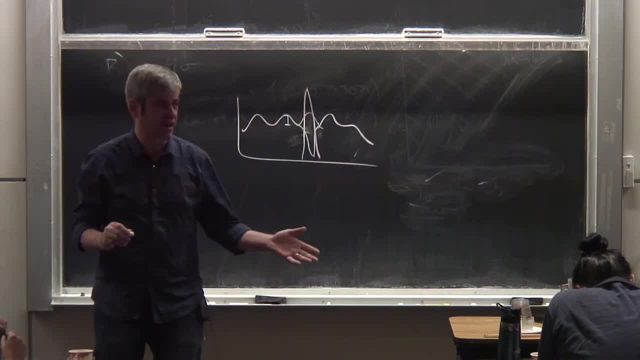 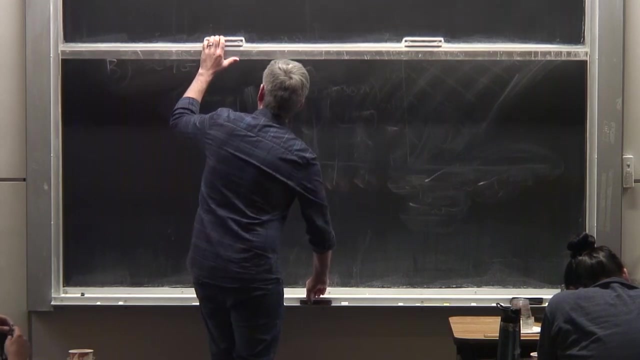 And when I put them together they cancel out in some smooth way. that makes me think there's not a feature there. Statistically very unlikely And there are known statistical tests you can apply to that sort of thing. Okay, So I promised that I would talk about other explanations that don't have to do with dark. 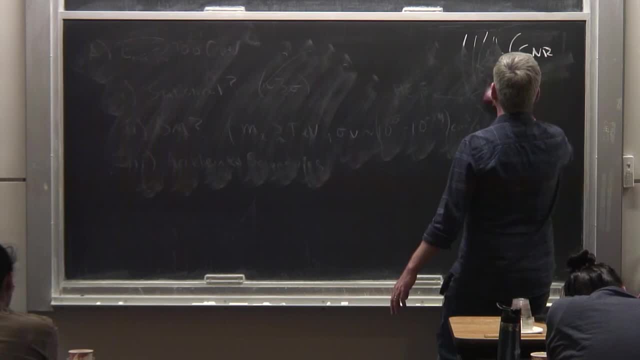 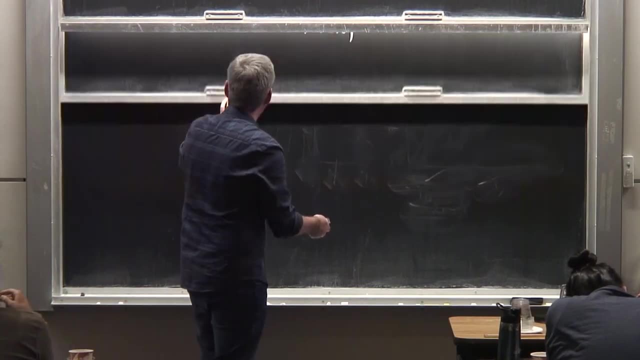 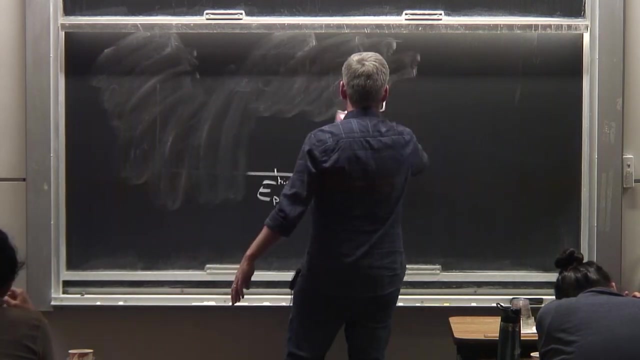 matter In particular. I'm going to tell you why. it's almost certainly the case that the positron excess comes from a handful of very nearby pulsars. Okay, So, So again, I remind you that just the energy loss information tells us that the sort of 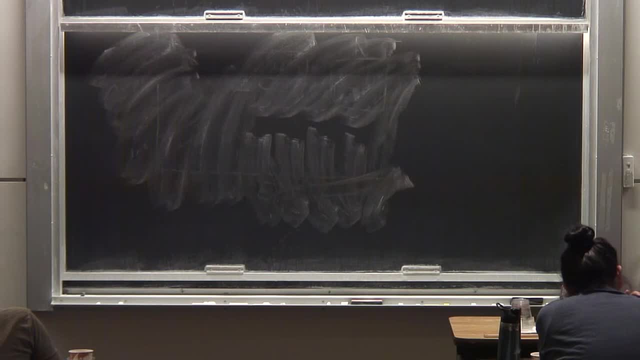 positrons at the high energy of AMS's range that we're looking at have to have been injected within the last few hundred thousand years, And they have to be injected within several hundred parsecs is approximately right. There are not many things that make high energy positrons in that, in that that meet those. criteria. Okay, There are two known pulsars: Gaminga and Monogym. It's weird, but Monogym is a controversial name among certain classes of astronomers. Technically speaking, Monogym is the name of a neutron star and the and the pulsar. 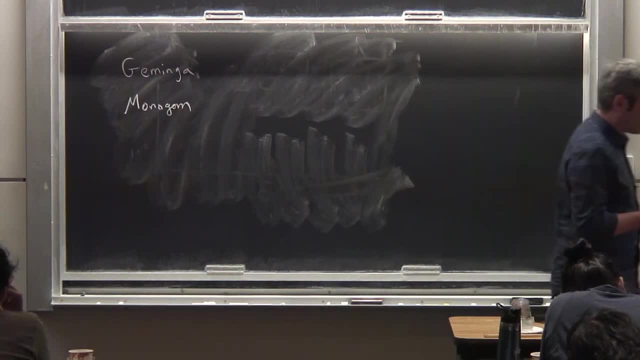 might not have anything to do with that thing. So people argue back and forth. I'm going to call it that. Sometimes they will insist that we call it B0656 plus 14, which they all agree that. that's the thing I'm talking about. 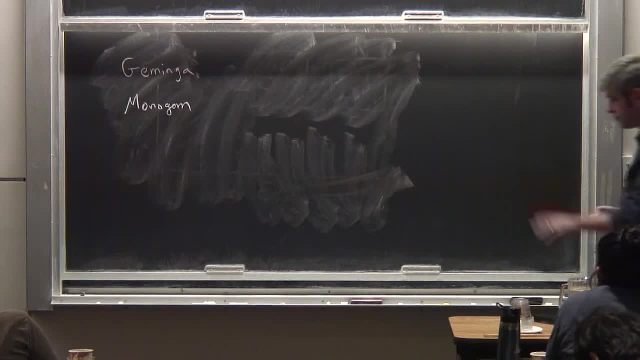 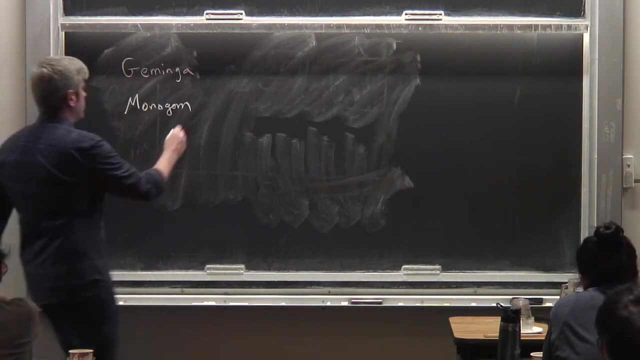 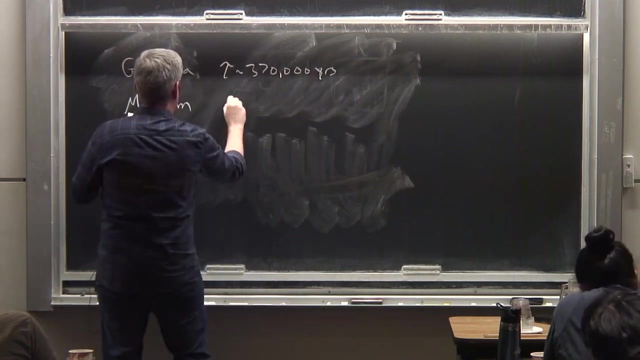 But almost certainly I'm talking about the same thing that they are. So these sources are both young, So Gaminga has a characteristic lifetime of about 370,000 years And Monogym's got about 110,000 years. So they, they, they. we're pretty sure that these things exploded- supernovae. Supernovae at this time scale roughly and have been injected a lot of particles around that time, And their distances are about right too. From parallax measurements we get these sorts of numbers. There are sizable error bars on that, but everyone's in agreement that these are you. 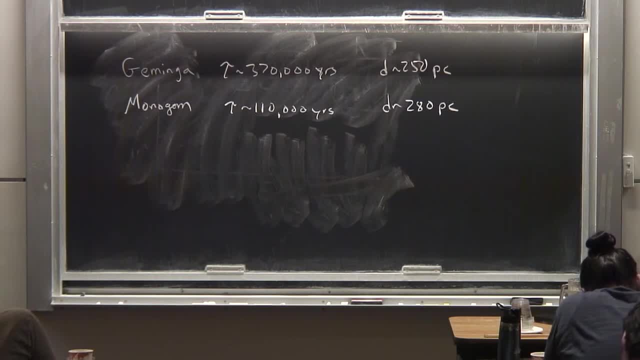 know a few hundred parsecs away, So we've known for a long time. I wrote a paper with Pasquale Blasi and Pasquale Serpico back in 2008., Saying that It could explain the Pamella excess. that's what we had at the time. if these sorts of 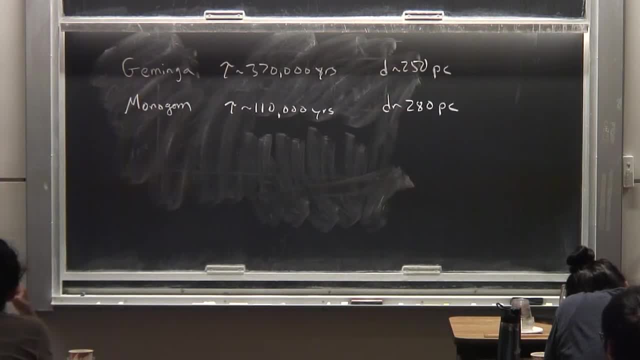 sources inject about 10% of their total energy budget into high energy pairs. That's what you needed. Now, we had no idea if that was true. No one had any idea. if that was true, If you looked at the literature on pulsars and their injection of high energy pairs. 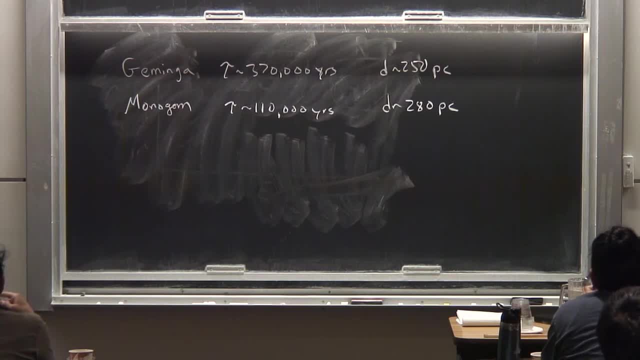 they all agreed it should happen, But some estimates said it could be as high as As high as tens of percents what we wanted, And some said it should be 10 to the minus 4, 10 to the minus 5 of the energy budget. 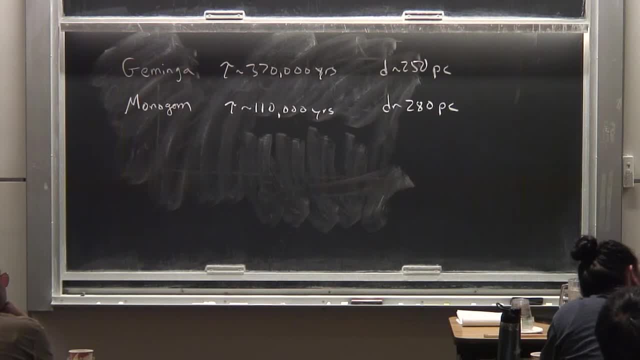 Numbers like this And there was no way of telling. We just did not know enough about how these things functioned to answer that question. So we put it out there as a possibility. I even argued it was a fairly likely possibility in some sort of Occam-Razor sort of argument. 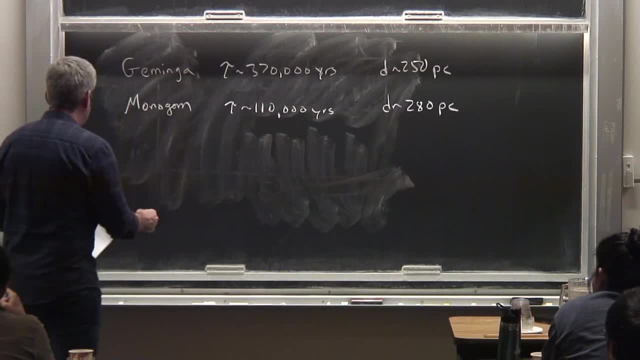 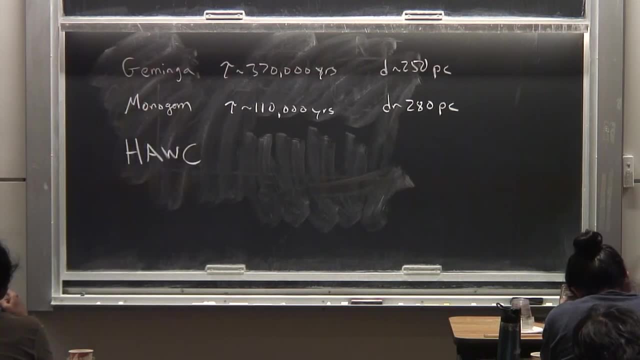 But we didn't know. We didn't know. And then this telescope called HAWC. HAWC came along. HAWC is a ground-based extremely high energy gamma ray telescope, water shrink-off detector, And it measured multi-TEV emission from both of these sources. 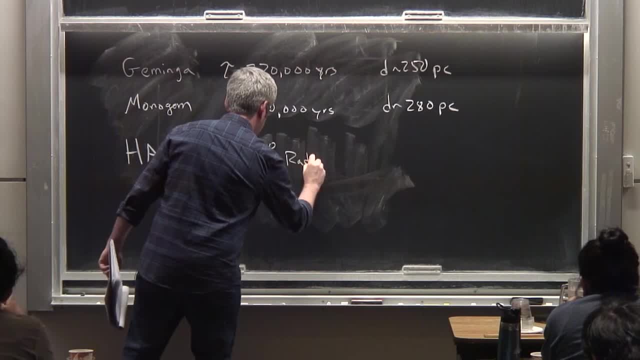 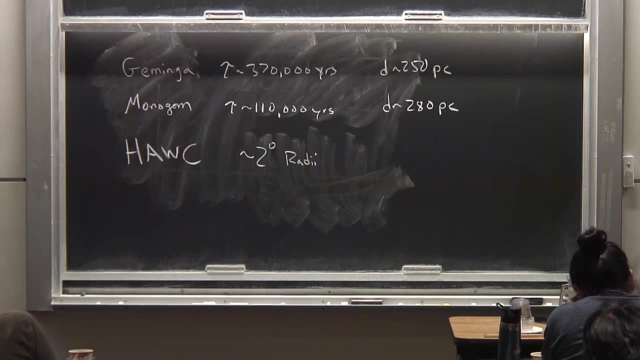 And they found that they both had about 2 degree radii spatial extension of their gamma ray emission. So that's what we did. So this is tens of parsecs we're talking about. So this is not a mission that's coming from the pulsar. 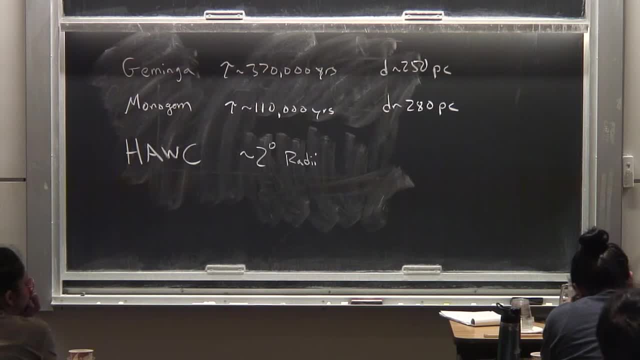 This is a mission from something going on in a tens of parsecs region around the pulsar. What could that possibly be? What's doing the decaying The gamma rays Under low pair production, As it were? So it's not going to decay. 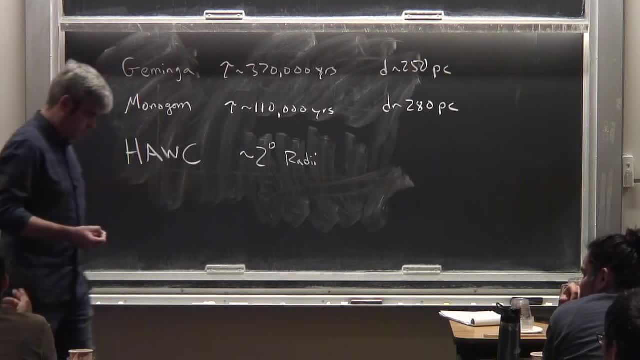 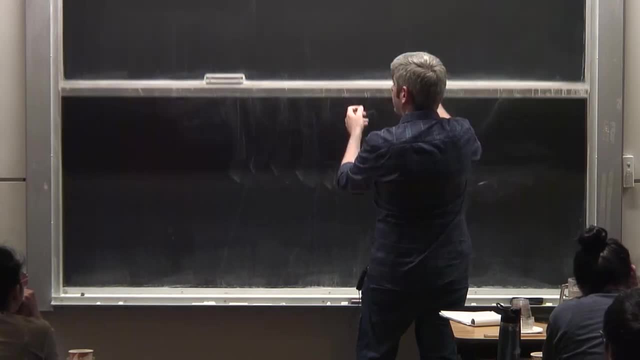 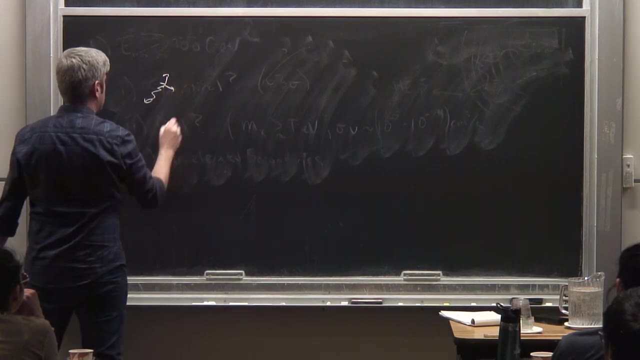 So if you have a gamma ray, it pair produces the angles at which those things go out. Okay, So what you have in mind, if I understand correctly- so I have the pulsar here- A gamma ray comes out, It pair produces. 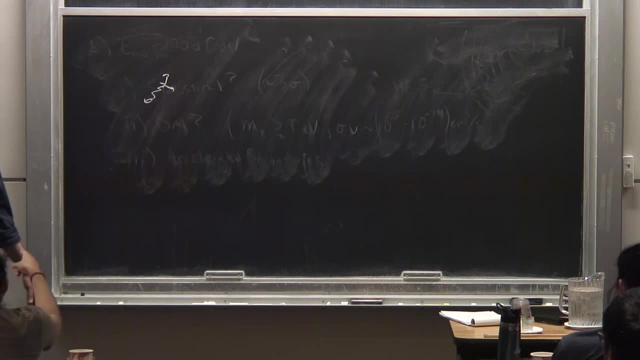 And then how do you make the new gamma ray? It annihilates another one, It goes nearby, Okay. So then, well, okay, but they don't do that Right. High energy: When you pair produce in high energy, They don't. 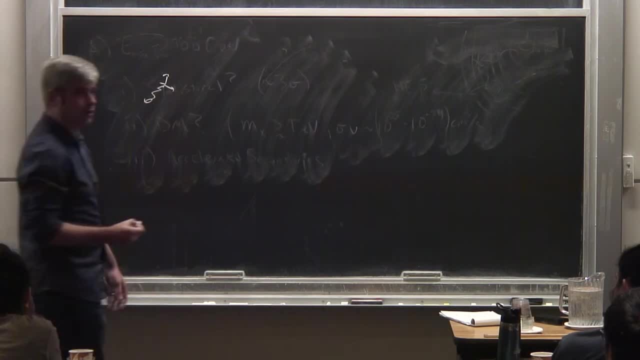 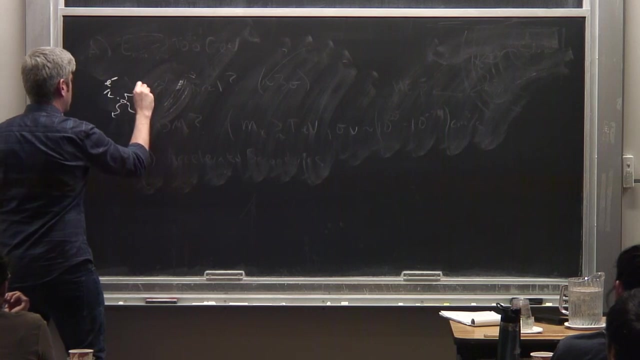 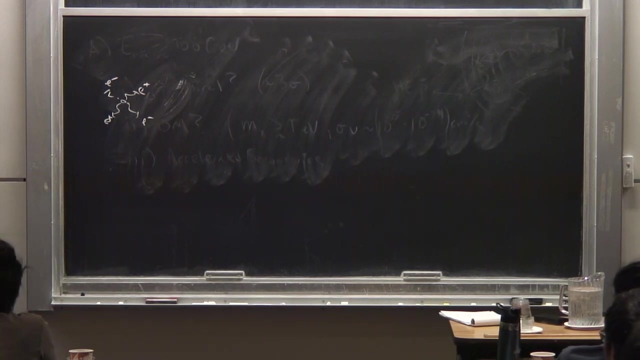 They don't annihilate. But you're close, Real close, So I'm going to do the first step. The first step is right. So I have electrons and positrons coming out in all directions. They fill a volume around the pulsar. 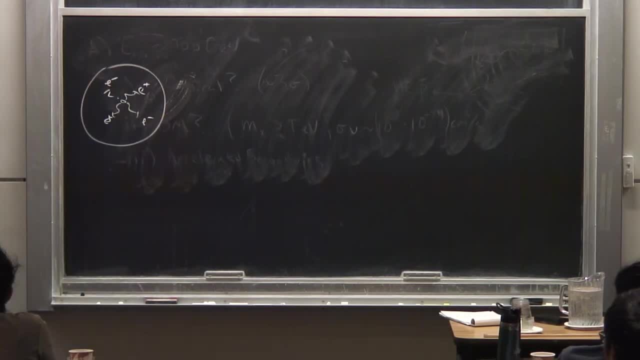 Tens of parsecs in extent. And then how do those electrons and positrons make photons, Something that's come up in these lectures a few times? Electrons scattering off gas, don't? I mean they can make brems, but that's, there's not. enough gas. Synchrotron radiation makes you really really low energy stuff. It doesn't make gamma rays. No, I'm not going for anything like that, Just inverse Compton scattering, All right. So you, You take the starlight. 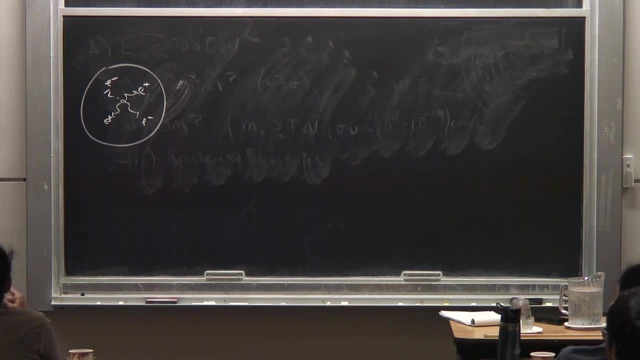 You take those electrons, You bombard the starlight, You make gamma rays, And now you've got this whole region that's bright in multi-TV gamma rays. So I literally think this is the only explanation for this data that makes any sense. It's weirdly controversial, but it shouldn't be. 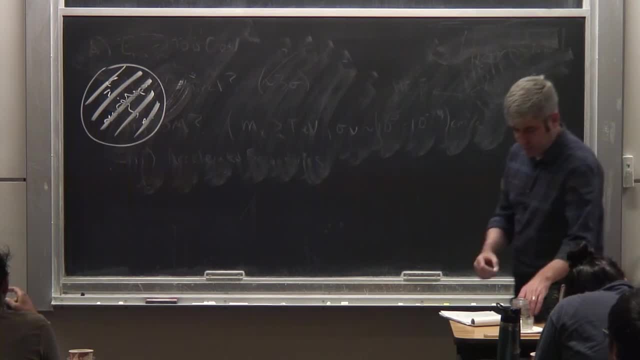 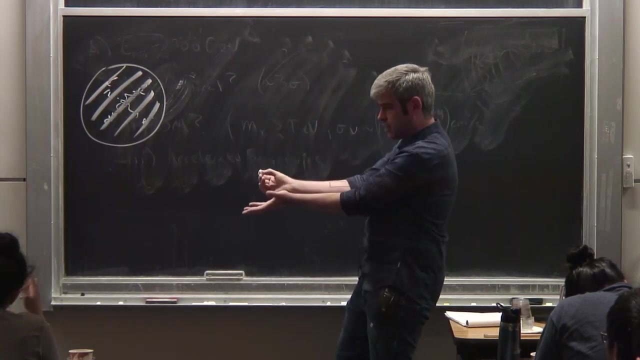 This will be the answer. when all the dust settles, I will. I will bet my car on that. Okay, Now I've got a nice car, All right. So here's where this is interesting for us, right? So now we have measured the gamma ray emission from this multi-tens of parsec region. 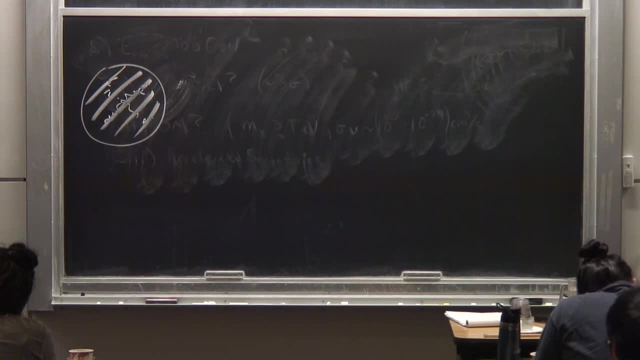 We essentially know that that gamma ray emission is coming from the very high energy electrons and positrons that are being injected. So now the flux that we see in these gamma rays is a direct measurement of the flux being put out in electrons and positrons. 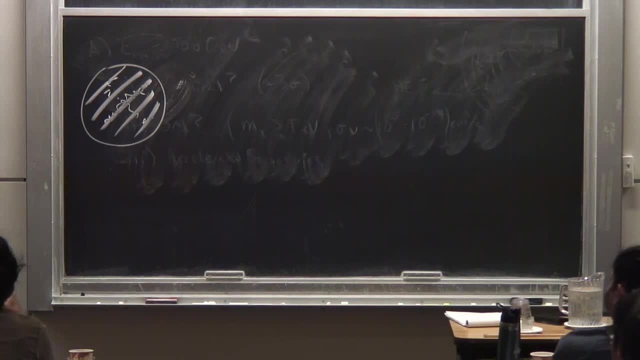 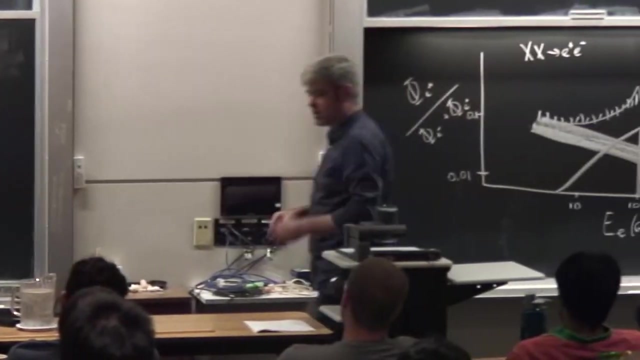 Okay, And lo and behold, it's about 10% of the energy budget of these pulsars. So Hawke has provided us with a way, with a factor or two error bar. That's about right. Hawke has told us that 10% of these objects' energy go into pairs. 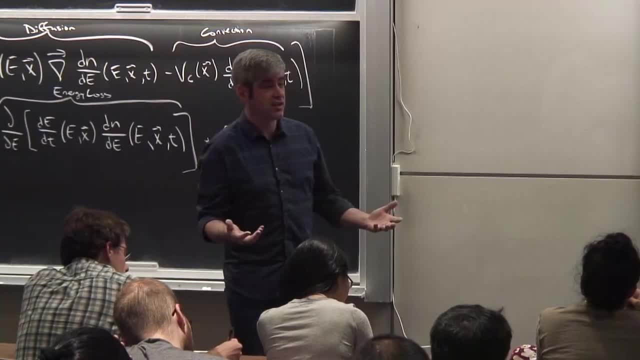 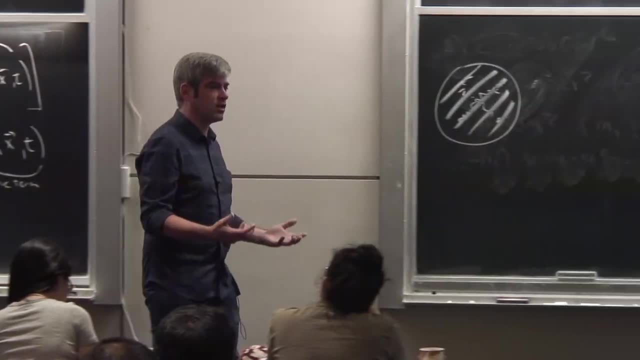 And we said back in 2008 that if about 10% of the energy of nearby pulsars went into pairs. So now we can explain this positron excess And in my view, this tells us that almost certainly what we're seeing here is being 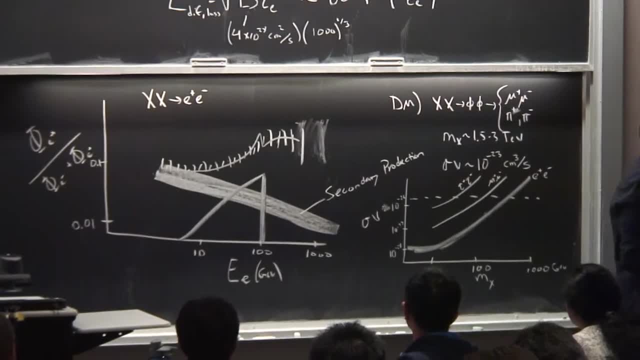 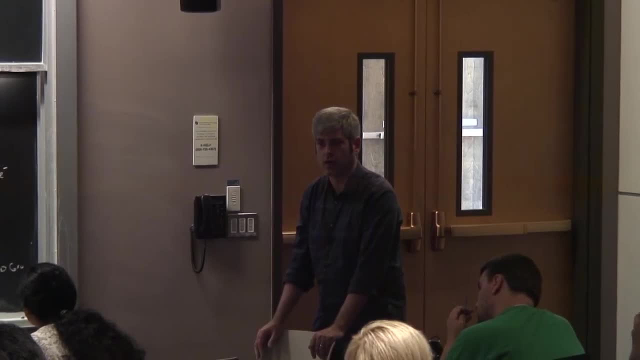 dictated by Gominga MonoGem and you know it could be a couple other pulsars. in an local neighborhood And at low energies there'll be a lot of pulsars because those have lower energy losses and therefore can extend out to greater radii.